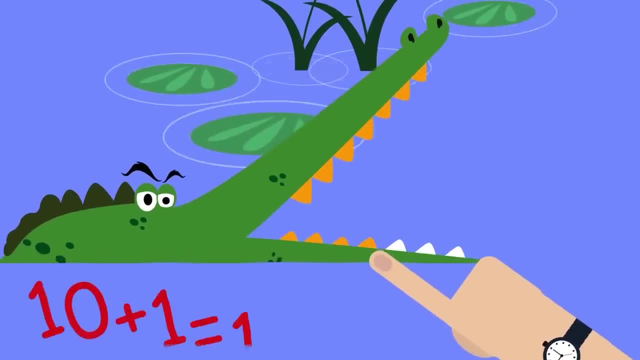 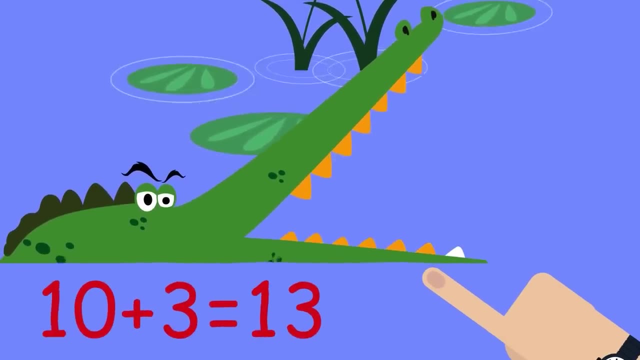 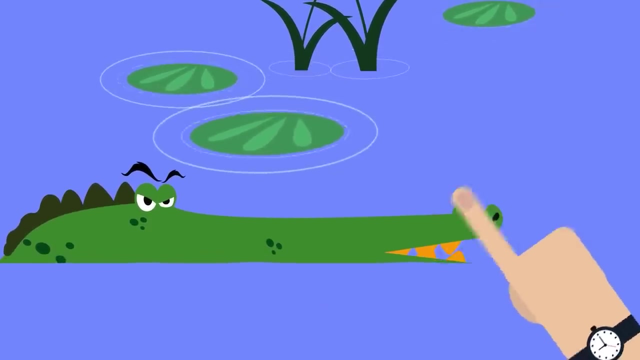 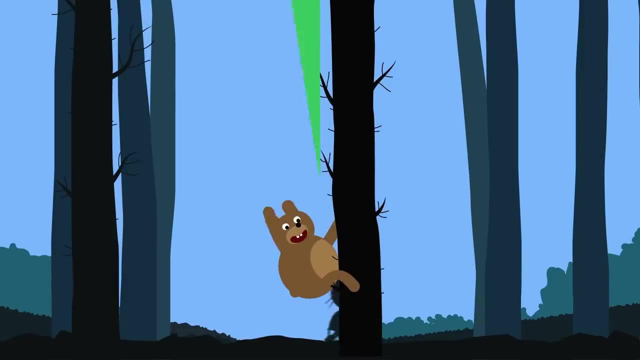 four, eleven, twelve, thirteen, fourteen. Ooh Crocky, you really are extremely mean. Ooh, What are you up to, Mr Bear, Climbing all the way up there? Aha, you're after something. 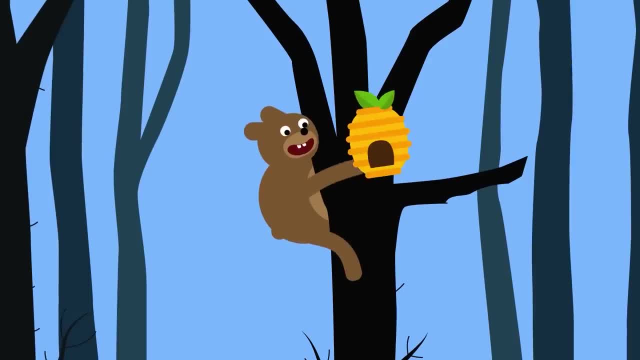 sweet, A sticky runny honey treat. Uh-oh, here comes one angry bee With two more friends, That's… one, two, three… four, five, six, seven, eight, nine, ten. Ooh, Crocky you really. are extremely mean. Well, let's be sure, We'll only count your perfect smile and count your teeth. Ooh, We'll only count your perfect smile and count your teeth. Ooh, Crocky, you really are extremely mean. We'll only count your perfect smile and count your teeth. Ooh Crocky, you really. 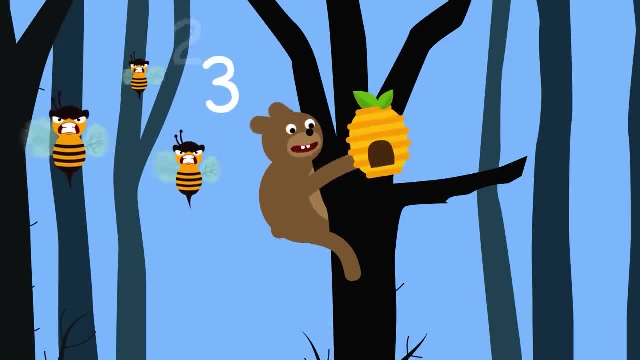 One, two, three, Another two just left the hive. Watch out, dear bear, because now there's one, two, three, four, five. You must stop now, before you're stung Too late. Ouch, That must have hurt your bum. 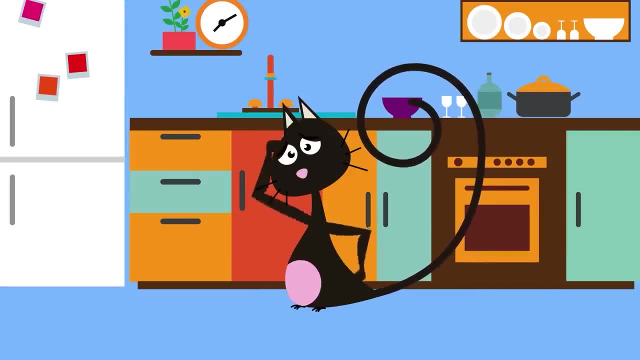 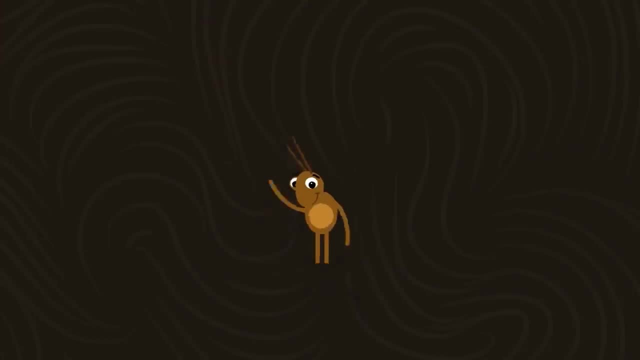 Hello there, Mr Scratchy Cat. Does it really itch as much as that It does you say, Well, let us see. Ah, no wonder, Cat, You've got a flea. Did you see it move just then? I'm sure it's going to hop again. 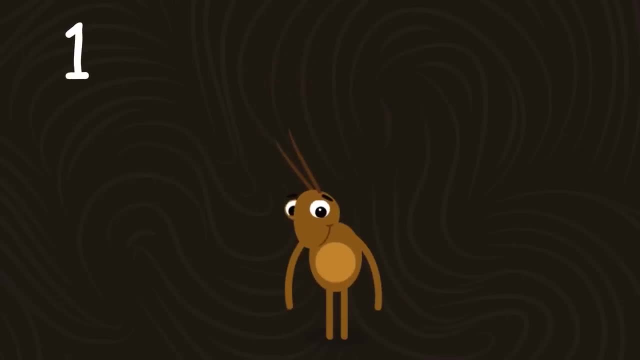 There it goes: One, two and three. How many hops do you think there'll be? Four, five, six, seven, eight, nine, ten? Oh look, It's going to hop again. There's only one thing left to do. 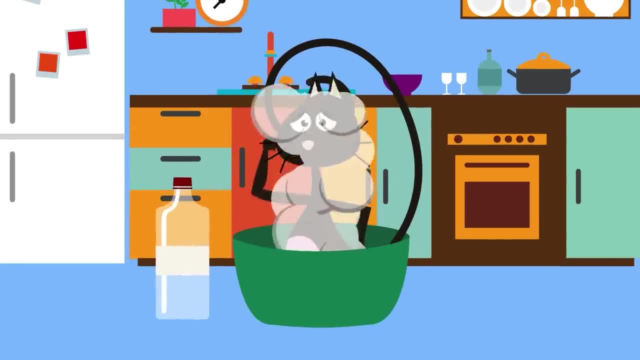 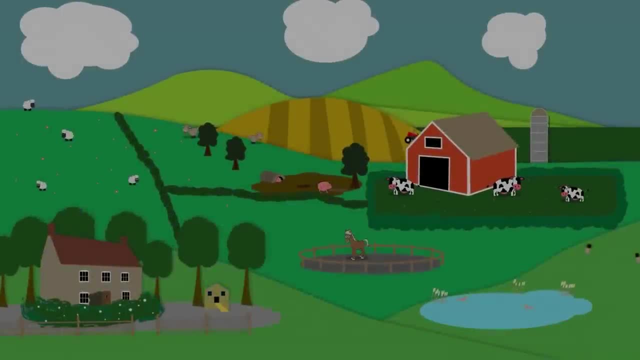 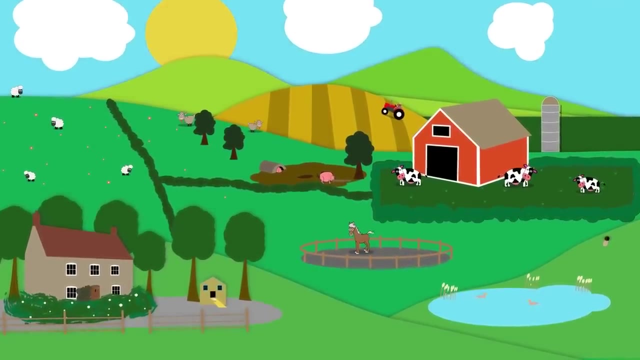 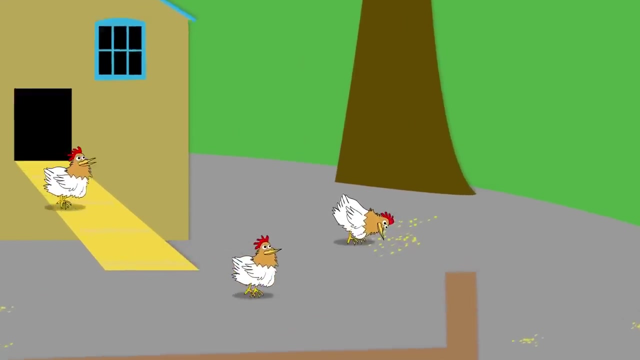 Wash it out with flea shampoo. Welcome to Number Farm. Shall we wake up the animals? Wakey, wakey animals. Definitely wear you a whichever coat you want. No Bill, You can't keep you from scurrying around in there, dominated by the flea. 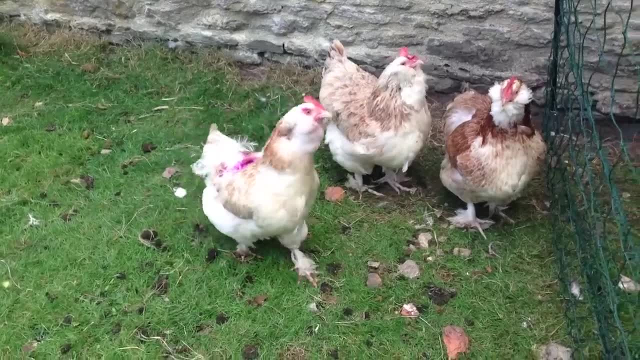 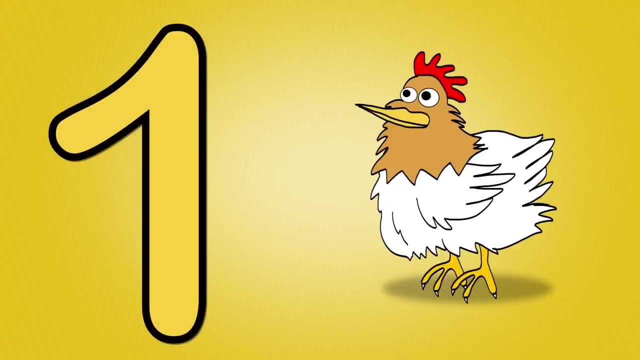 Look at how covered it is. it hurts. These kids have lost their jobs. Oh's sure they will. But you need to get driving and back out of here And get in your car and put your tailaxes on. Come on, Bill, come on. 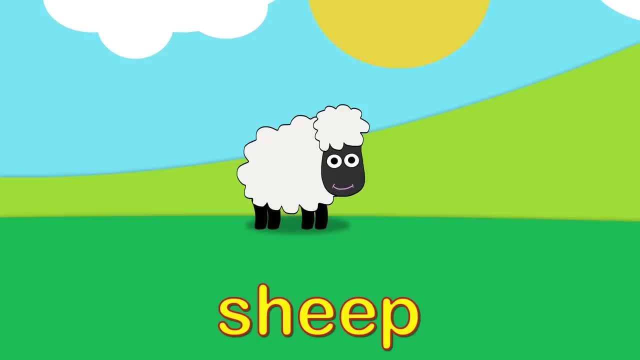 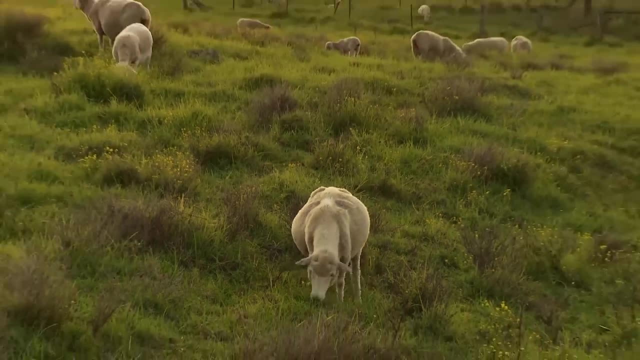 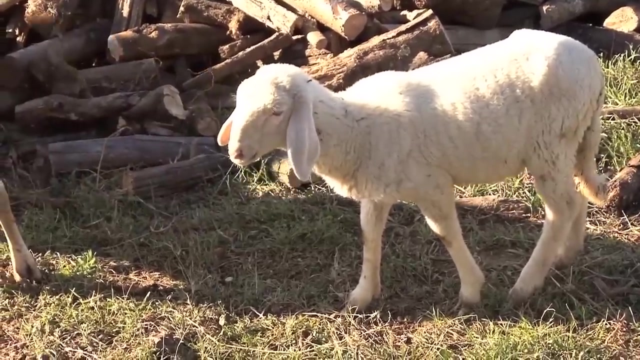 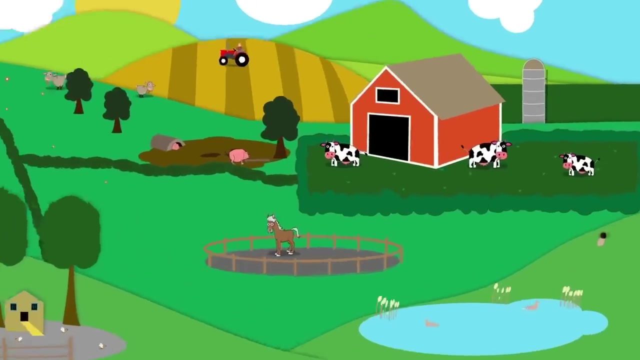 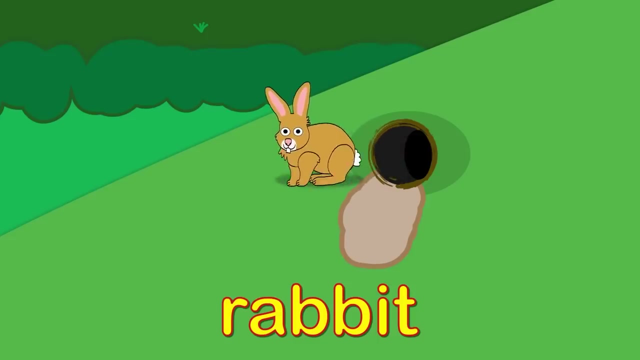 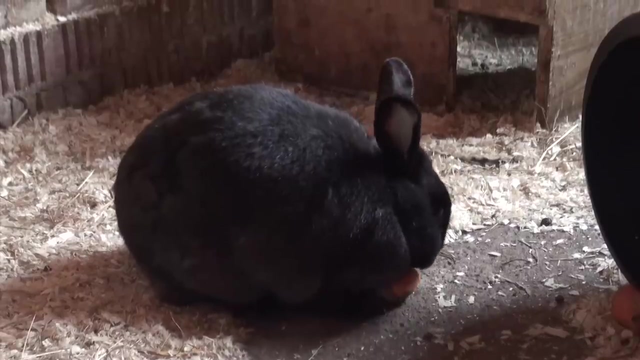 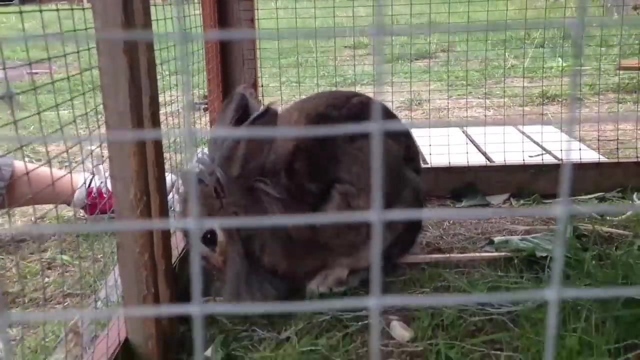 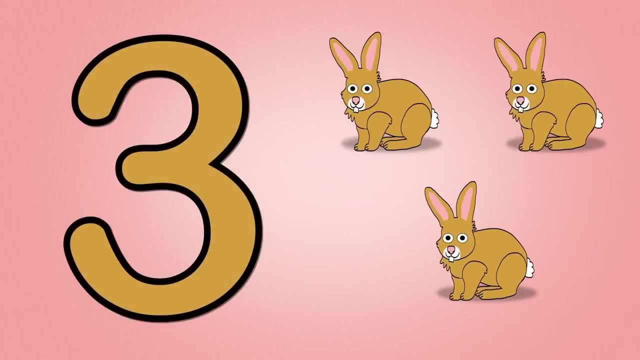 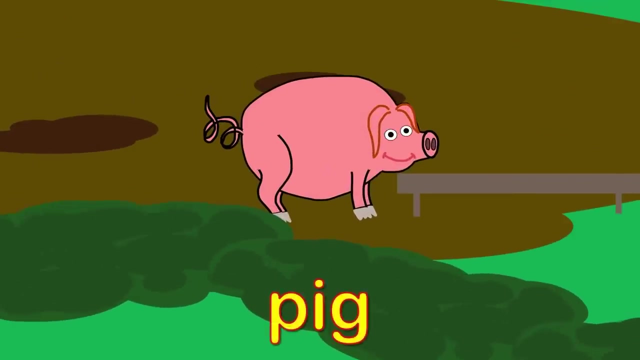 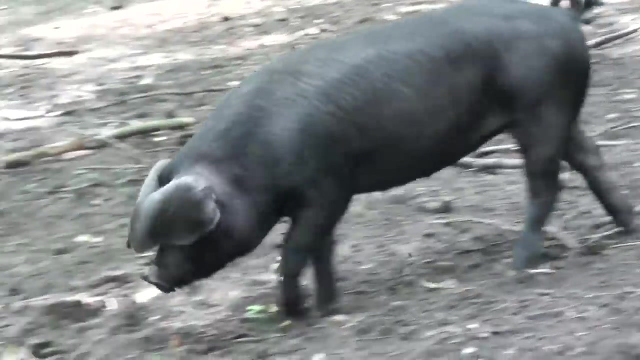 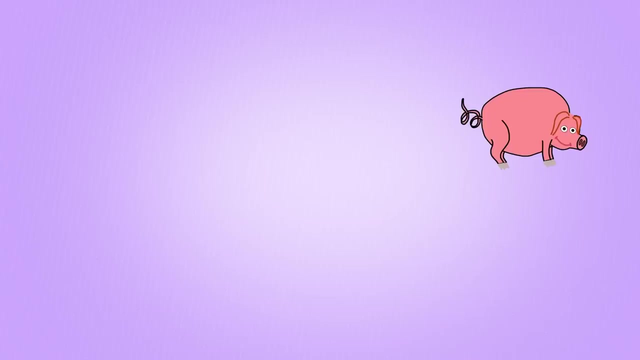 I'll get the car, but here we go and wash these dogs. Wait, Here comes the 식y: One, two, two sheep. Hello hopping rabbit. One, two, three, Three rabbits. Hello pink pig. One, two, three, four, Four pigs. 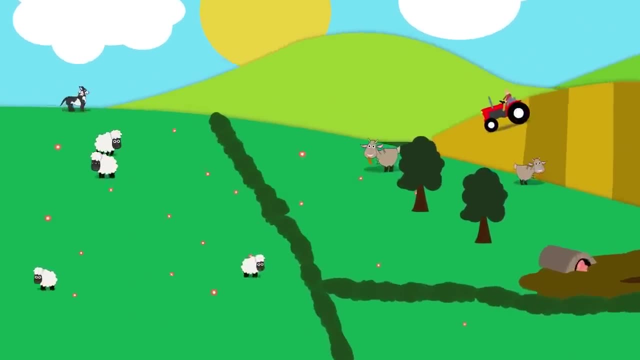 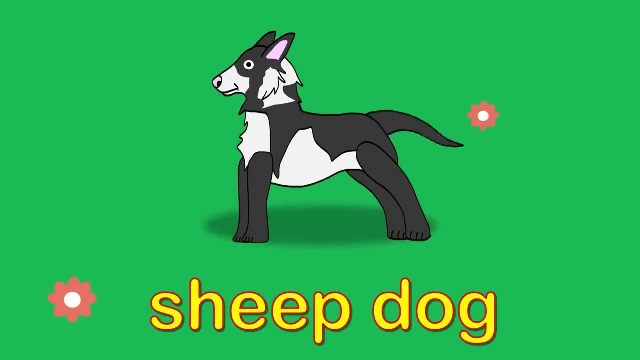 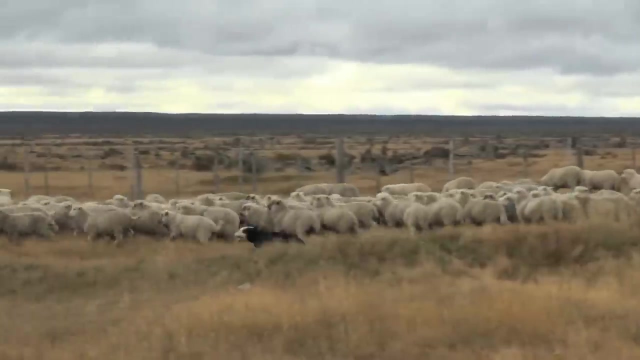 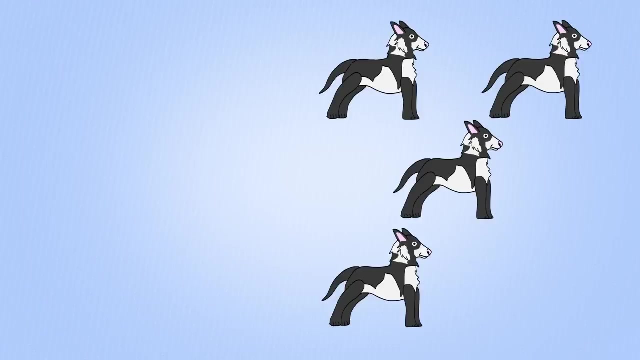 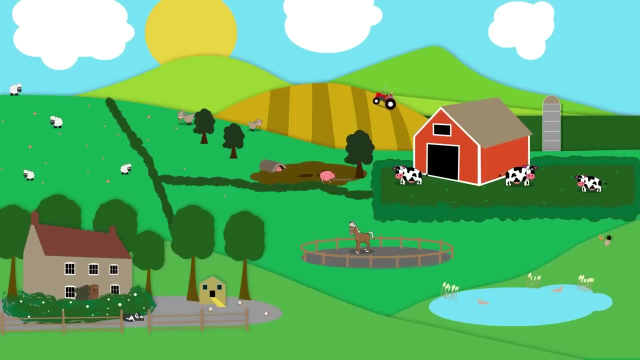 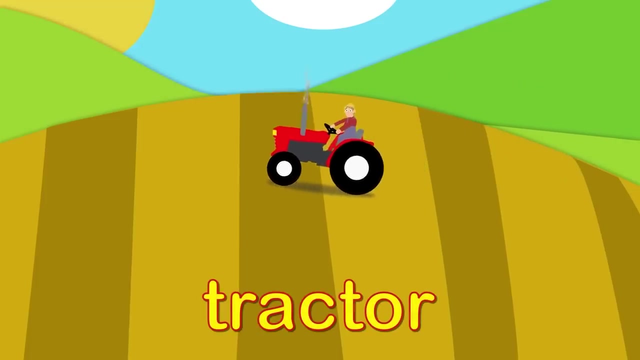 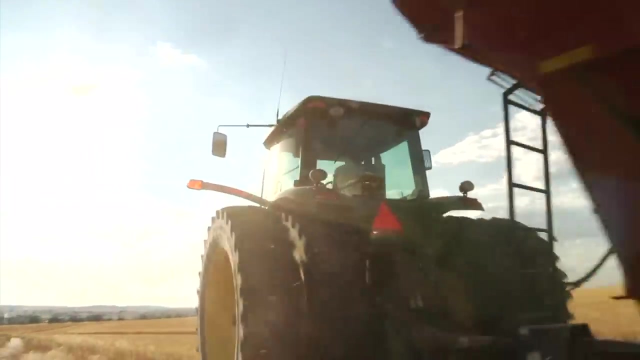 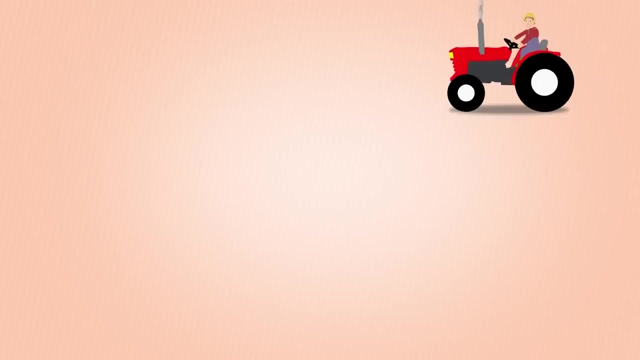 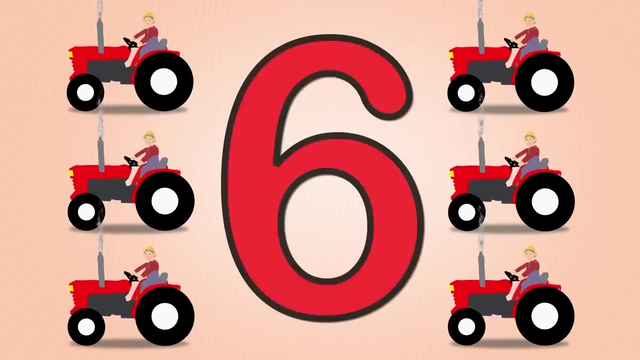 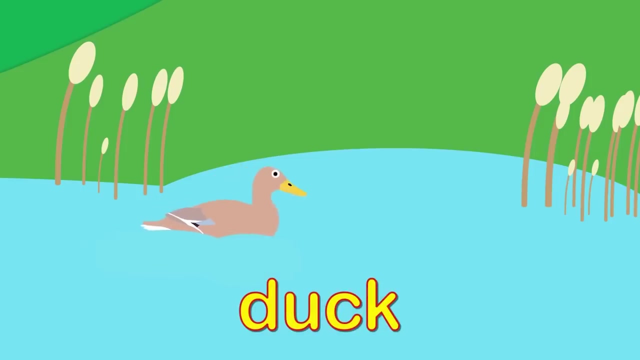 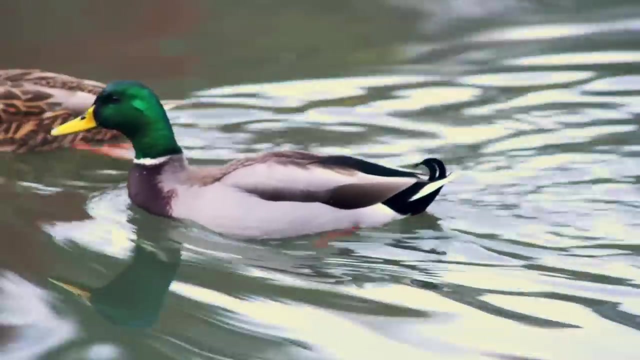 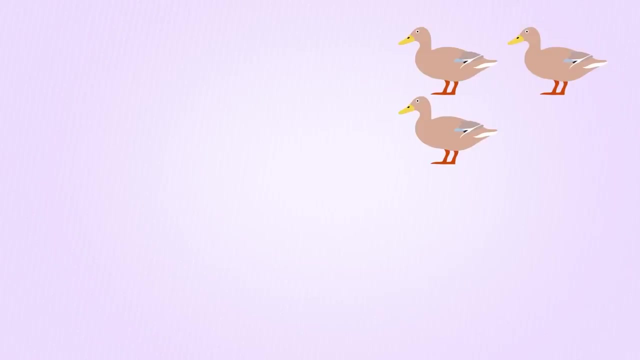 One, two, three, four, Five sheep. Hello there clever sheepdog. One, two, three, four, five, Five sheepdogs, Three sheepdog. Hello red tractor. One, two, three, four, five, six, Six tractors. Hello quacking duck. One, two, three, four, five, six, seven. 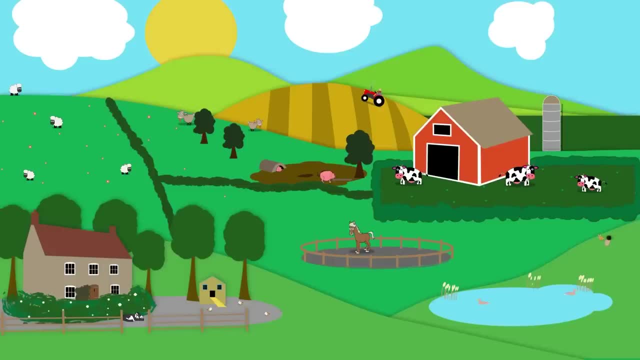 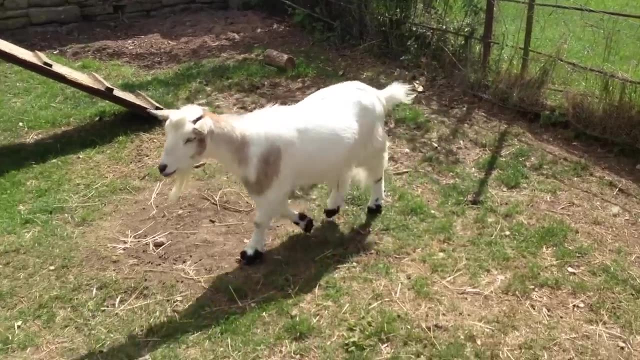 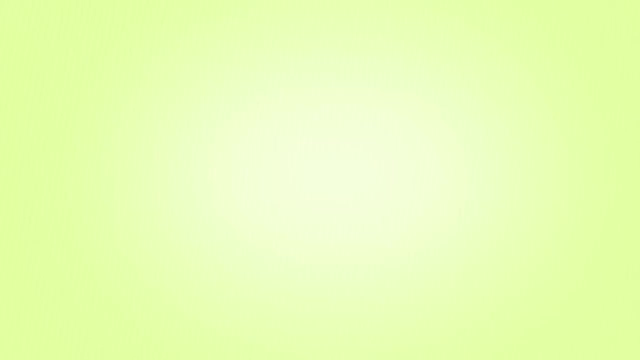 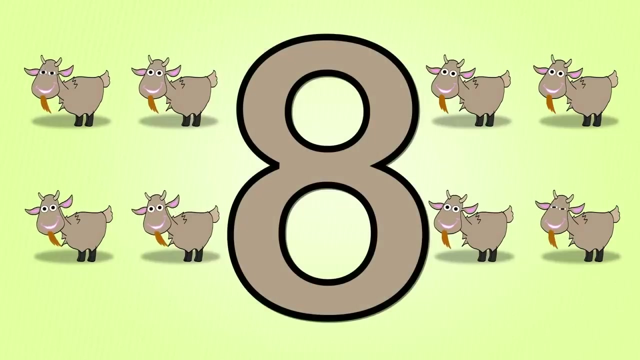 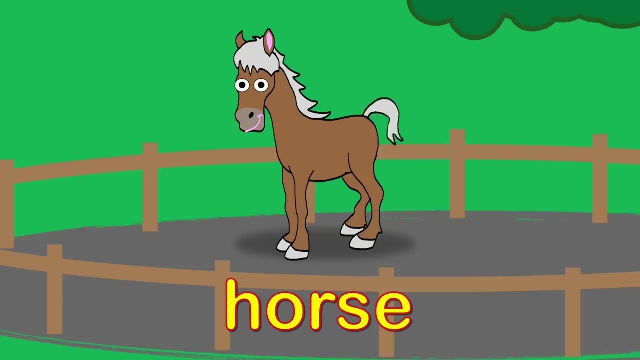 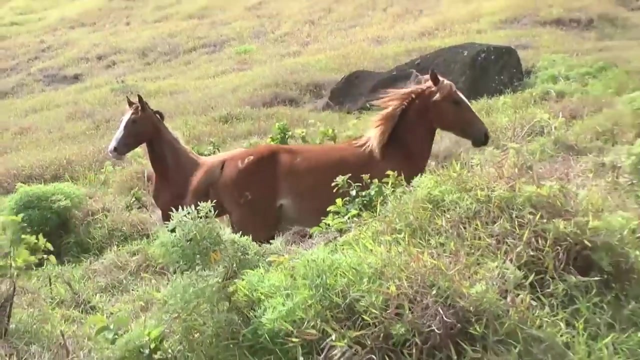 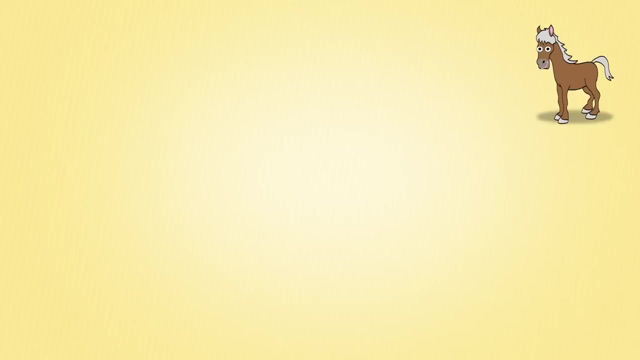 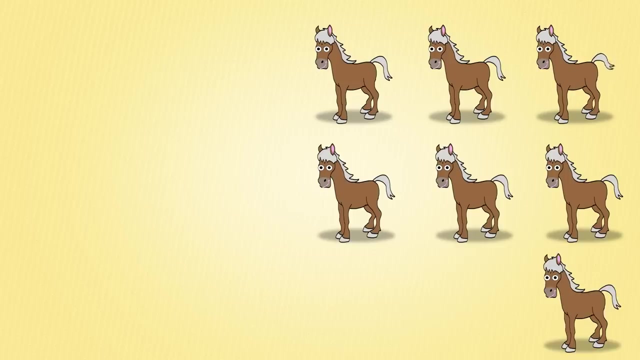 Seven ducks, Six tractors: One, two, three, four, five, six, Eight goats. Hello smiley Goat. One, two, three, four, five, six, seven, eight, Eight goats. Hello lovely brown horse. One, two, three, four, five, six, seven, eight, nine. 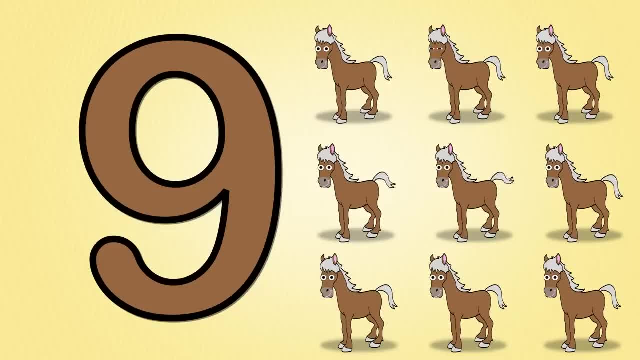 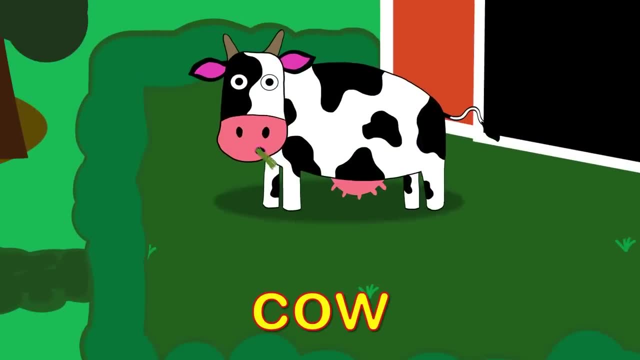 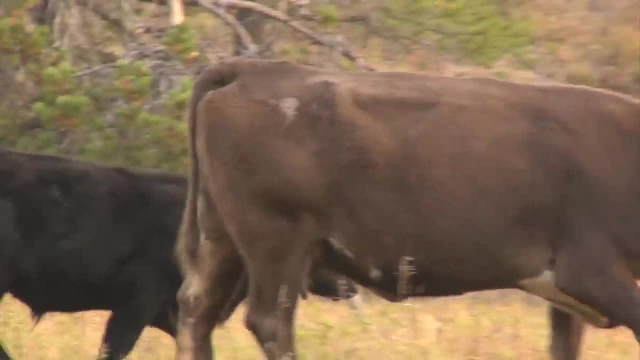 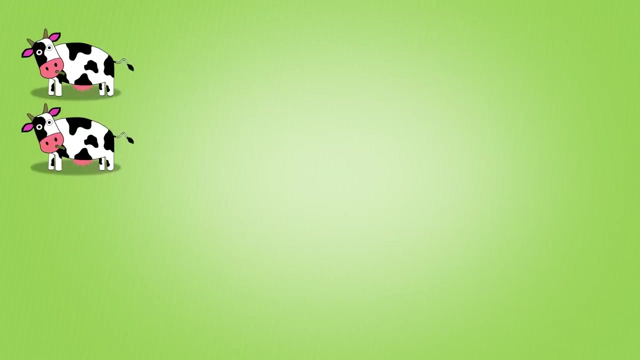 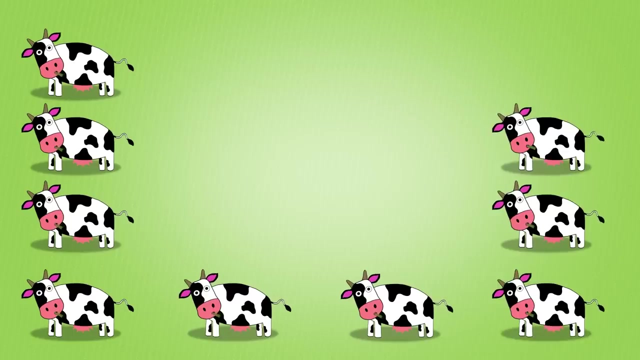 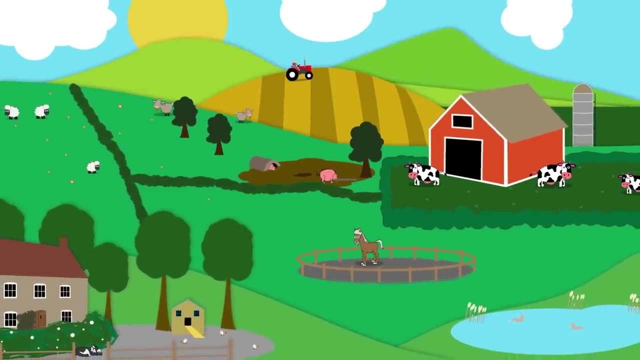 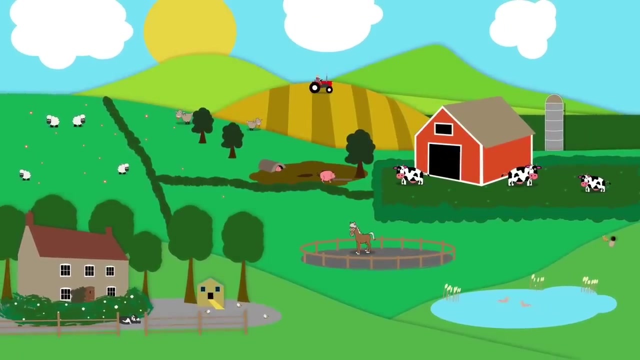 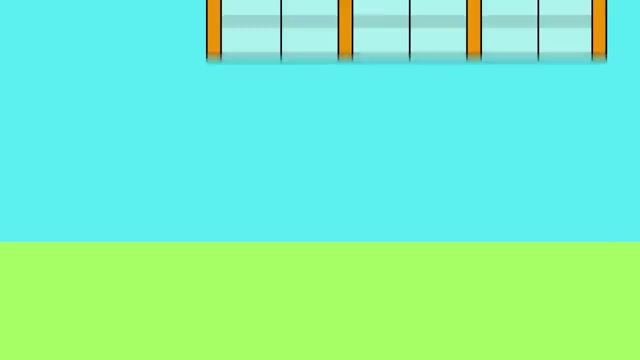 Nine horses. Hello, moo moo cow. One, two, three, four, five, six, seven, eight, nine, Ten, Ten cows. Thank you for visiting Numberpharm. Have a good day. See you again soon. Let's build a plane Airport. 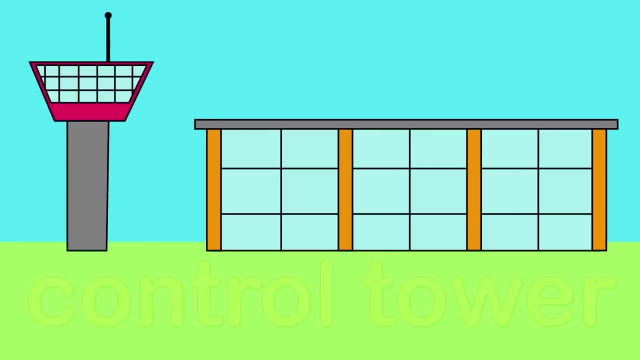 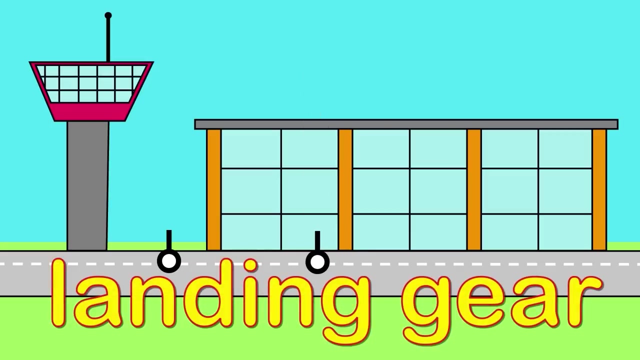 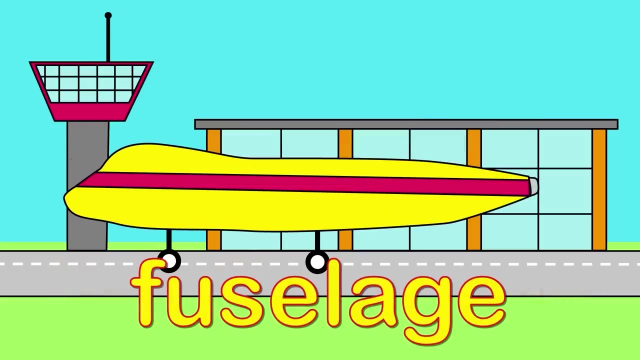 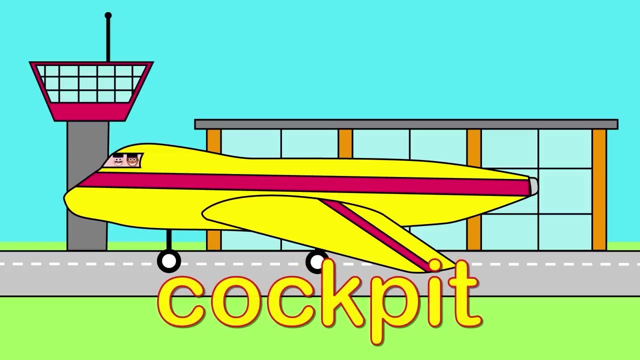 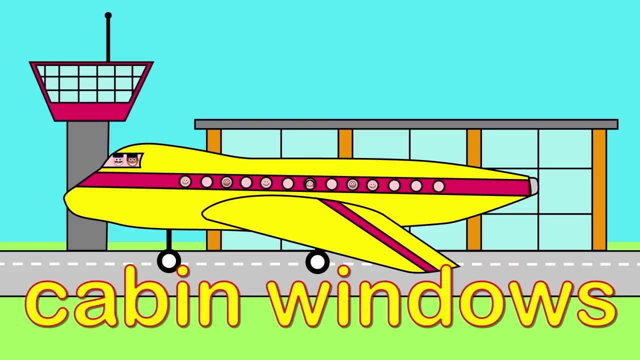 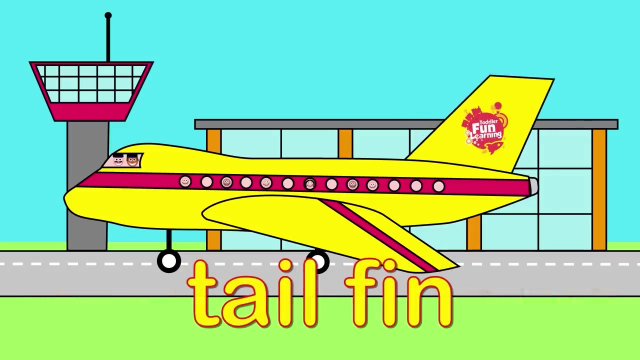 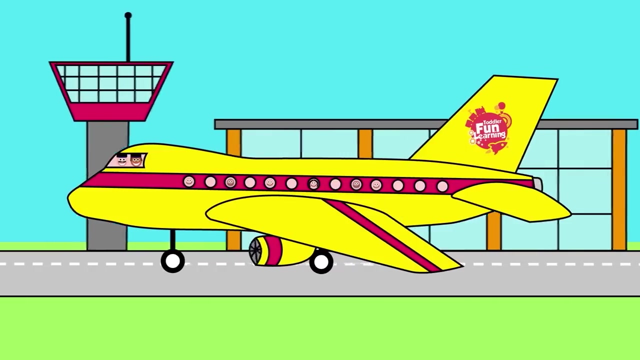 Let's build a plane. Let's build a plane: Airport Control tower, Runway, Landing gear, Fuselage Airplane Airplane Airplane Warhead. Airplane Sink. Wind Spinning ан Thin Tail, Thin innovation, advertising Joint validate Google ü Jet engine Rear wing. Let's take off. 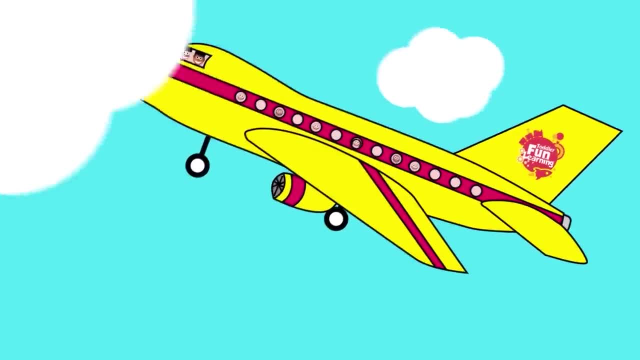 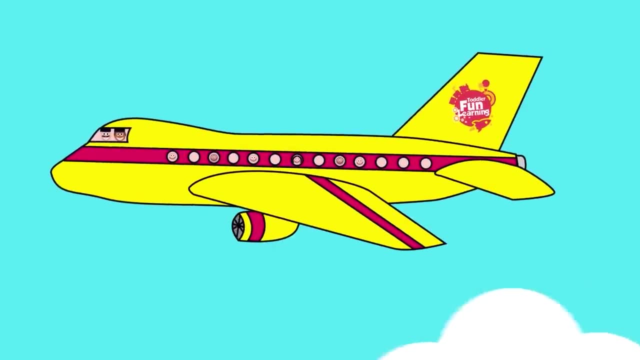 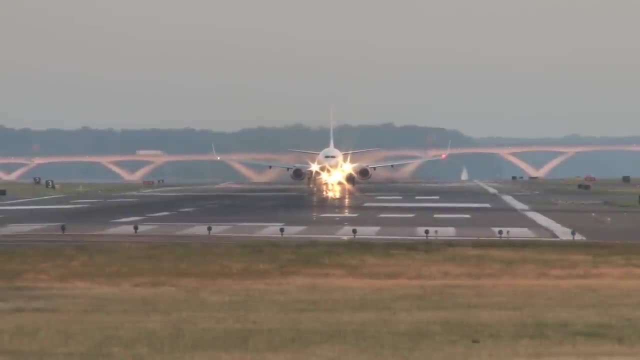 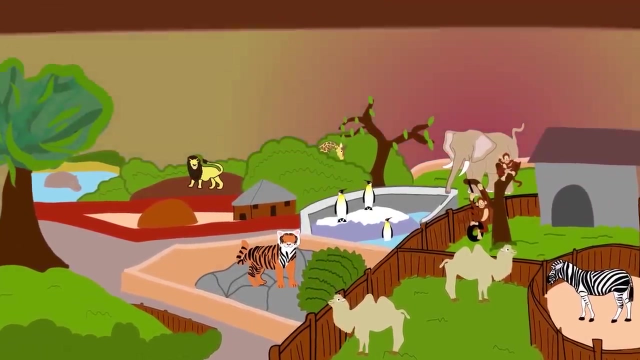 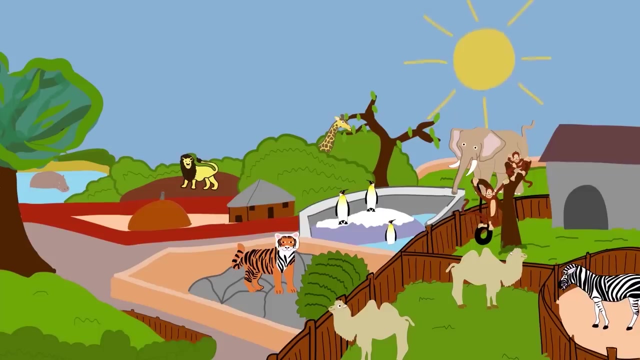 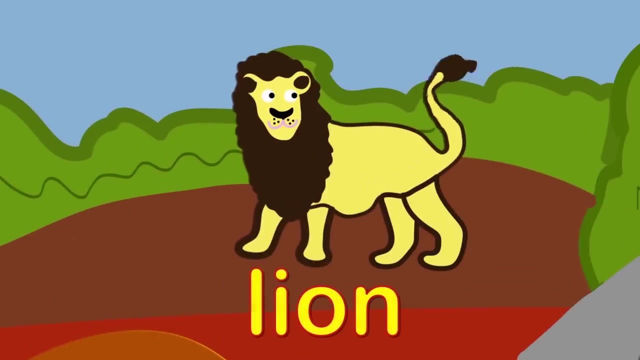 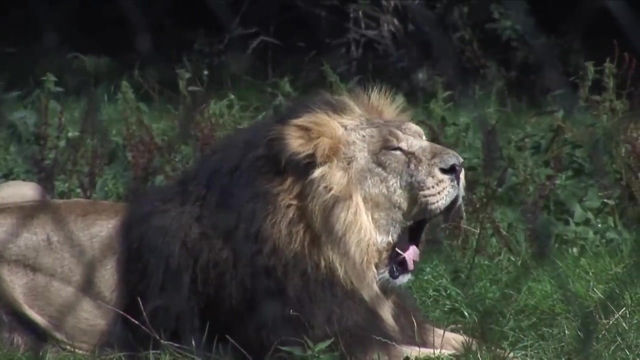 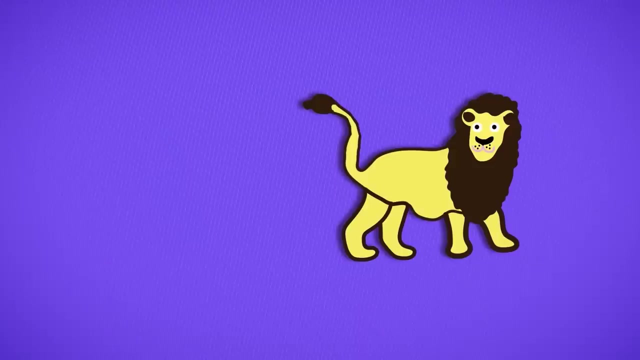 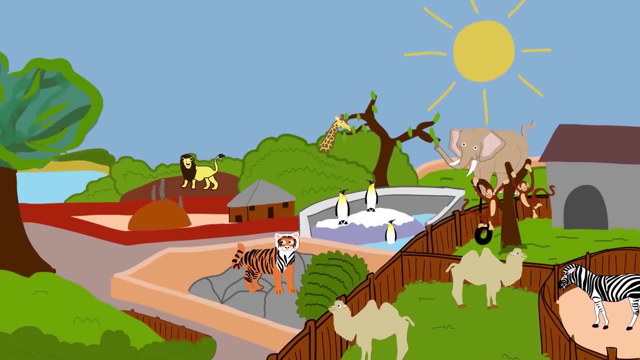 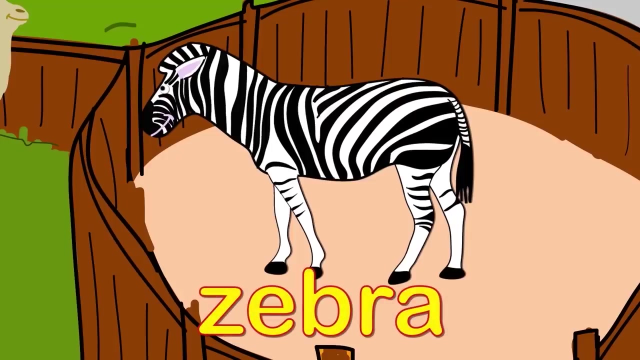 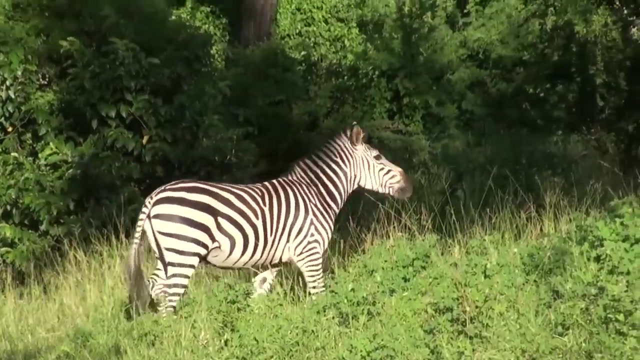 We're flying woohoo. Welcome to Number Zoo. Good morning animals. It's time to wake up. Wakey, wakey. Hello, furry lion. Hello, One one lion. Hello, stripey zebra. Hello, Hello, Hello. 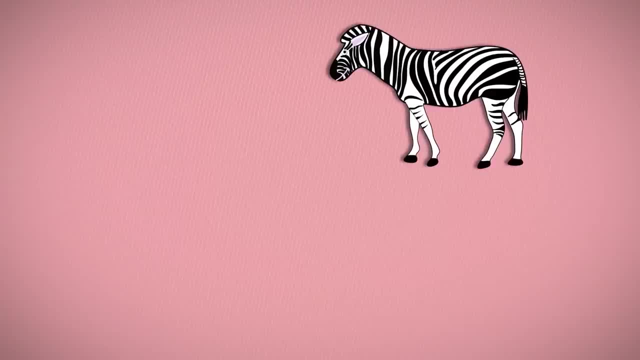 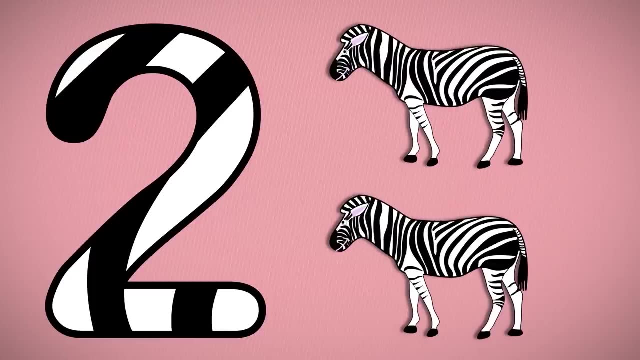 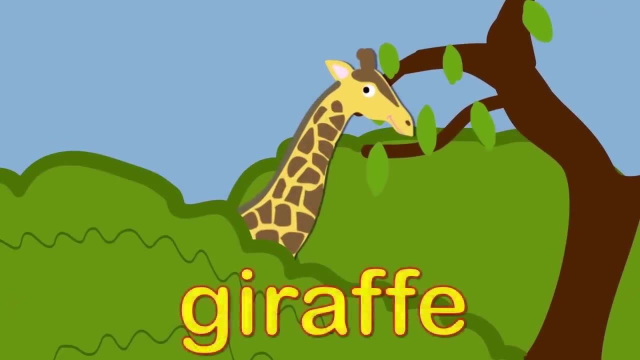 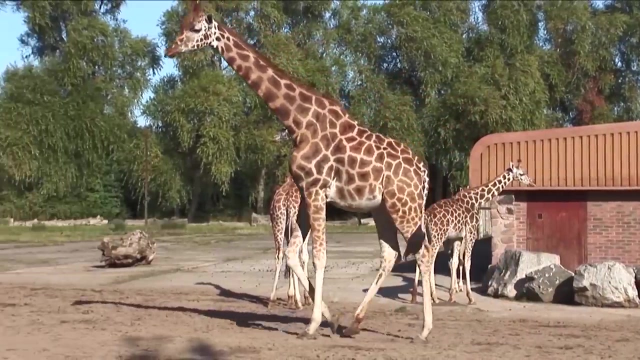 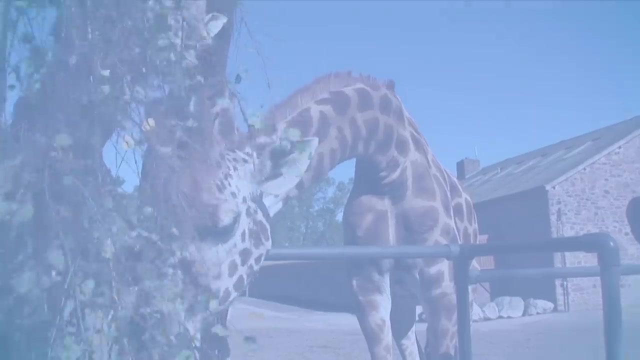 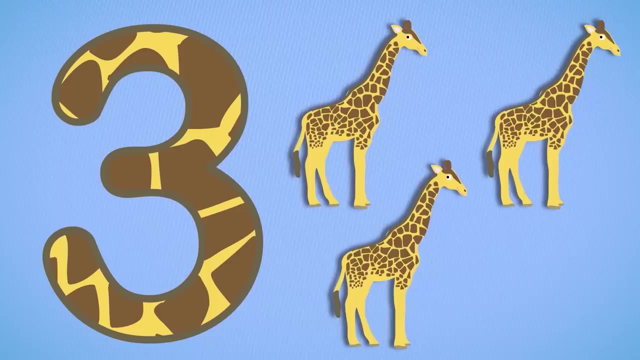 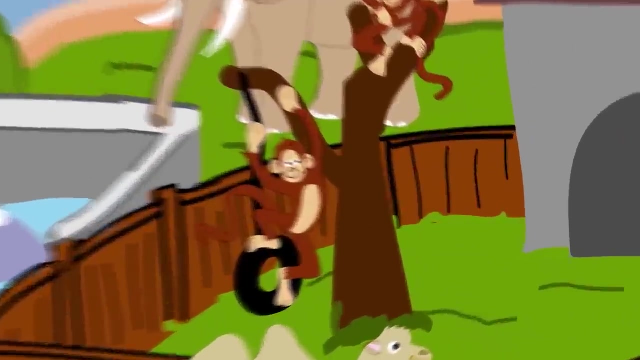 Hello, Hello 1,, 2,, 2 zebras. Hello giraffe My, what a long neck you have. Hello giraffe My, what a long neck you have. Hello giraffe. One, two, three, three giraffes. 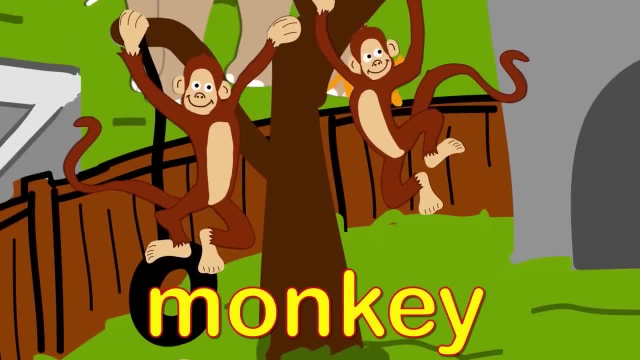 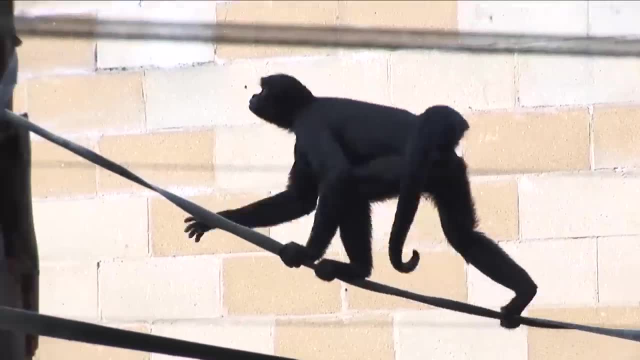 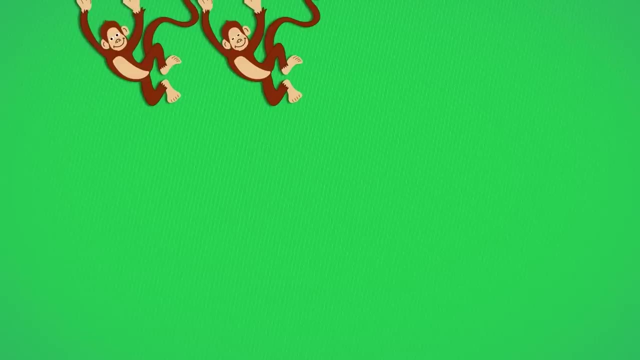 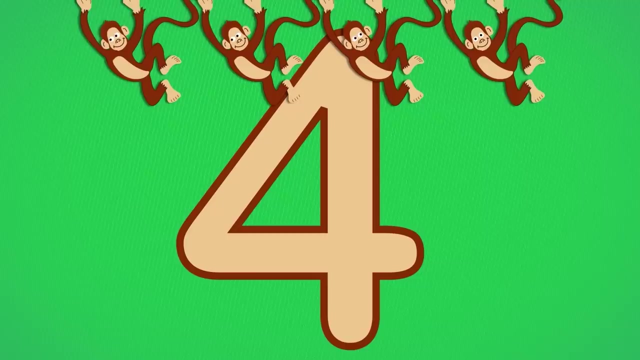 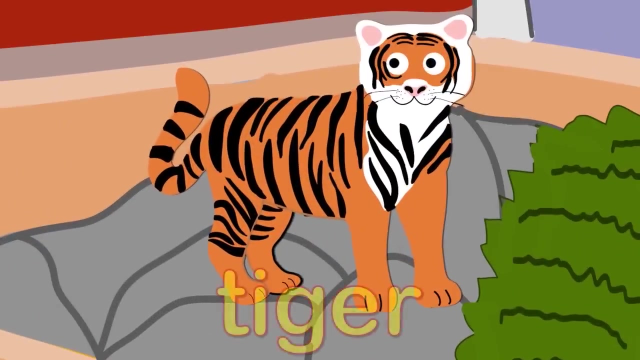 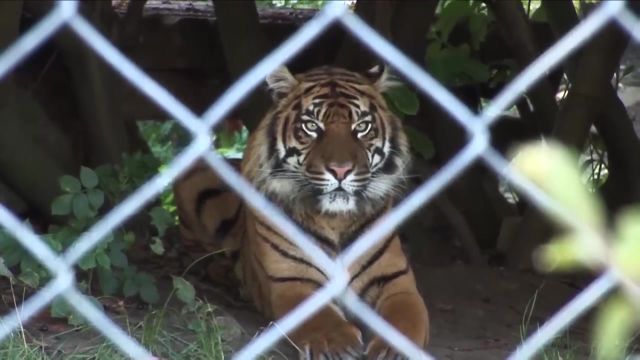 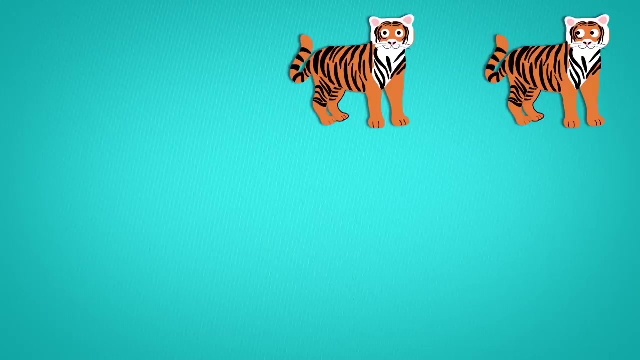 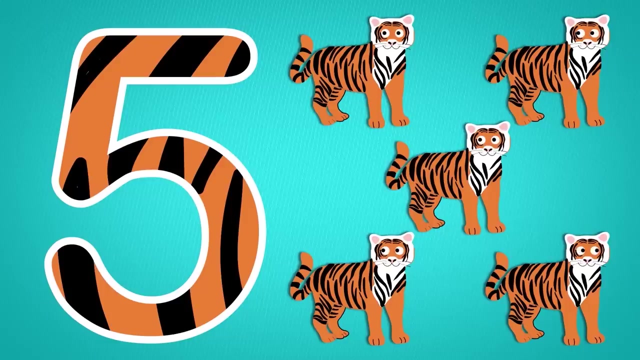 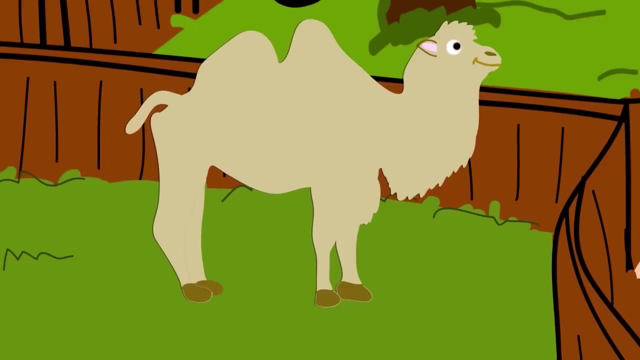 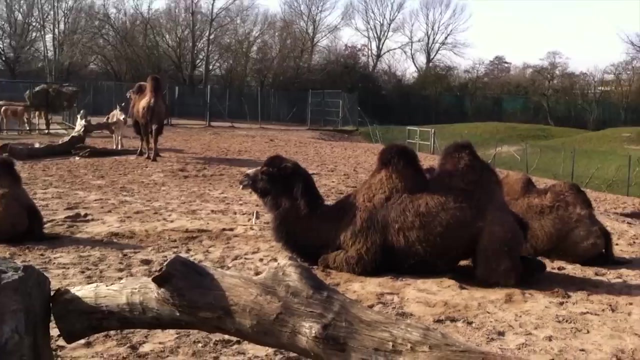 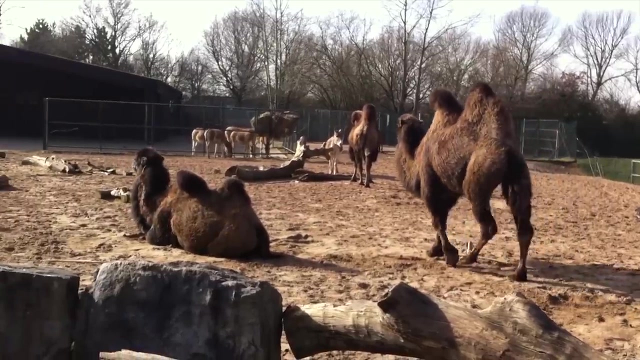 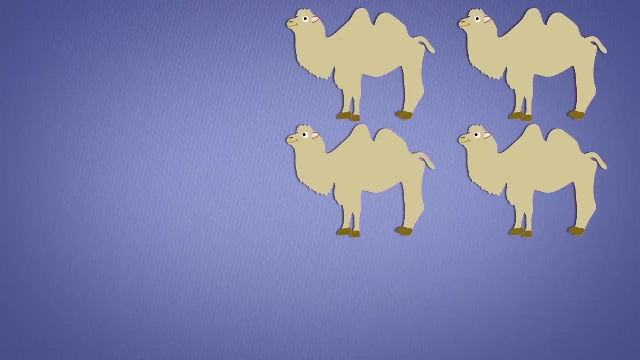 Hello cheeky monkeys. One, two, three, four, four monkeys. Hello orange tiger. One, two, three, four, five, five tigers. Hello humpy camel. One, two, three, four, five, six, six camels. 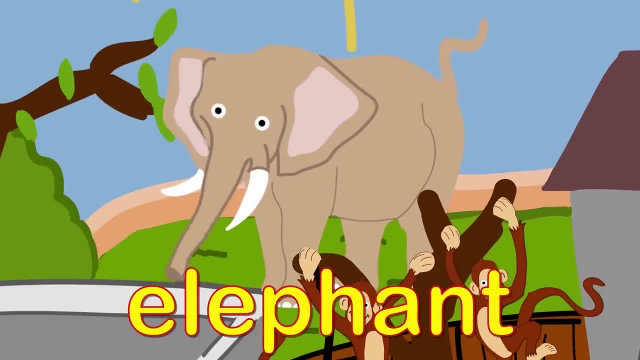 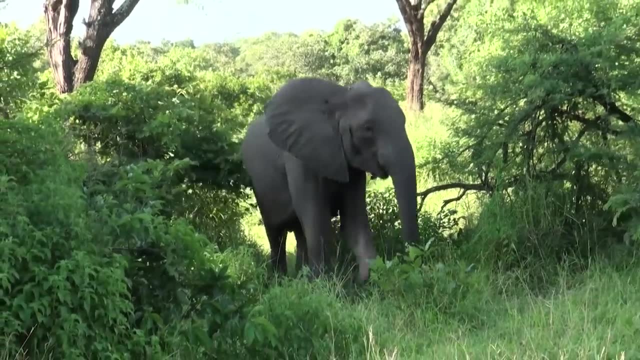 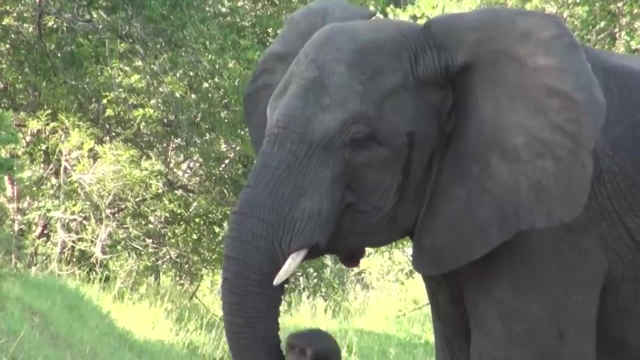 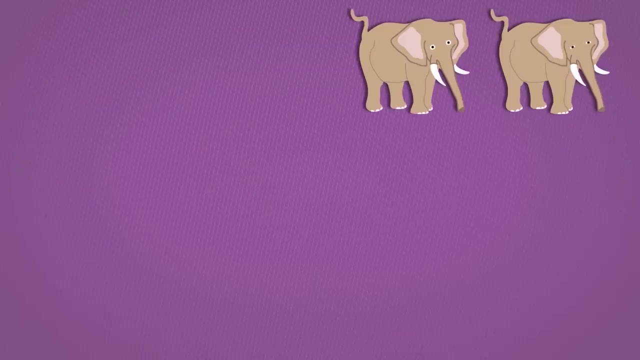 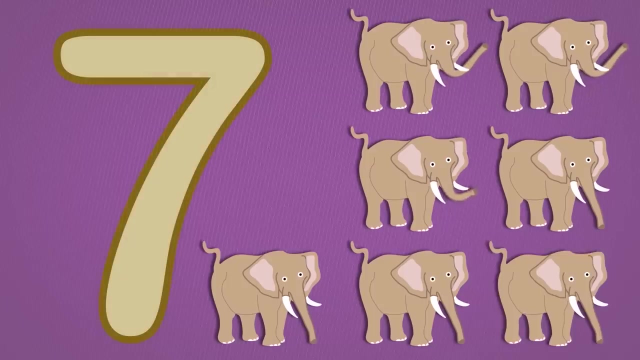 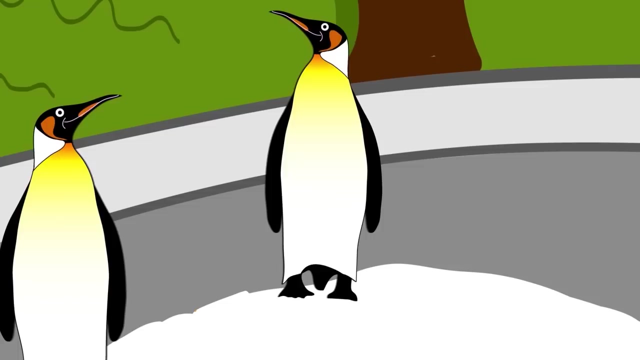 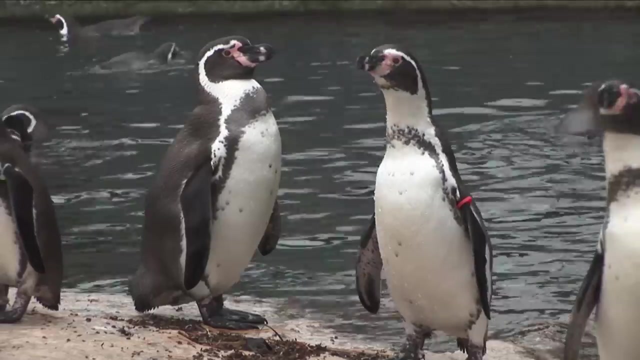 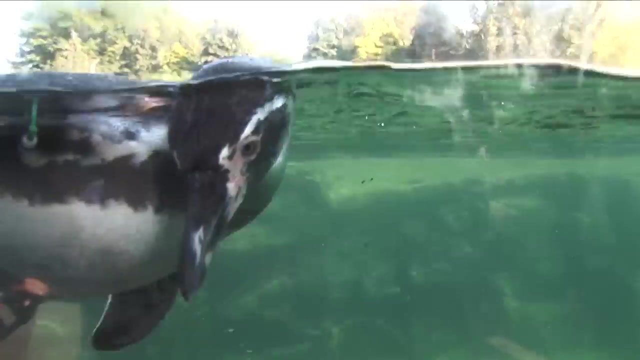 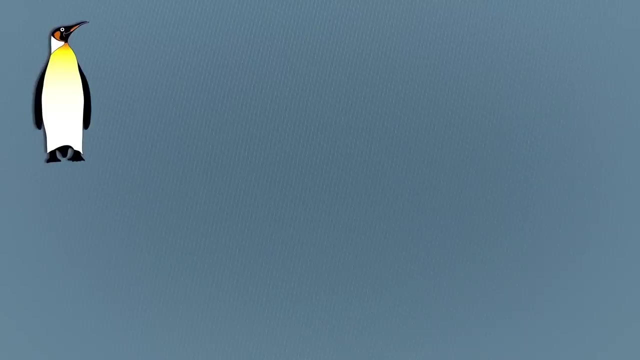 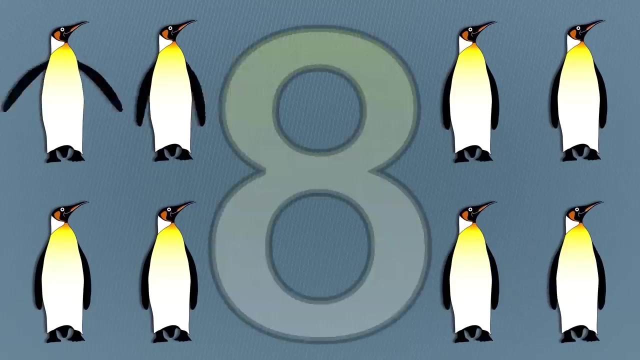 Hello big elephant. One, two, three, four, five, six, seven, six camels, Seven elephants. Hello pretty penguin. One, two, three, four, five, six camels. Seven elephants. One, two, three, four, five, six, seven, eight, eight penguins. 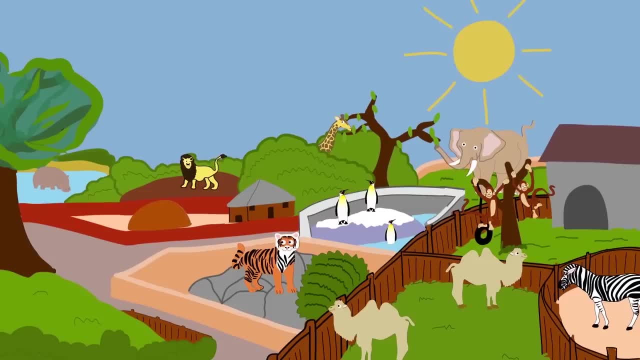 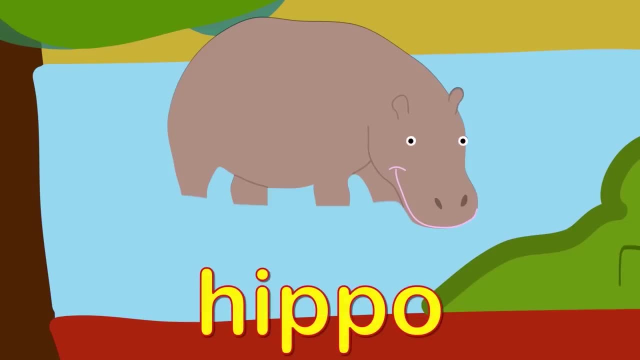 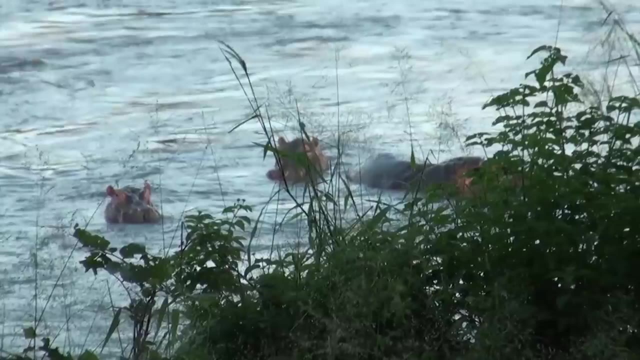 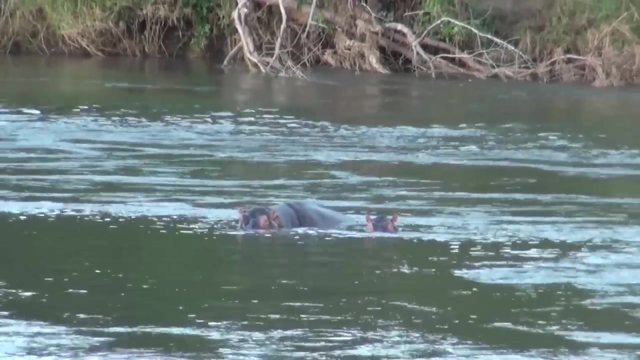 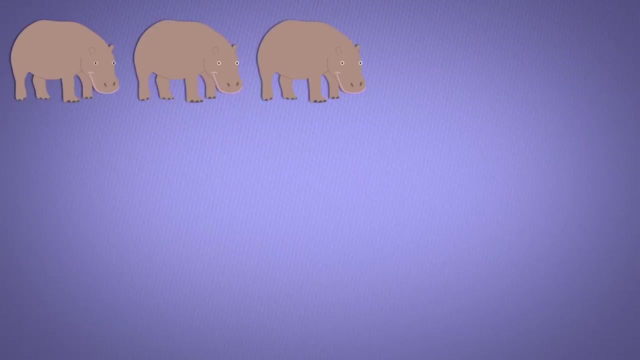 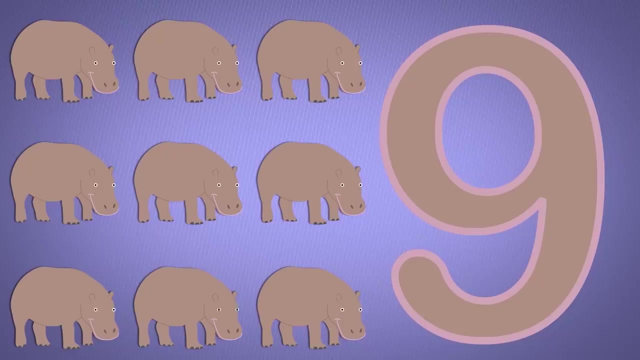 One, two, three, four, five, six, seven, eight penguins. Hello hungry hippo. Hello hungry hippo. Hey little Kiwi. Hey little Kiwi. 1,, 2,, 3,, 4,, 5,, 6,, 7,, 8,, 9,, 9 hippos. 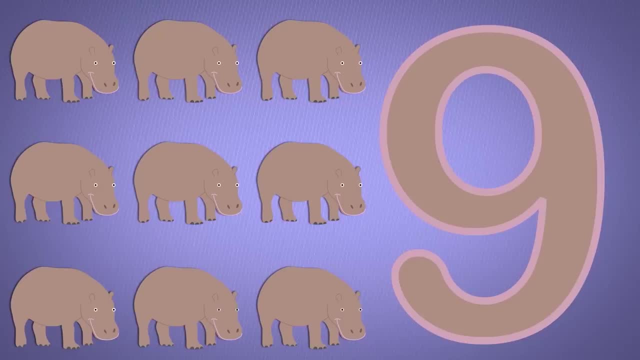 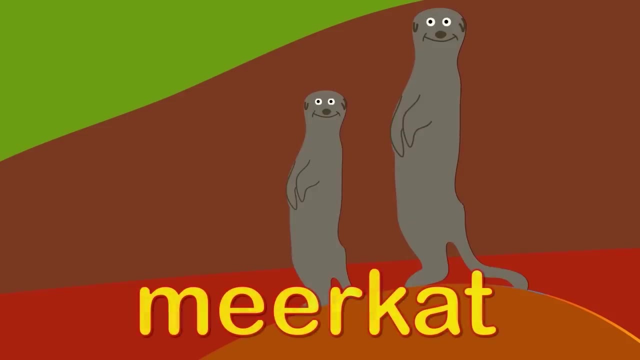 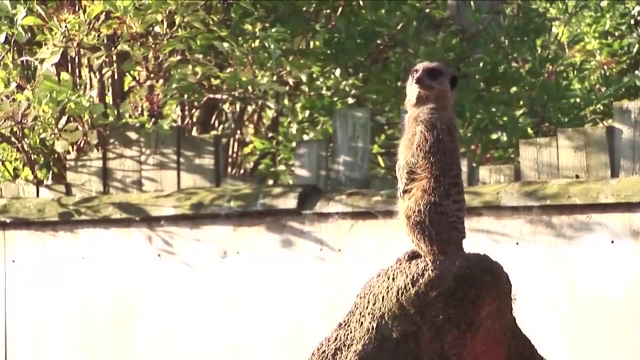 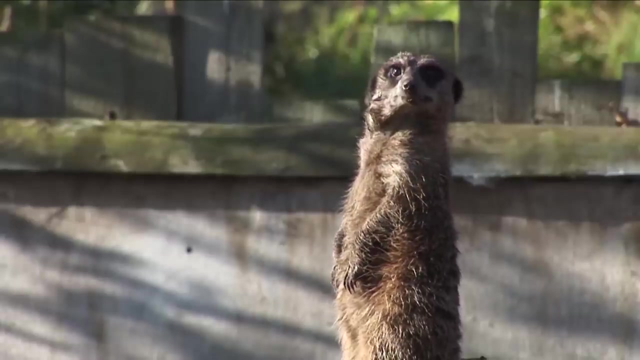 Hello nosy meerkat. 1, 2,, 3,, 4,, 5,, 6,, 7,, 8,, 9, 10. 1, 2,, 3,, 4,, 5,, 6,, 7,, 8,, 9, 10. 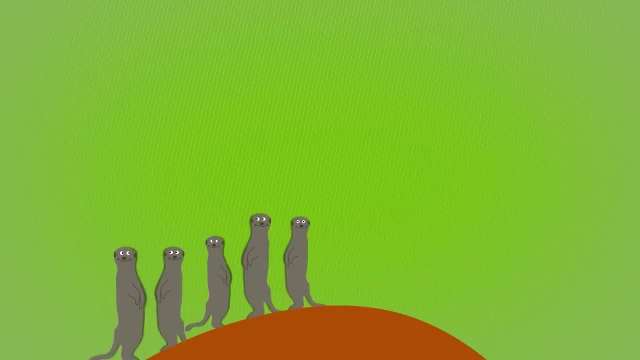 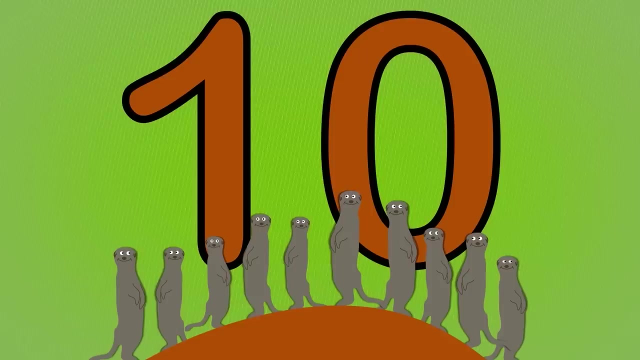 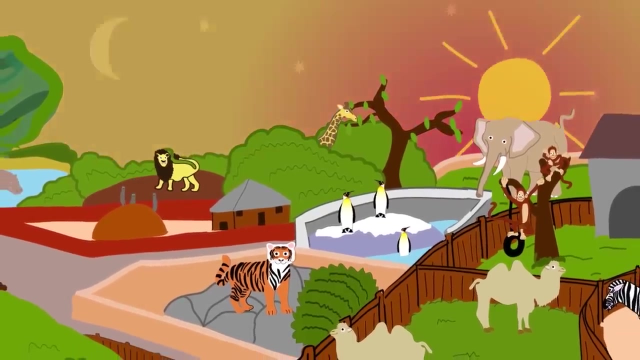 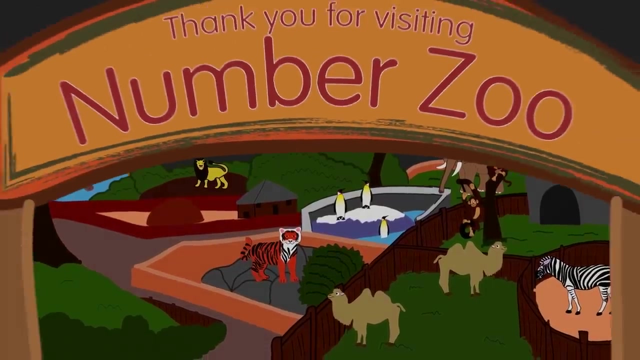 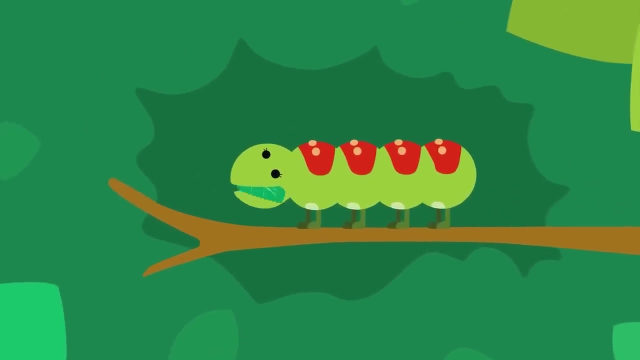 1,, 2,, 3,, 4,, 5,, 6,, 7,, 8,, 9,, 10, 10 meerkats. Goodnight animals sleep well. Thank you for visiting Number Zoo. See you again soon. Aren't you full yet? 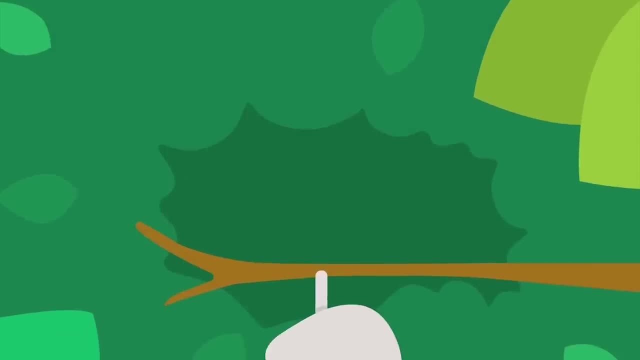 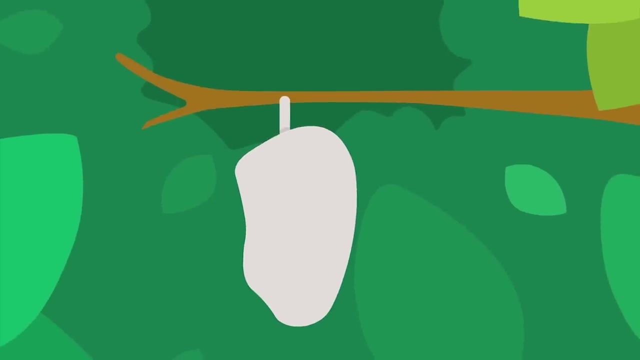 You've been eating all day Caterpillar, caterpillar. How very weird She was by that green leaf. Now she's just disappeared. But how can this be When she's not left my sight? And where did that come from? That shape, That shape There? that's white. 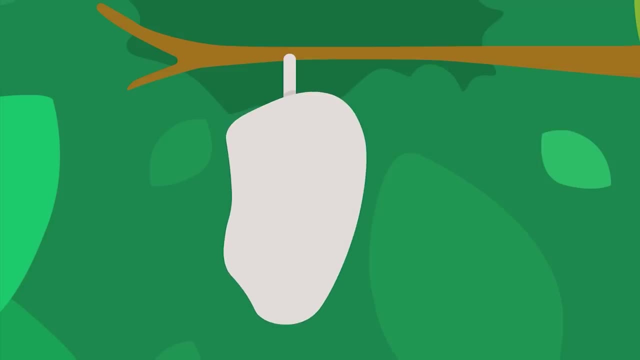 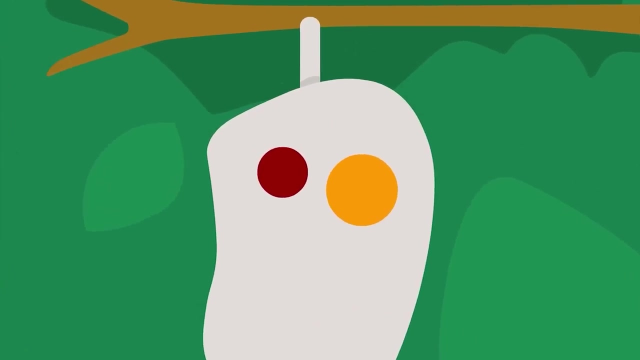 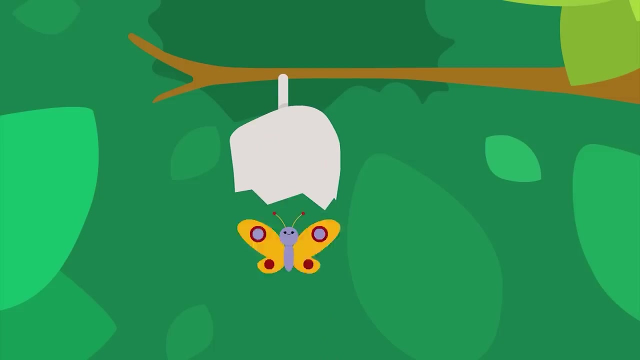 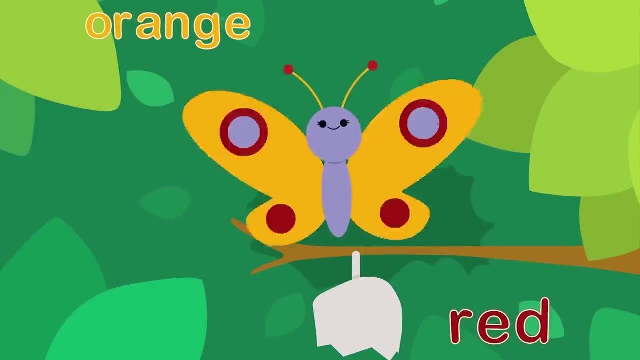 And now it's just moved And there's colours inside. It must be a monster And those are its eyes. Wait, hang on a minute. That's not a monster, But wings in the sky Of an orange and red coloured butterfly. My caterpillar was here All along. 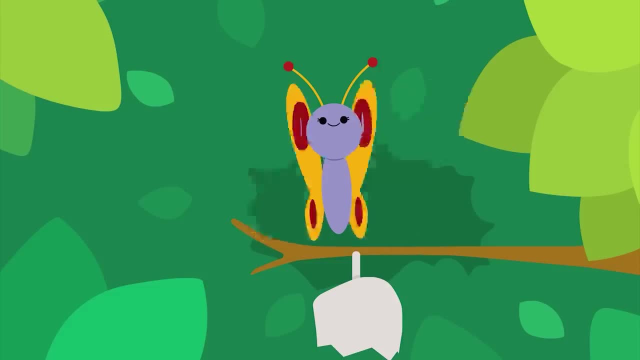 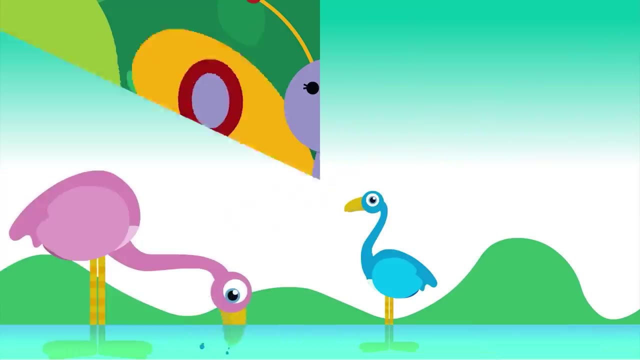 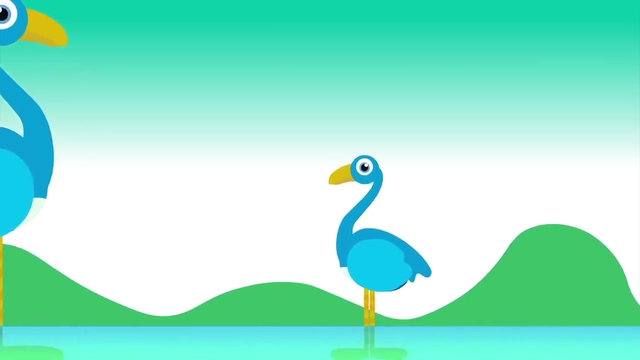 She was just changing Into a flut, flut, Fluttering butterfly. Wow, Oh, poor, poor flamingo, I've lost you, I think. Can anyone find him? His colour is pink. No, no, He is pink. That's not me, That's not my blue bird. 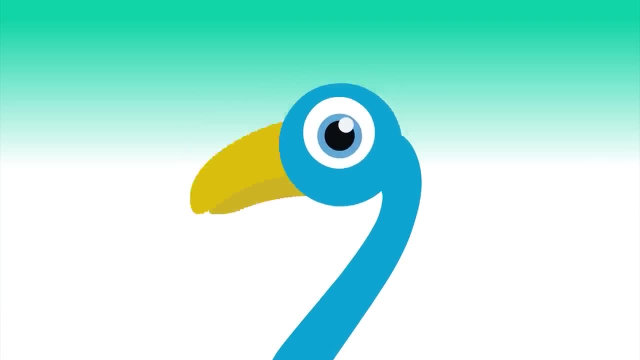 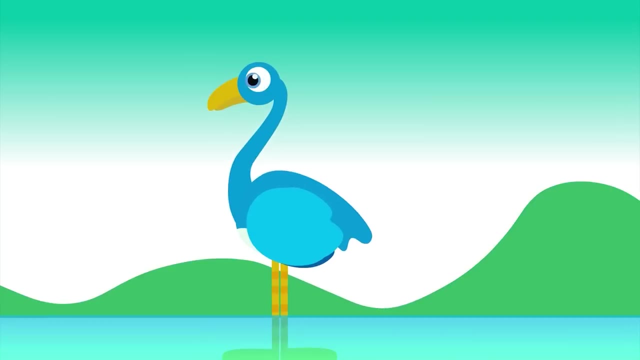 What Flamingos change colour? Don't be so absurd. They can't simply change their colour or hue. They can't simply change from pink into blue. Well, that must be the strangest thing I've ever seen, That once blue flamingo has now turned quite green. 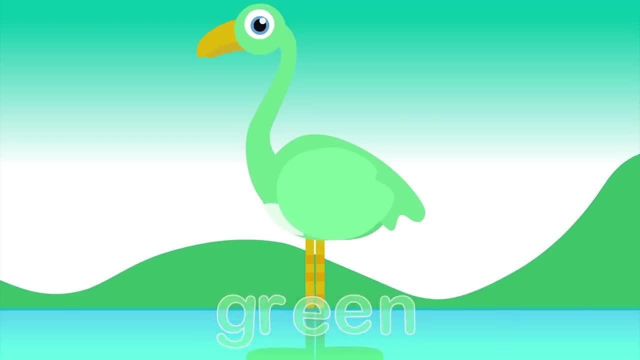 Well, that must be the strangest thing I've ever seen, That once blue flamingo has now turned quite green. What a shock. So it was my flamingo all along. He'd just changed to the colour of his food. I think we need to feed him some nice pink shrimp. 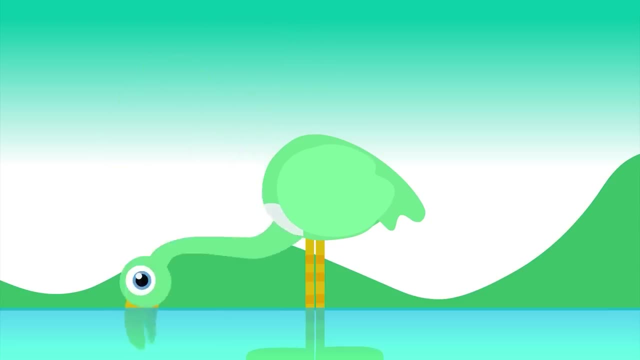 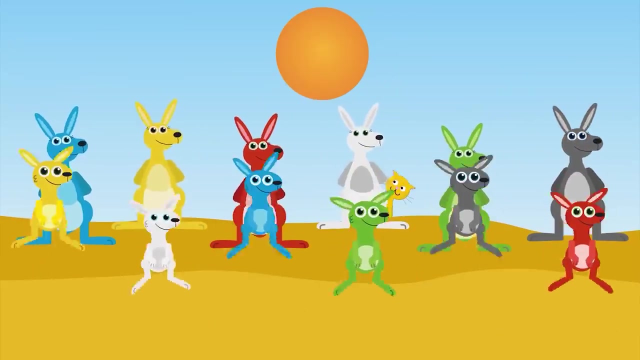 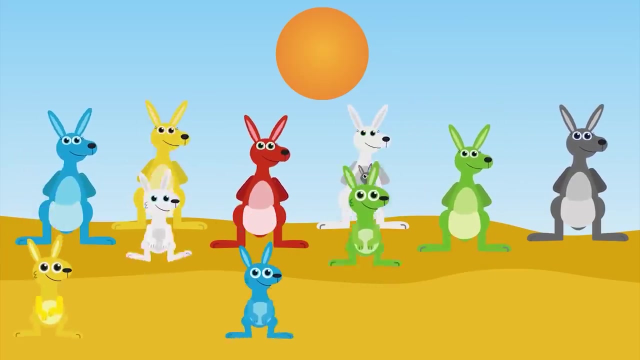 So he can change back to pink again, Don't you? Ah, that's better. Hello Green Roo, Are you having fun playing with your friends? Yes, I hope everyone has a lovely day. Have fun with all your friends And don't forget to subscribe to my channel. 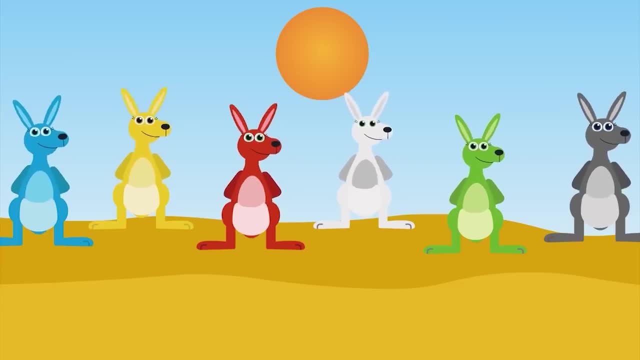 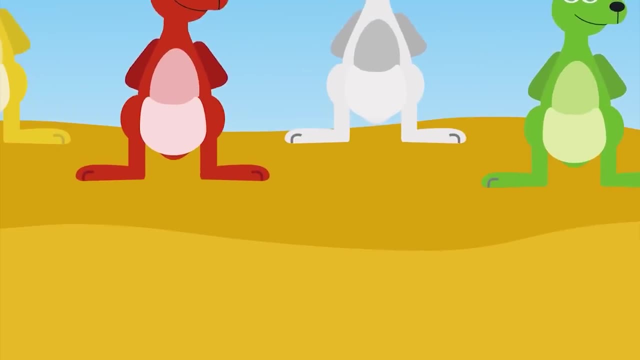 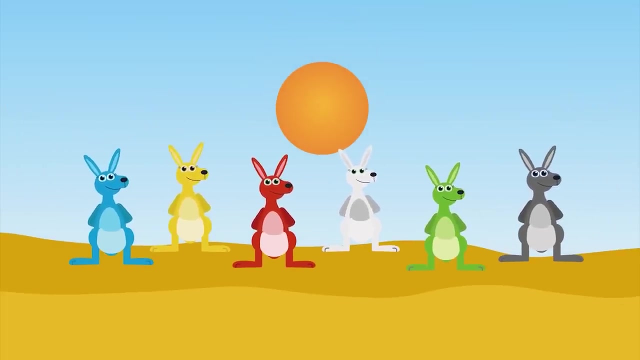 So that I can get your likes and comments. Bye, I've lost my Roo. Has anyone seen? He jumps very high And his colour is green. He was hopping right here with his friends. Now he's gone. What He jumped in the pouch of a mummy. 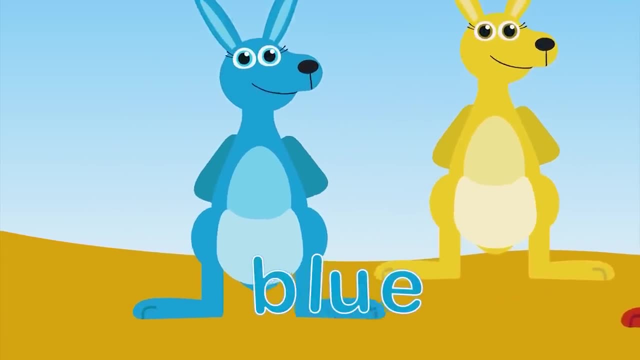 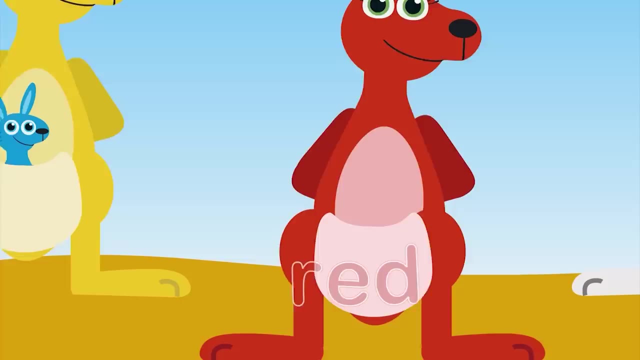 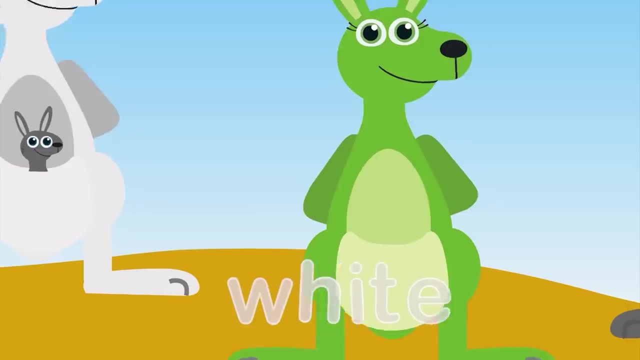 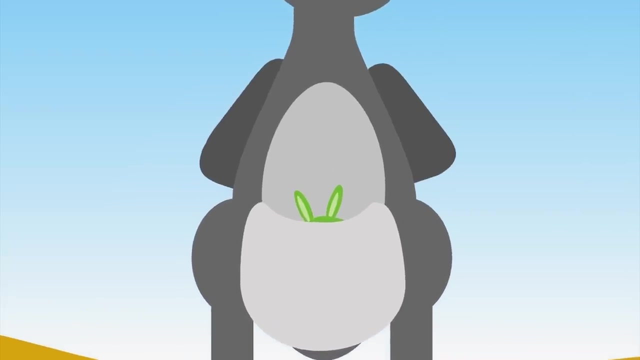 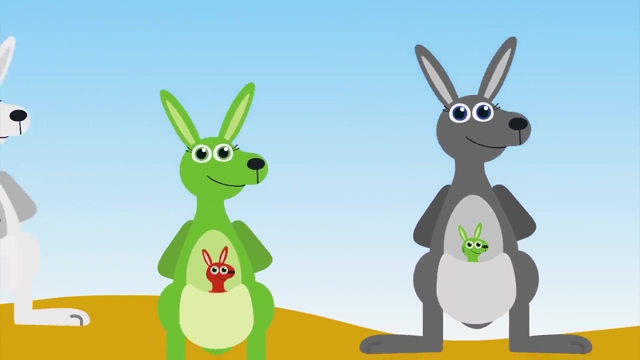 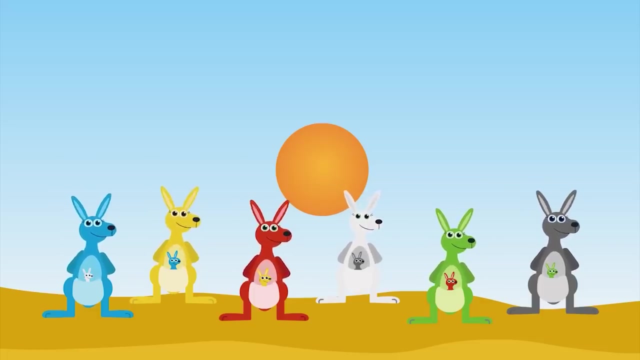 did he jump in? the blue one: no. the yellow one, no. or red, no. the white one, no. the green one, no. oh, look, there's his head, hooray, there he is in the mummy who's grey, but now he won't come back, he just wants to stay. goodbye, baby Roo. oh well, I can't say I blame him. can you, are you ready to? 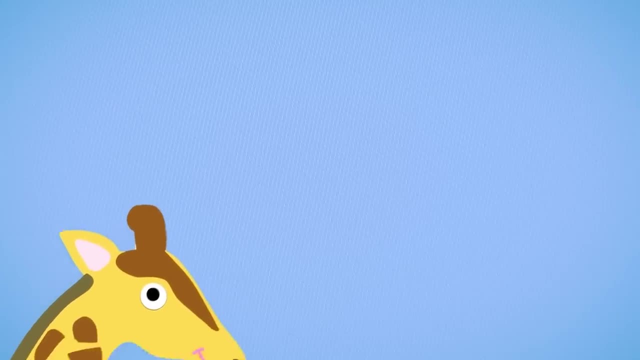 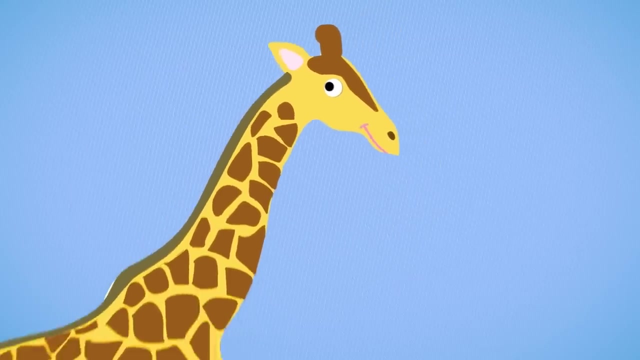 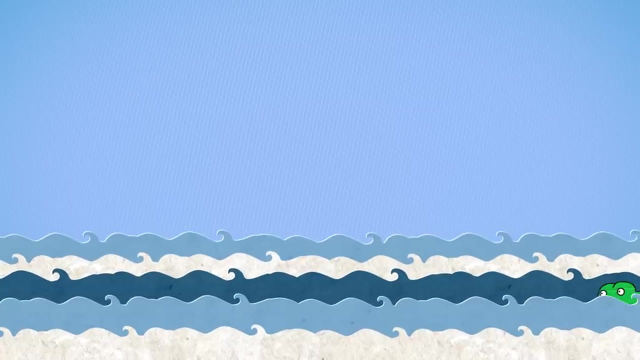 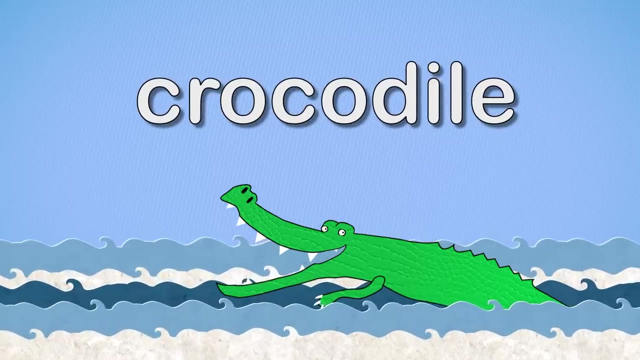 have some fun. let's see who's animal number one with his very long neck. you must be a giraffe with a cheeky grin and green, scaly skin. this is one animal you don't want to get in the water with. it's a crocodile. 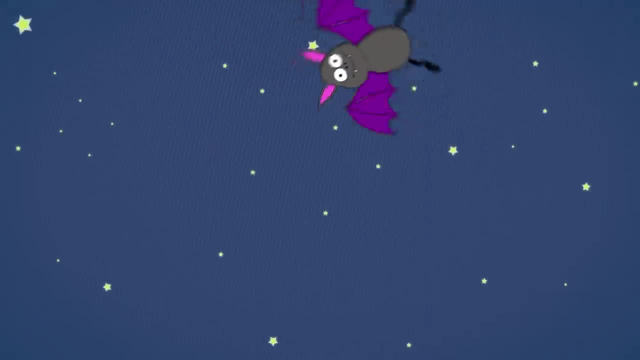 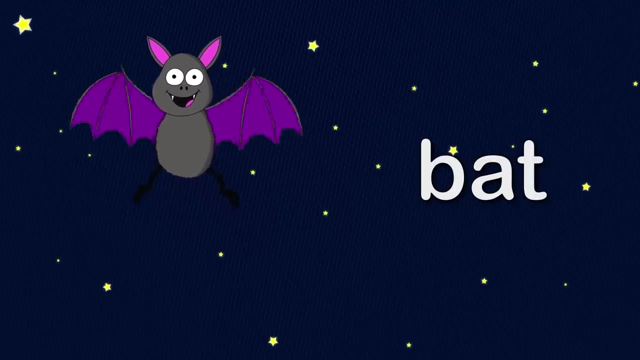 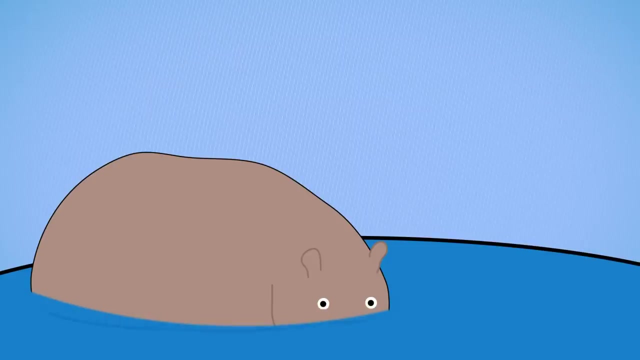 during the day you sleep upside down and only come out to play at night. you must be a bat. where's our next animal? oh, there you are. you can hold your breath underwater for a long time. wow, you're huge. you're a hippopotamus, or hippo for short. 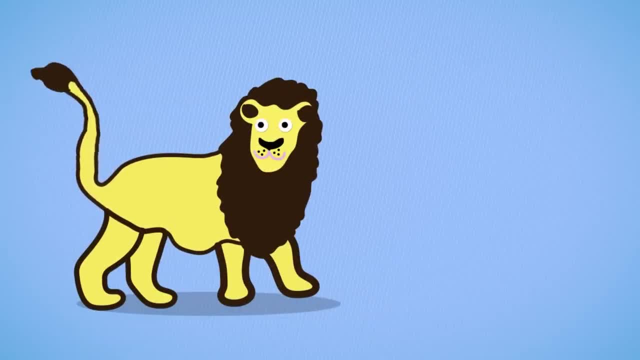 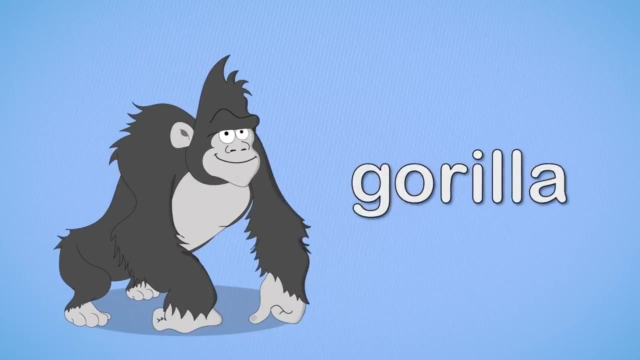 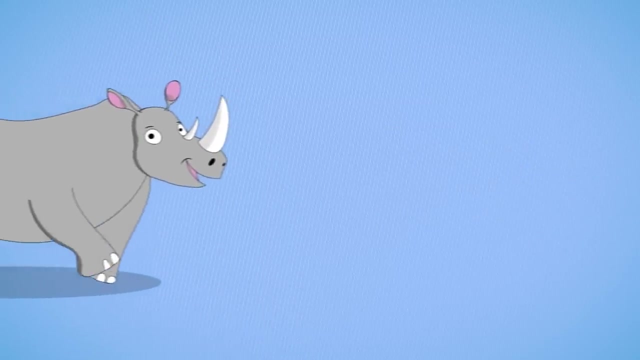 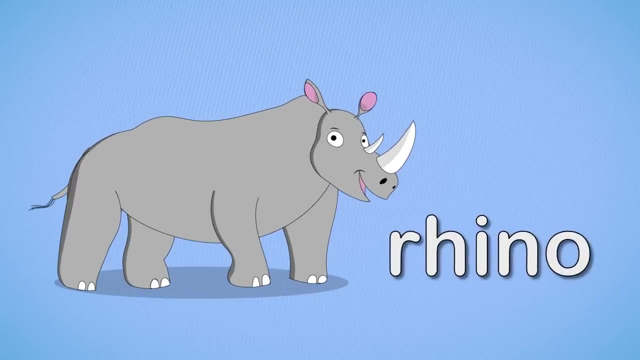 you're a very big cat. I love your fluffy mane around your neck and your beautiful yellow coat. it's a lion, big and hairy, with long, strong arms- hello gorilla. thick grey skin and a large pointy horn on your nose. you're a rhinoceros, or rhino for short. 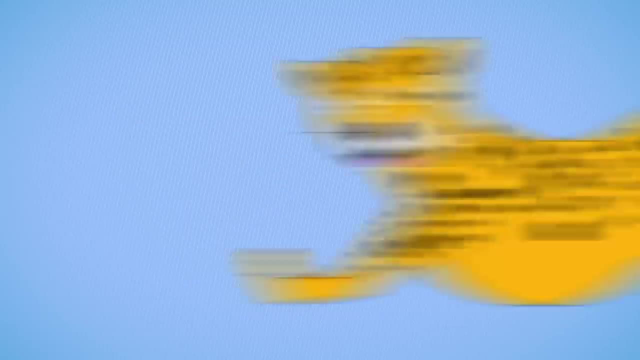 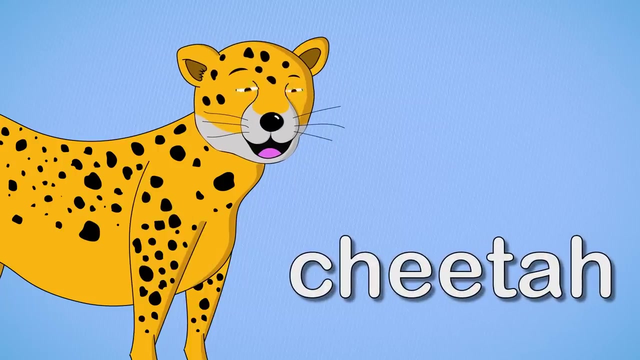 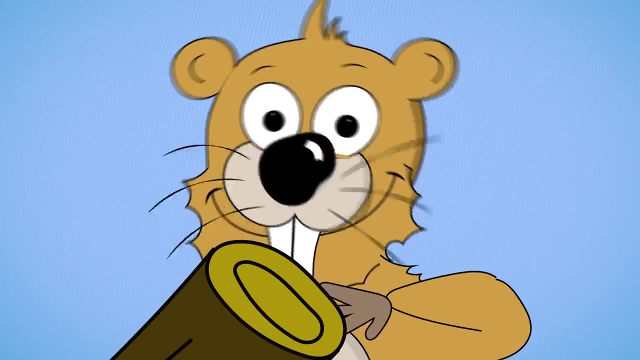 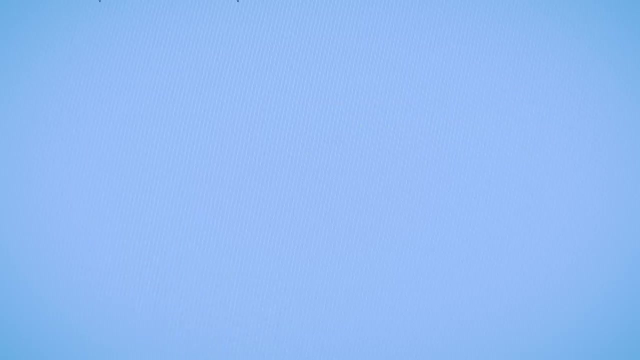 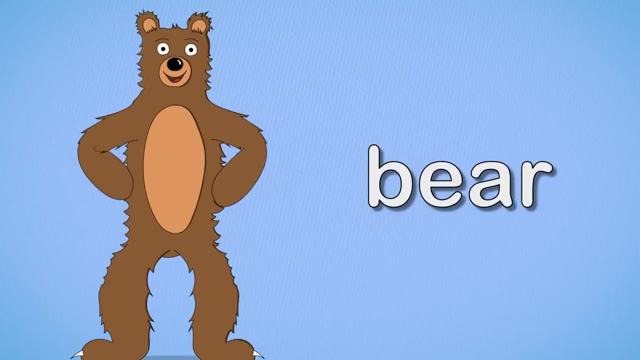 whoa, what was that? it looked just like a cat. oh, it's the fastest animal on land. it's a cheetah- big front teeth for munching on wood. hmm, you must be a beaver. you're big, brown and furry and you look very, very strong. I think you're a bear. 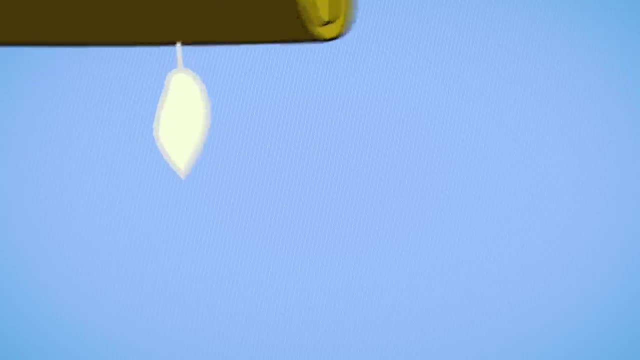 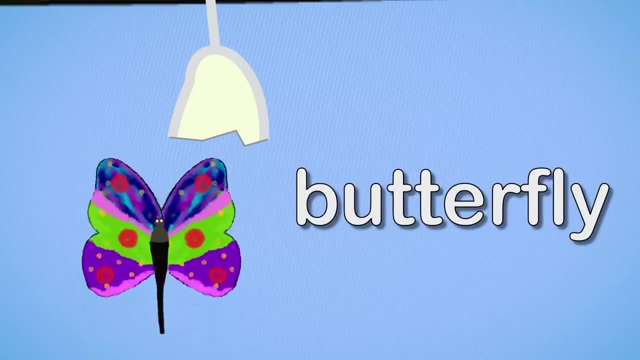 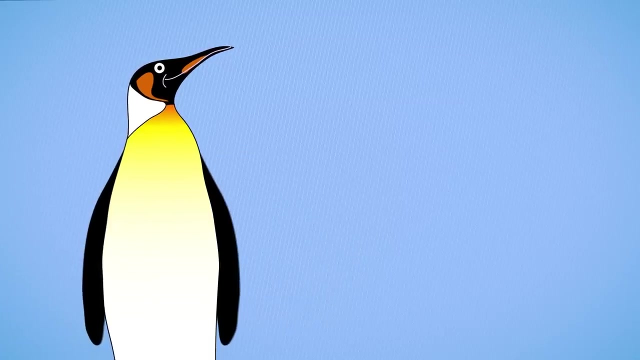 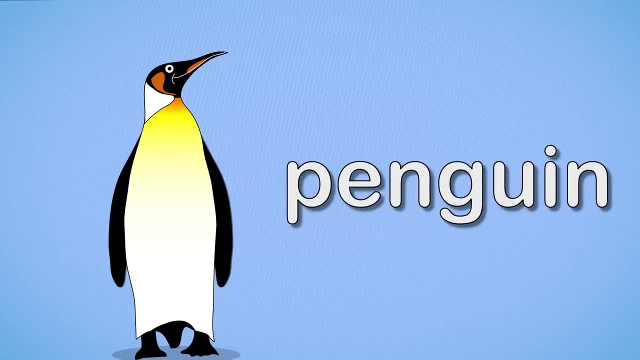 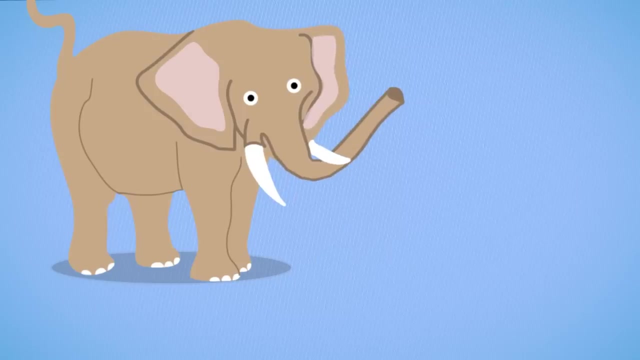 what's inside that white cocoon? look, it's coming out there. it's a beautiful butterfly. okay, so you're a beautiful black, white and orange bird, but you can't fly. oh, it's a penguin. look, it's the biggest land animal in the world with that long trunk and beautiful white tusks. 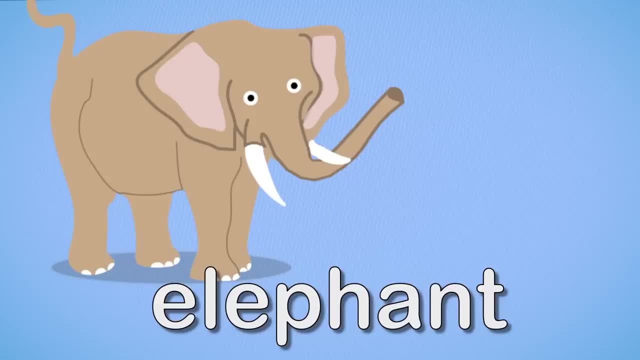 there's no doubt that you're an elephant. i love it too. الع. 왜냐하면這是一个红白的小貓? there's no doubt. here we go a little closer, like we're a dragon or a squirrel. i'm a monkey, but never a squirrel. 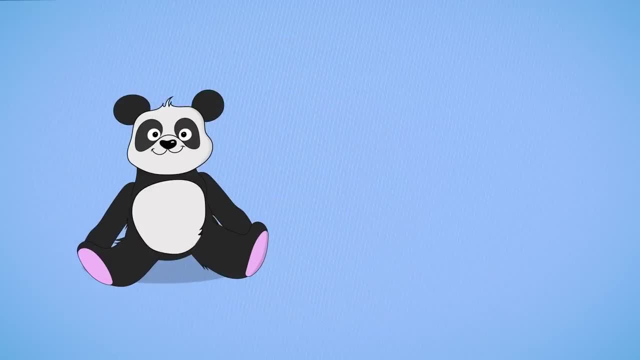 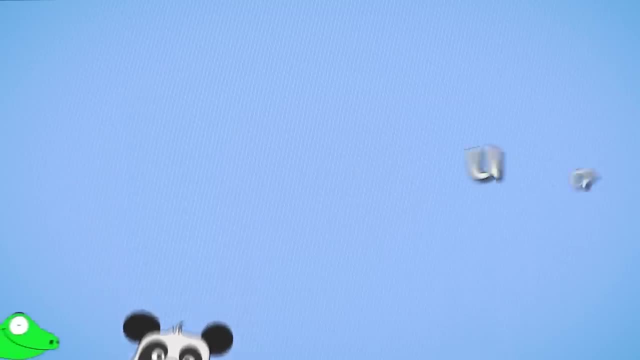 You're a black and white bear and very, very cute. It's a panda With no arms or legs. you're a reptile who slithers along the ground. There's only one thing: you could be A snake. Hello. 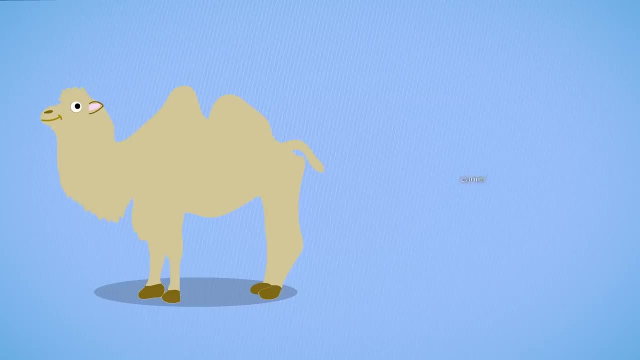 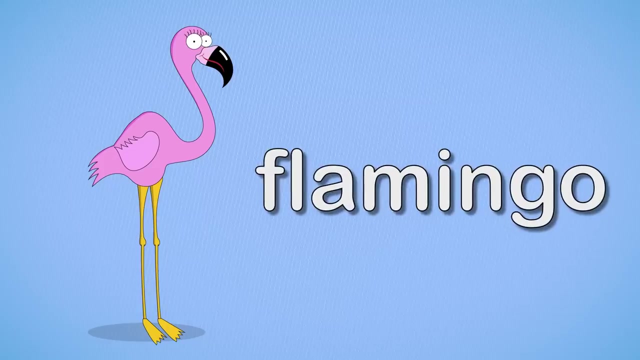 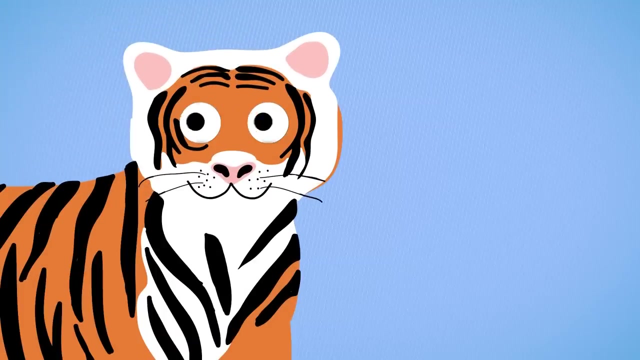 Look at those humps on your back. are they used for storing water? You must be a camel, A bright pink bird with a long neck. It must be a beautiful flamingo. Here's another big cat with stripy orange and black fur. 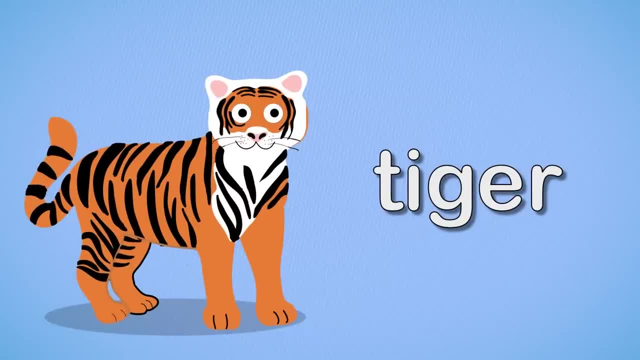 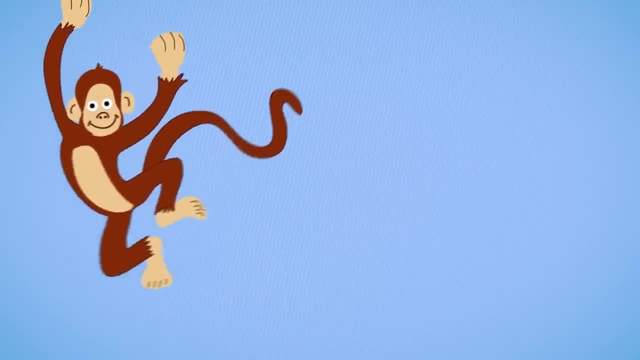 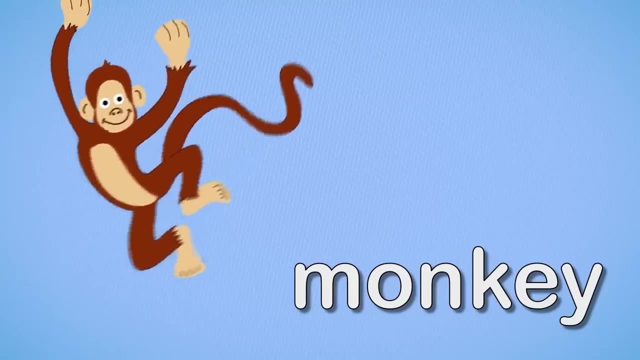 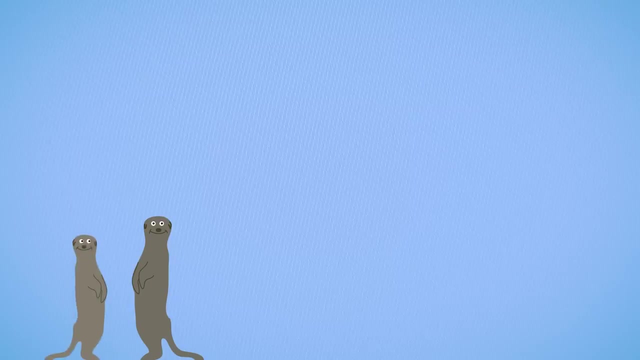 It can't be anything. You're a tiger. Hello, funny swinging creature. Look at your long tail. I know what you are: You're a monkey. Hello, small furry thing. Oh, hello to your friend too. And your other friend, Or are they your brothers and sisters? 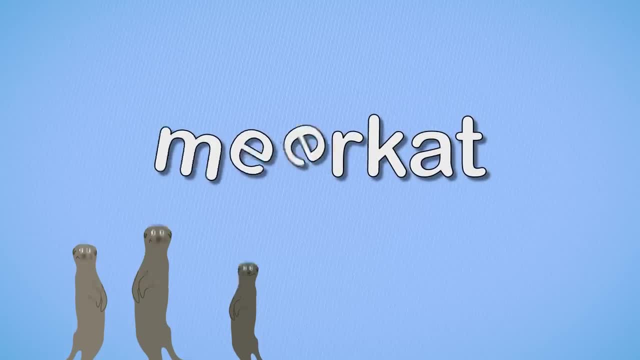 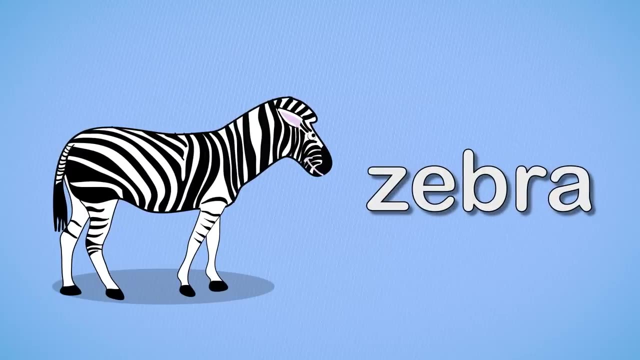 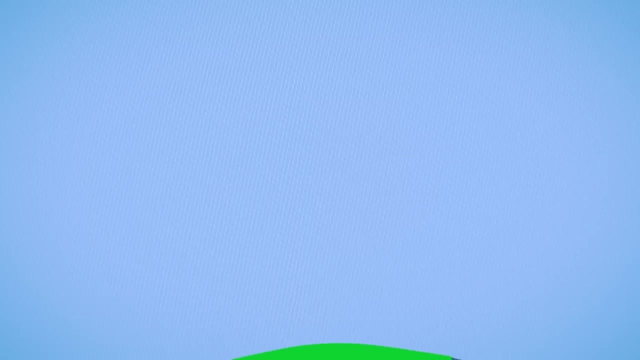 You're a meerkat. Hello, You look like a horse, but you have the most amazing black and white stripes. You're a zebra. There's so many amazing animals that live all around the world. They're all different and unique, just like you. 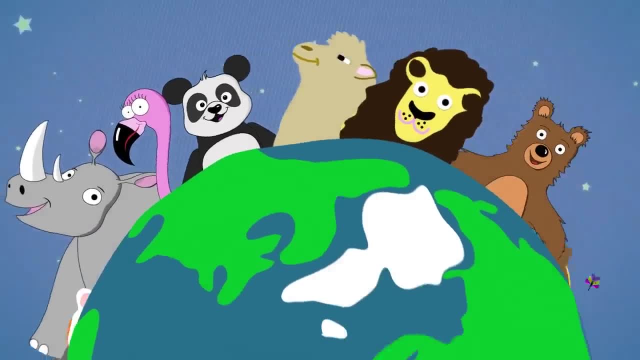 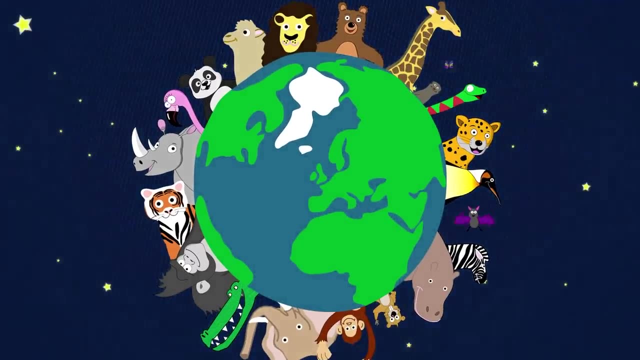 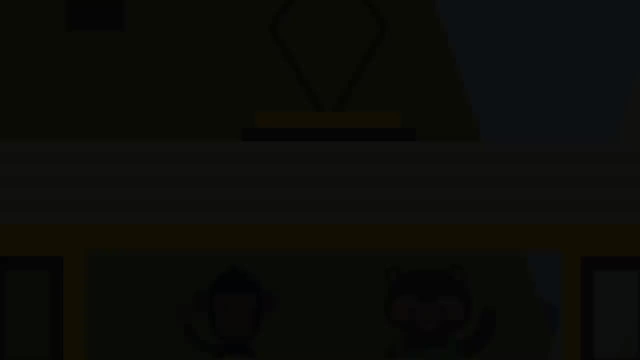 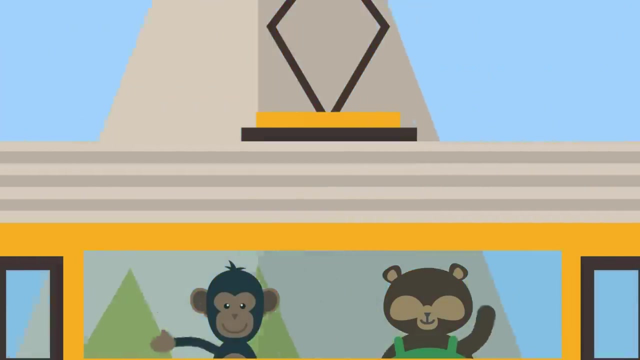 We must work hard together to look after them. Hello, Hello, Hello, Hello, Hello, Bye-bye animals, I love every single one of you. Welcome to train or plane. play along with us. What do you think this is? Is it a train or is it a plane? 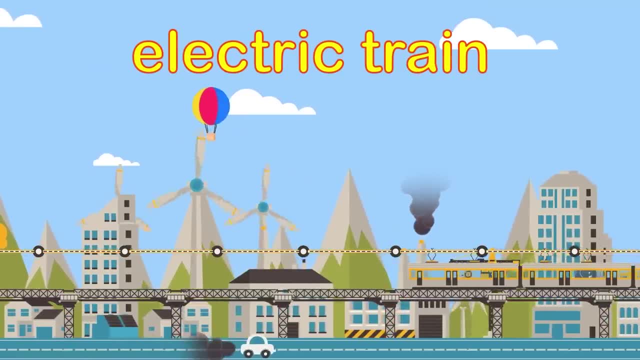 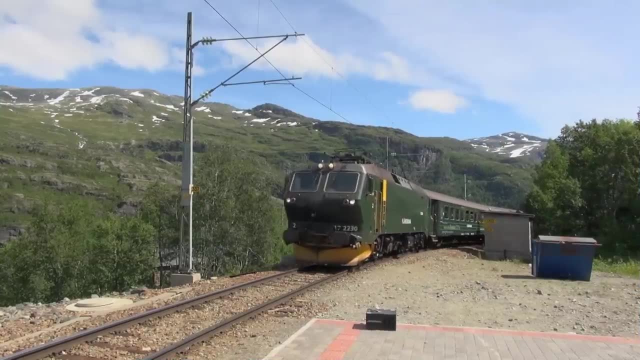 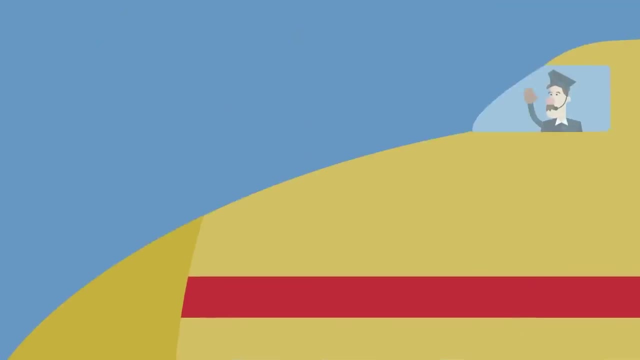 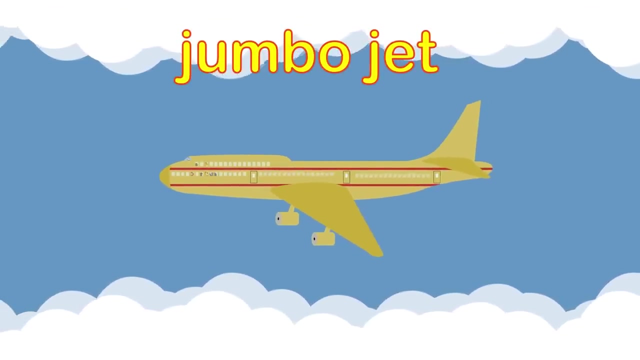 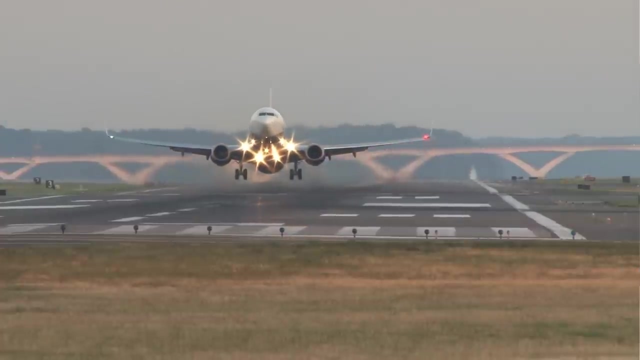 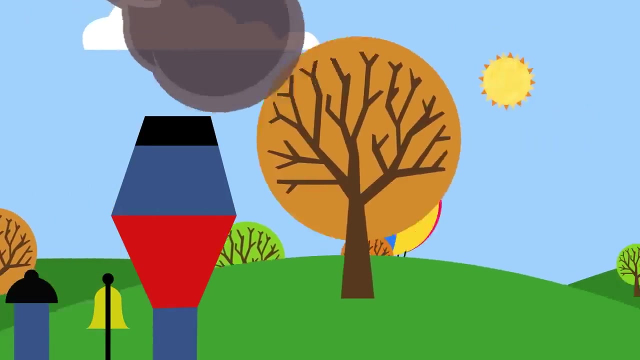 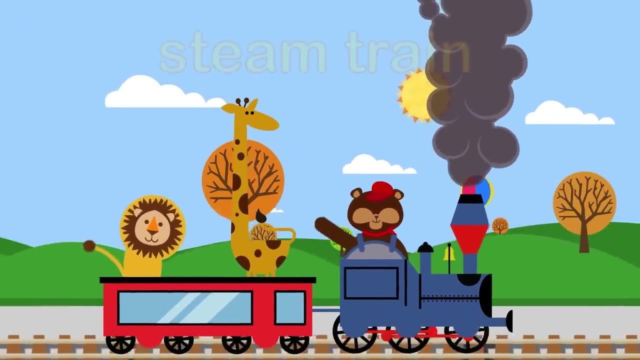 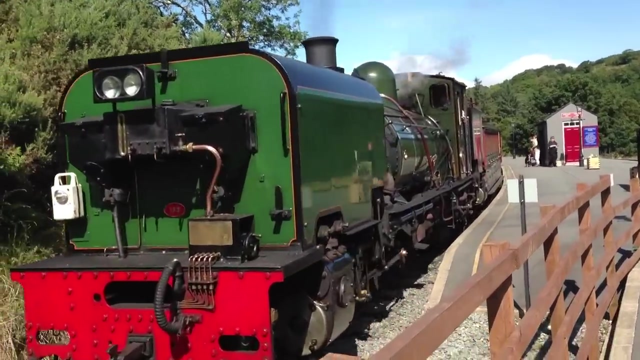 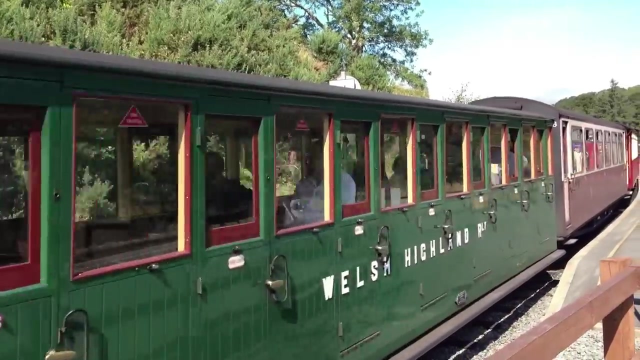 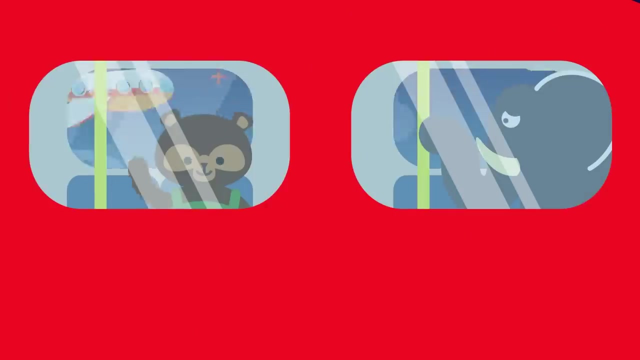 It's an electric train. Oh, How about this one? is it a train or a plane? It's a very big plane. it's called a jumbo jet. I Wonder what this one is. Can you guess? train or plane? It's a steam train. Oh, There's another one. look closely. is it a train or a plane? 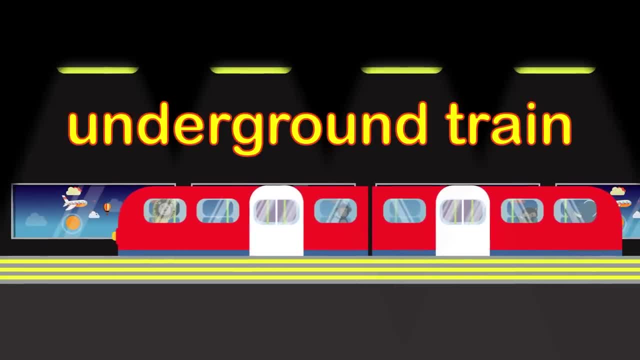 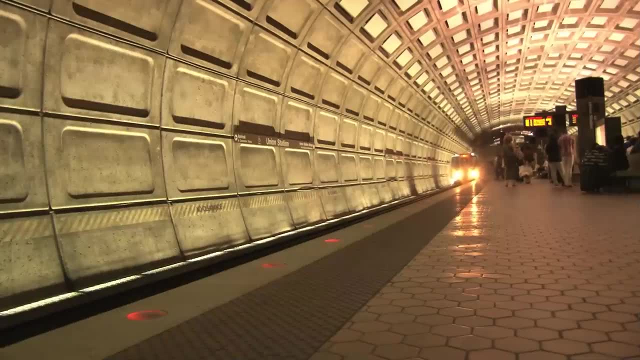 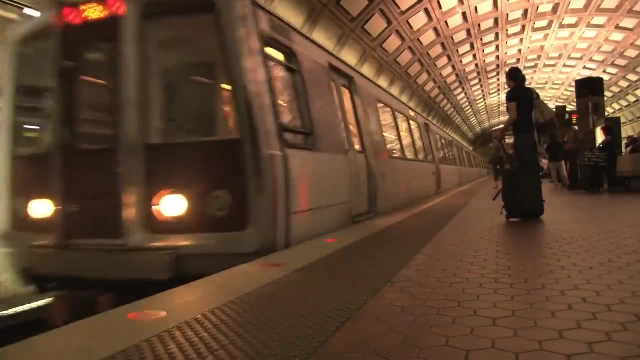 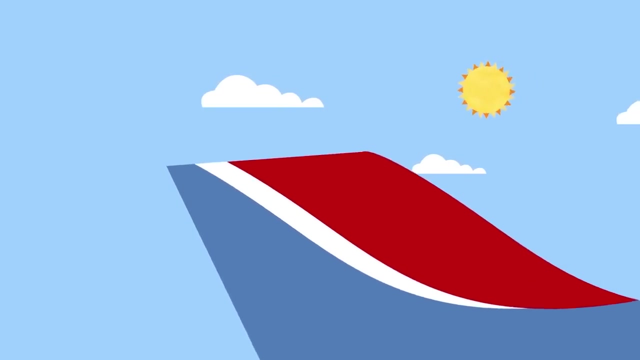 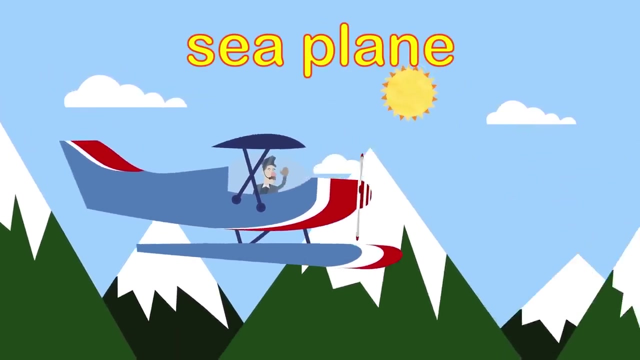 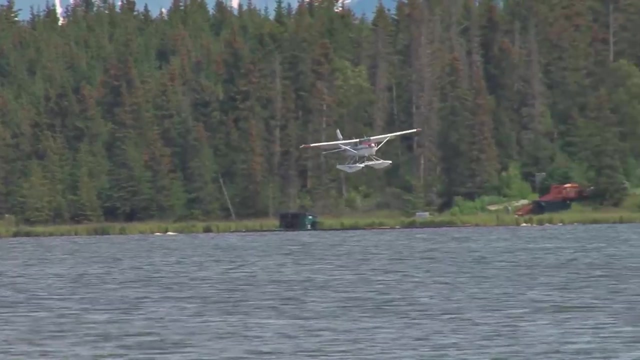 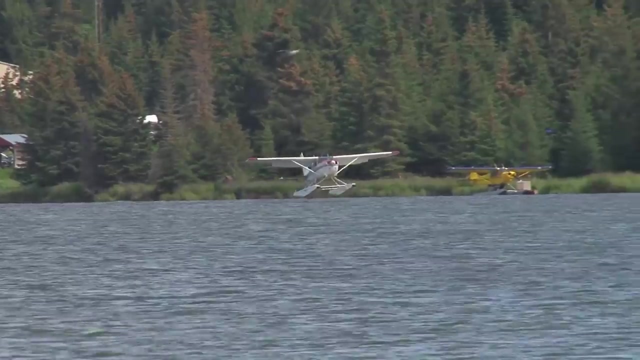 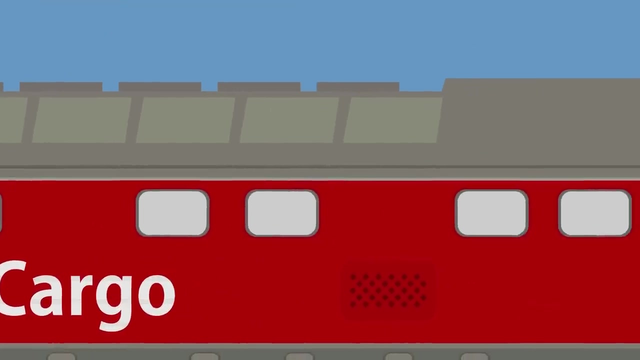 It's an underground train. It's an underground train. Have a look at this one. Do you think it's a train or a plane? It's a seaplane. It's a seaplane. How about this one? It's got a big wing. Yes, it's a big thing. There's two rails: on one side There's a huge one and the other's in the other, middle of them. 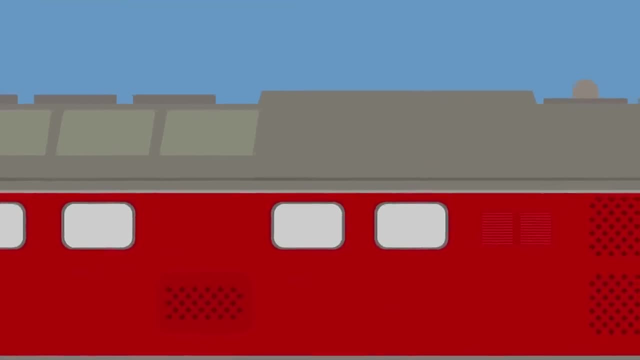 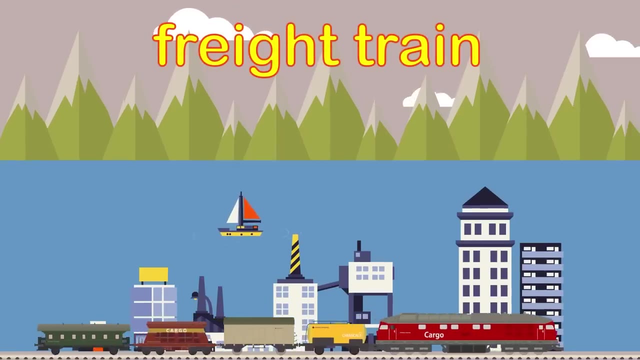 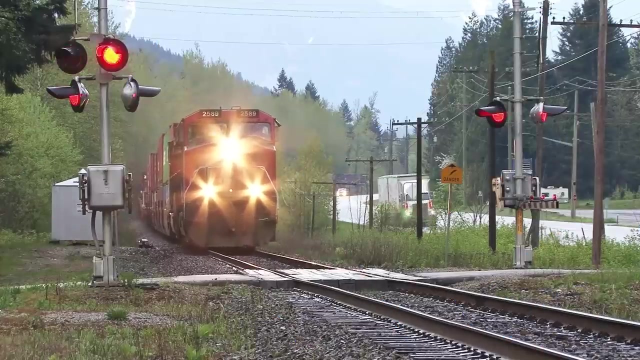 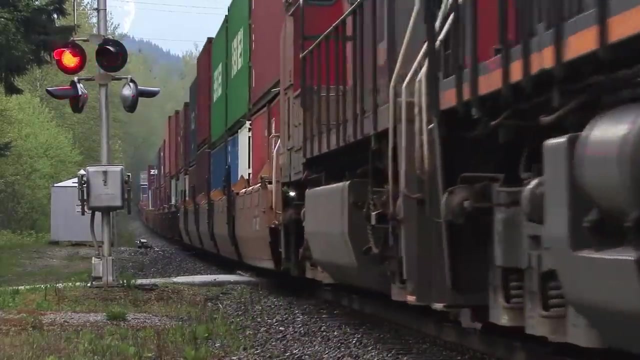 So it can be in the other behind it. Having a feeding pipe is such a great idea. Is it a train or is it a plane? It's a freight train. Let's have a look at this one. Do you think it's a train or a plane? 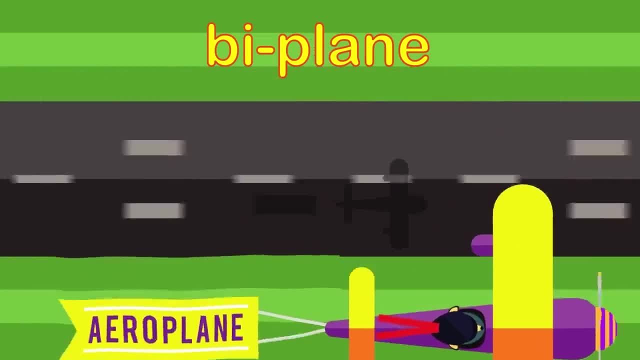 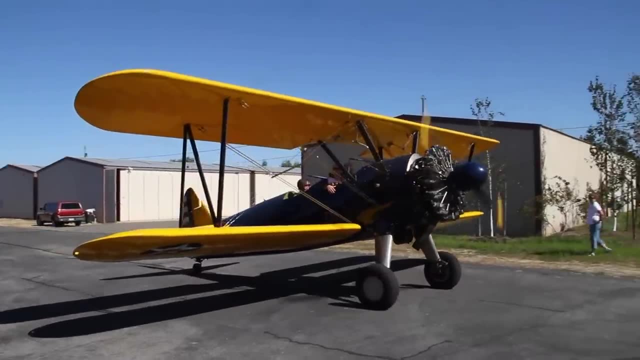 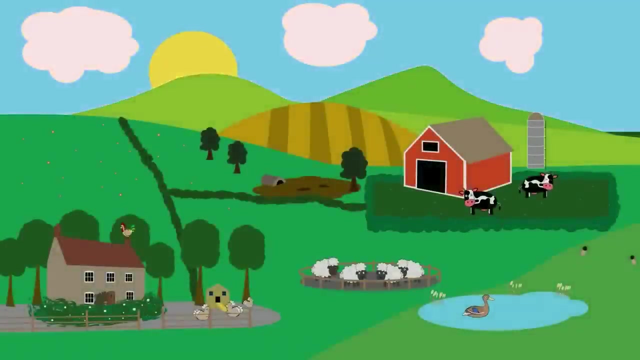 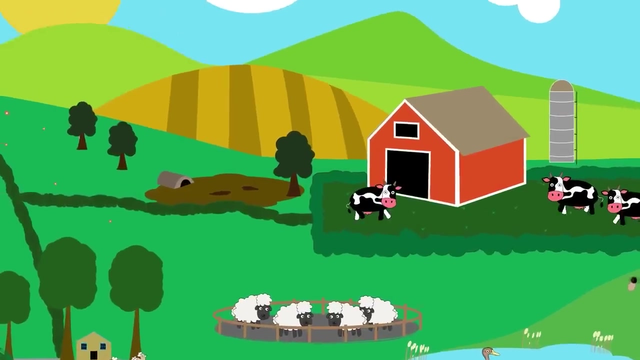 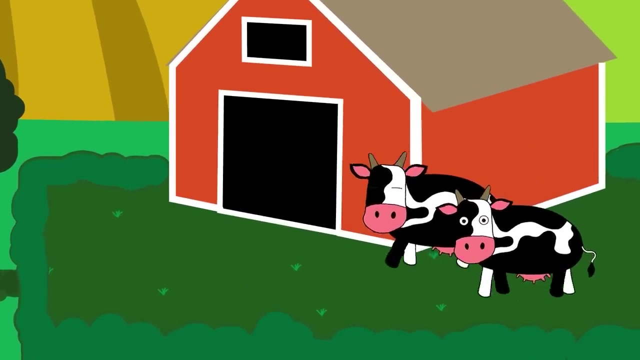 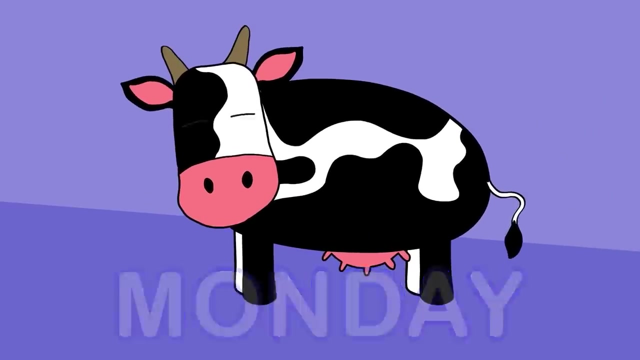 It's a biplane. Well done. I hope you enjoyed playing along. Hello and welcome back to Number Farm. Farms are very busy places. Shall we have a look at what happens during the whole week at Number Farm. Today is Monday and it's time for Farmer George to milk the cows. 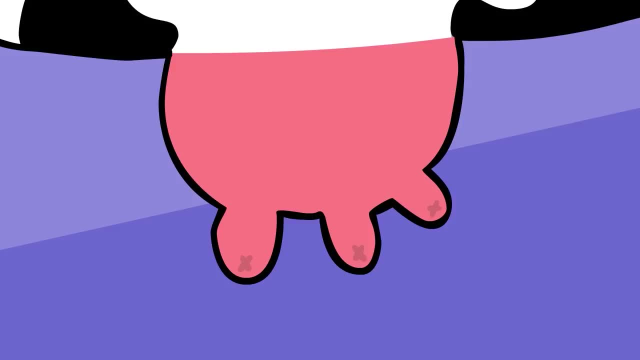 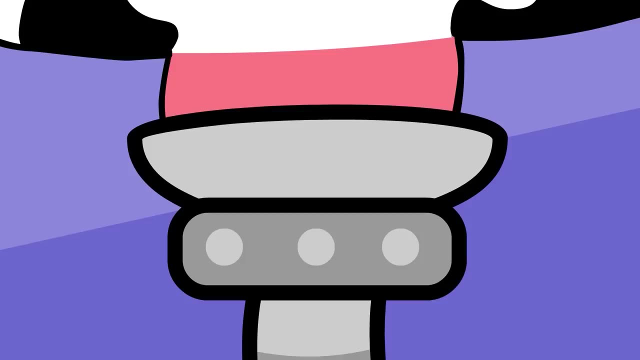 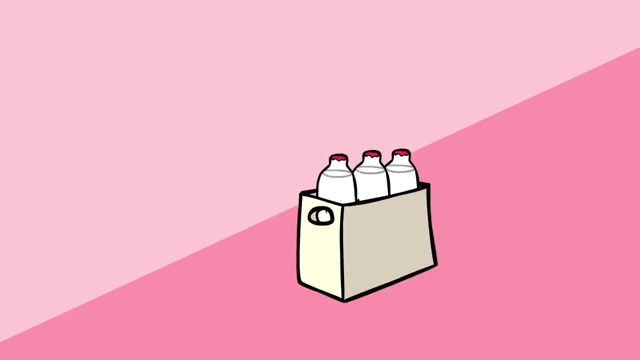 He has brought the cows into the milking parlour and connected his milking machines to the cows udders. The udders are where the milk comes from And all of the milk from the cows gets collected and bottled, ready to be put on your breakfast cereal. 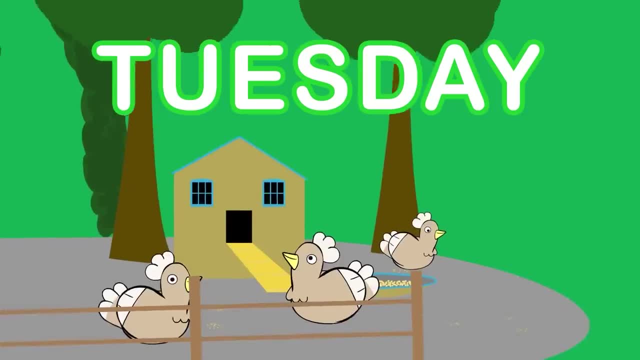 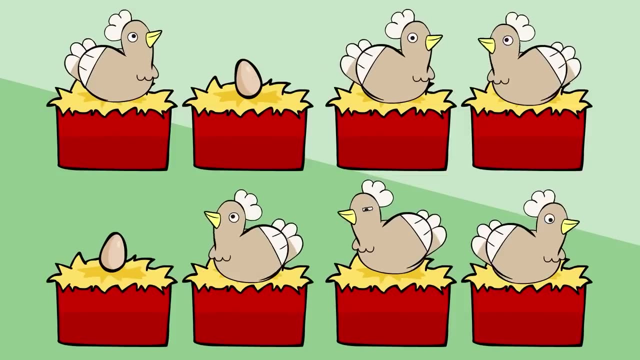 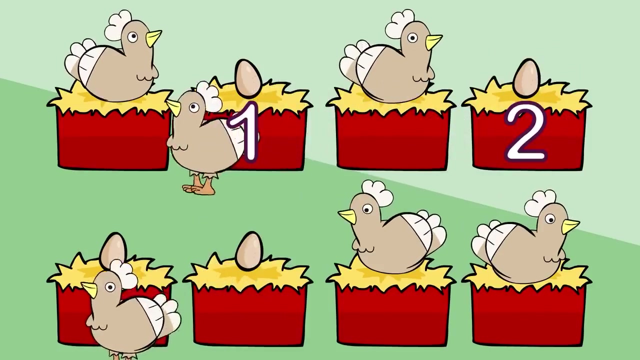 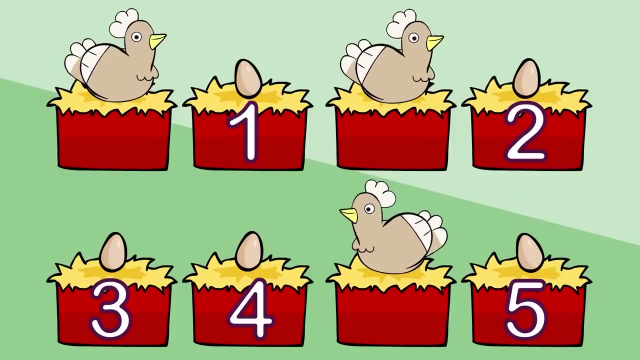 It's Tuesday today and it's time to collect the eggs from the hen house. Shall we count how many eggs the hens have laid in their nests? There's one, two, three, four, five. Now how shall we cook them? 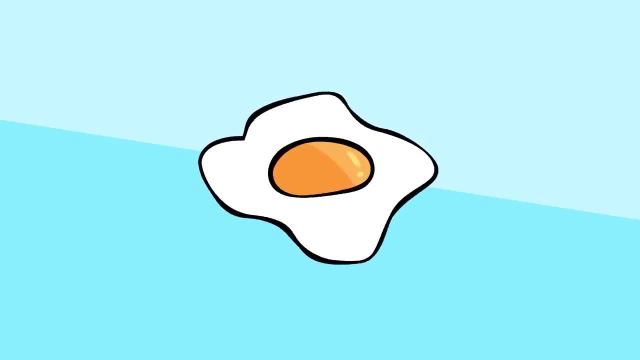 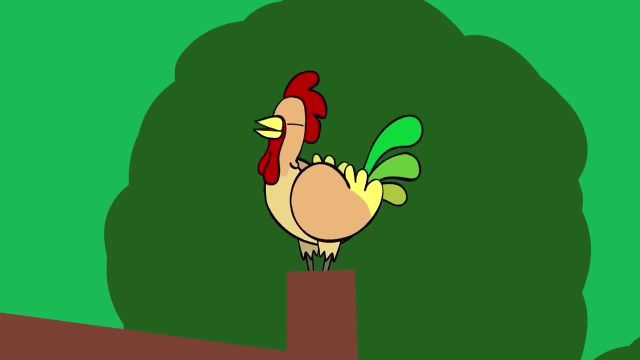 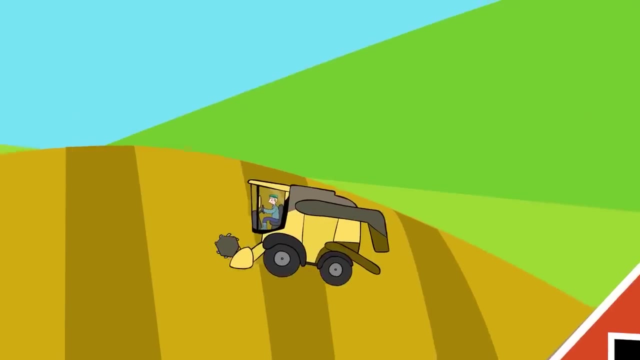 Boiled, scrambled, fried or poached- What's your favourite way to eat eggs? On Wednesday, Farmer George is out for a walk. Today, Farmer George is out driving his combine harvester. A combine harvester is a machine that harvests the crops that grow in the fields. 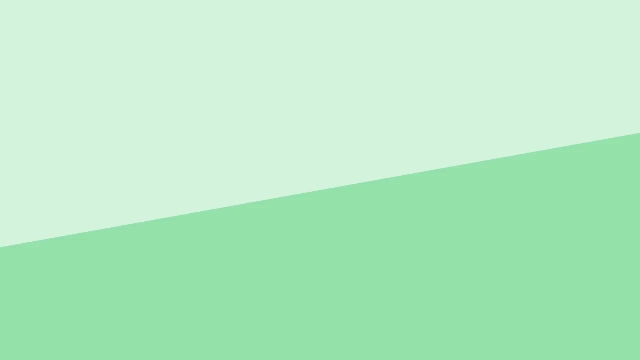 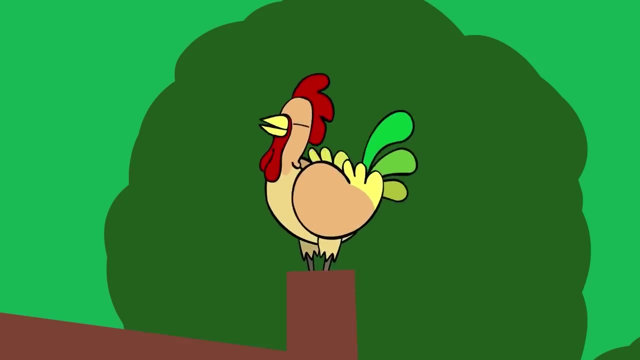 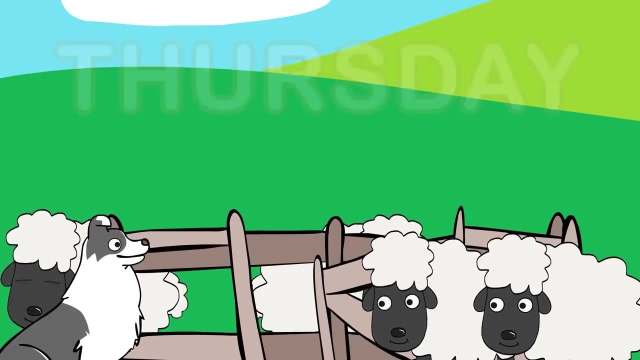 In this field, Farmer George has been growing wheat, which will then be used to make things like bread. Today is Thursday And Sammy the sheepdog is training for his sheepdog trials. That means he has to round up all of the sheep into the pen as quickly as possible. 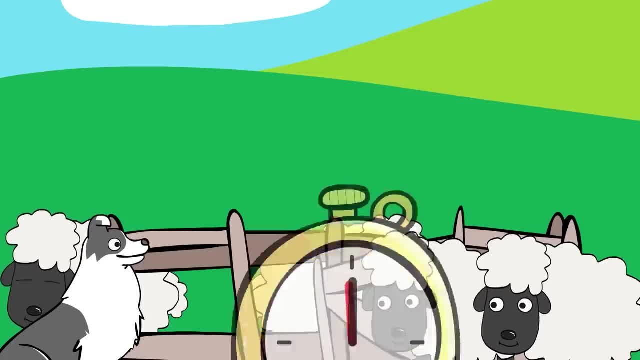 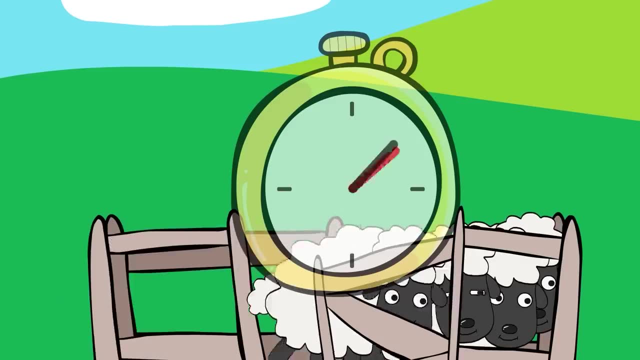 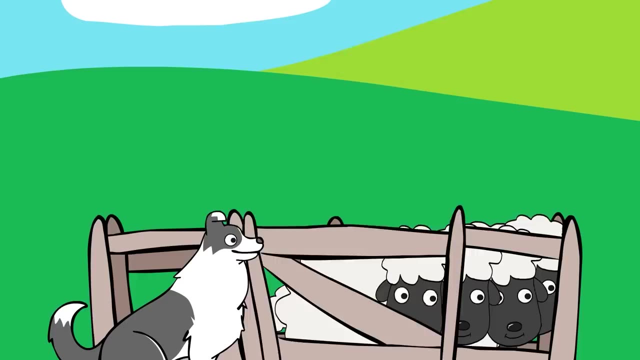 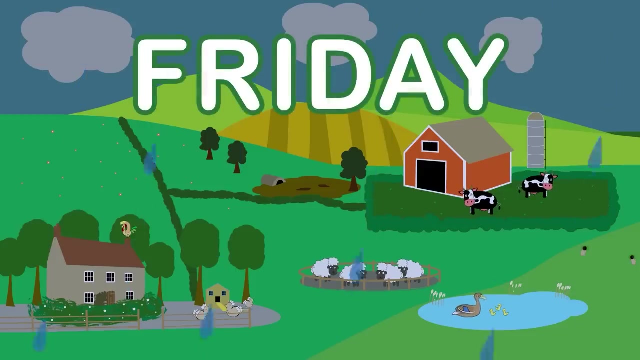 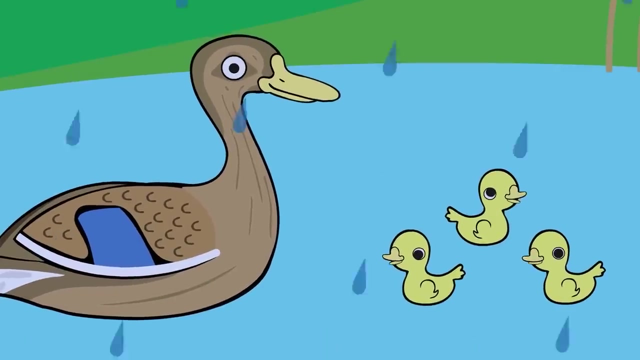 Ready, steady, go. Come on, Sammy, you can do it. Yay, Sammy, rounded up all the sheep in just 12 seconds. Friday is a very rainy day, but the ducks don't mind. Oh look, Mummy Duck has given birth to some beautiful ducklings. 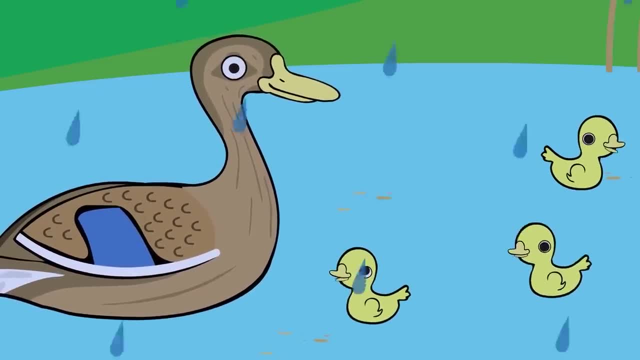 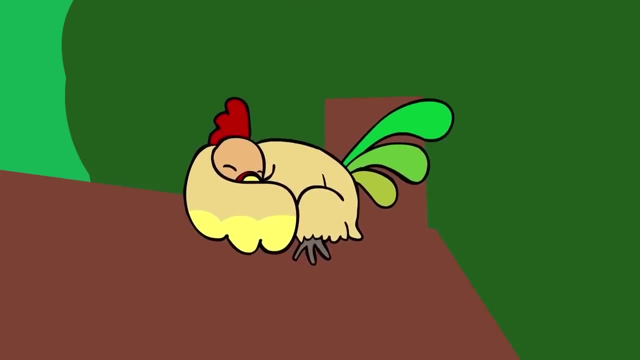 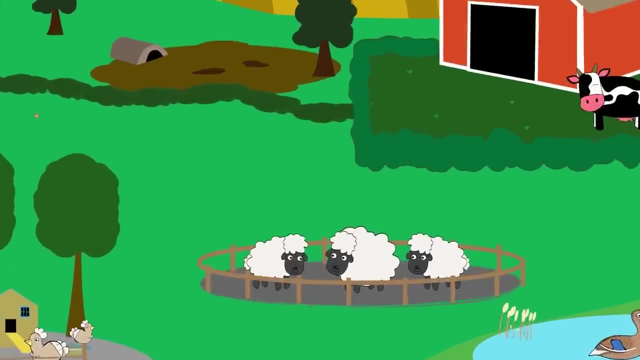 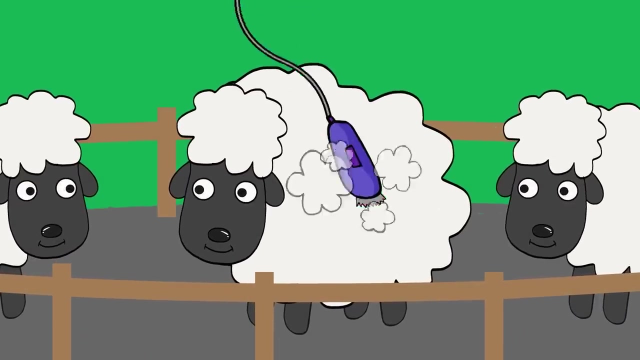 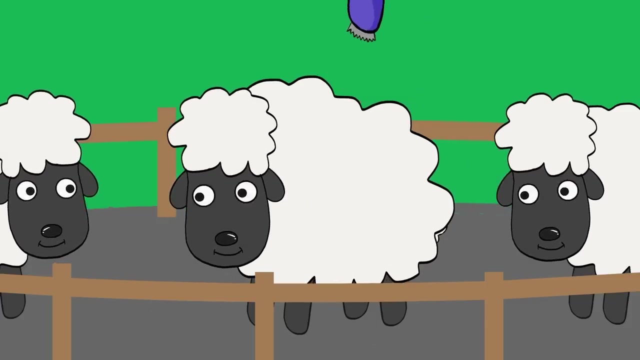 Let's feed them some bread. It's Saturday today, and that means it's the weekend, But work doesn't stop on the farm. It's a very hot day, so it's time to give the sheep a haircut Every few months. a sheep's coat will get too long, so the farmer will shear the sheep's coat with some clippers. 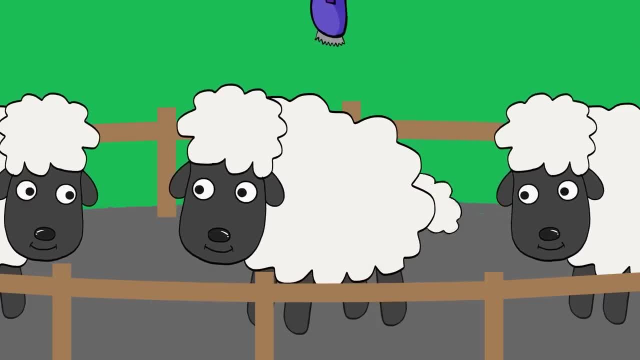 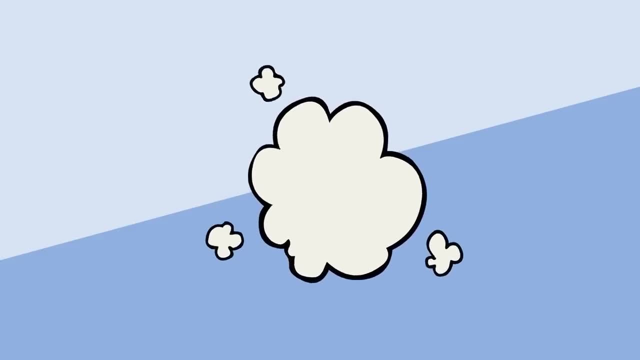 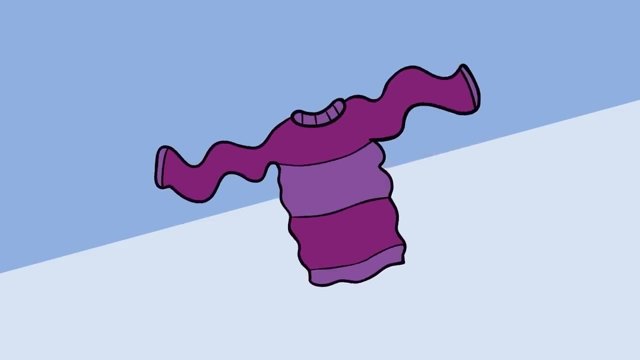 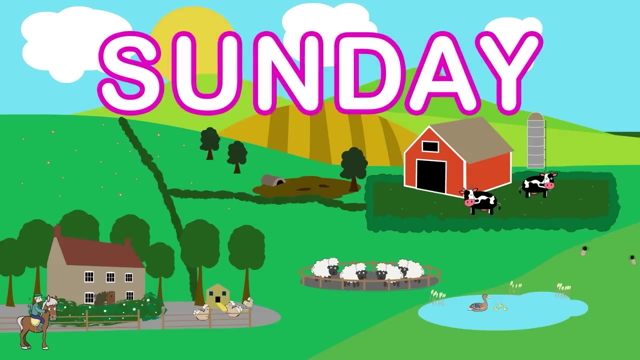 This is called sheep shearing and stops the sheep getting too hot in summer. The wool from the sheep's coat is used to make lovely woolly jumpers that keep us warm in the winter. It's Sunday, the last day of the week, so it's time for some fun. 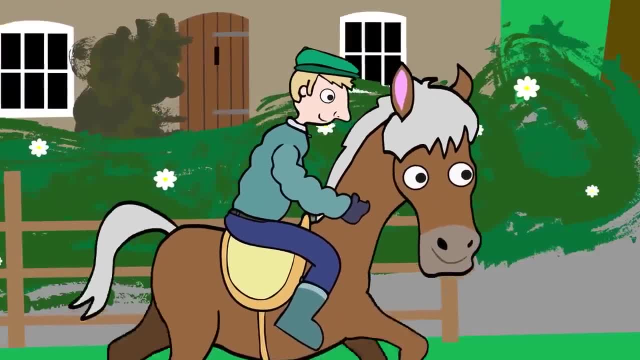 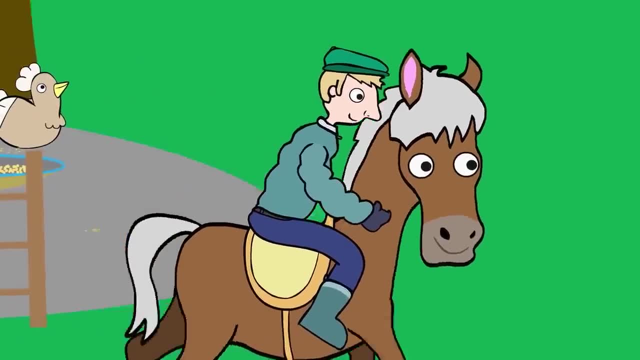 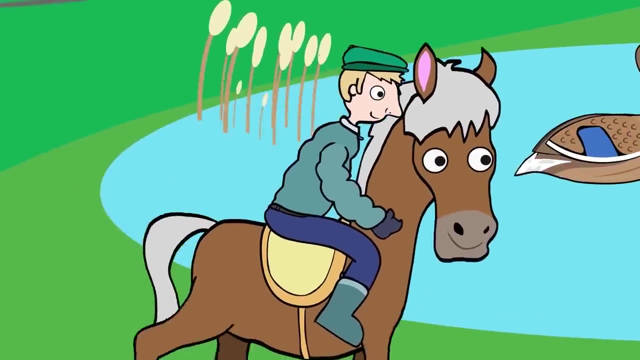 Whoopee Farmer George likes to ride his horses on Sundays, And Harry the horse loves galloping as quickly as he possibly can. Wow, look at him. go Hold on tight, Farmer George, you don't want to fall off. 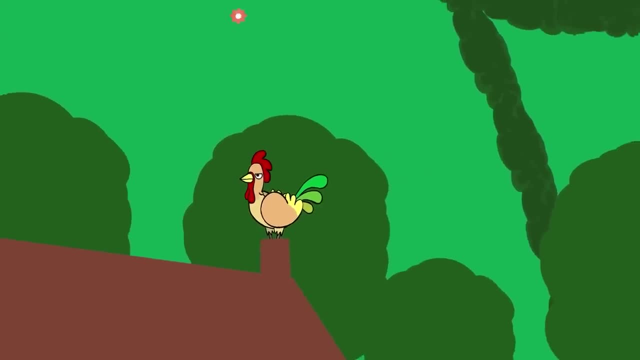 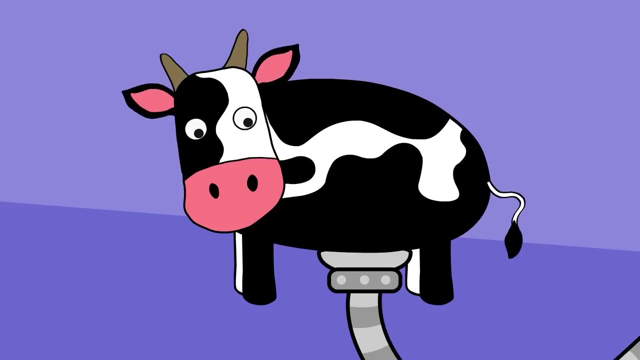 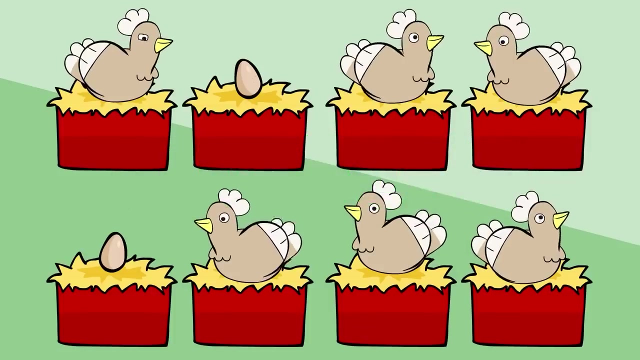 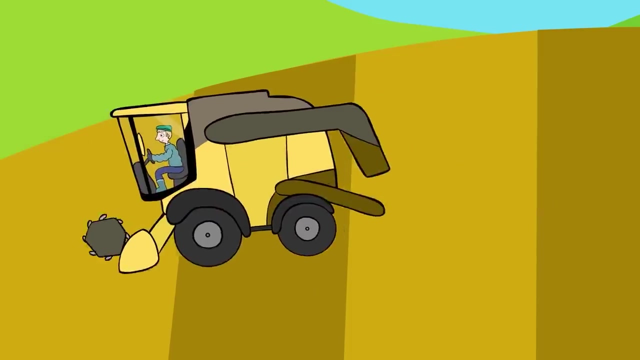 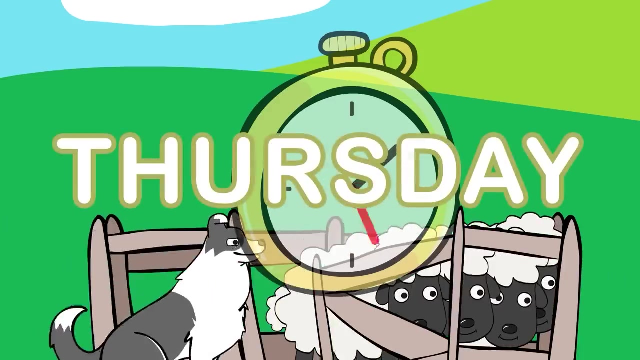 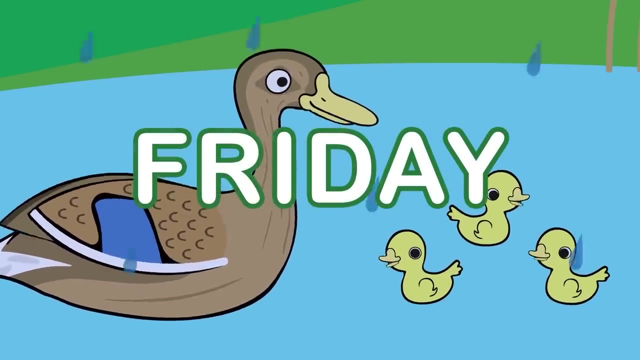 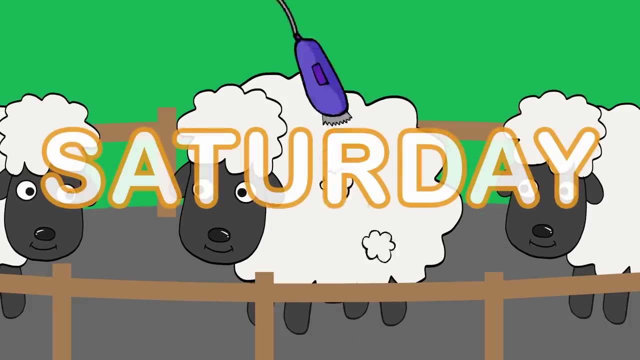 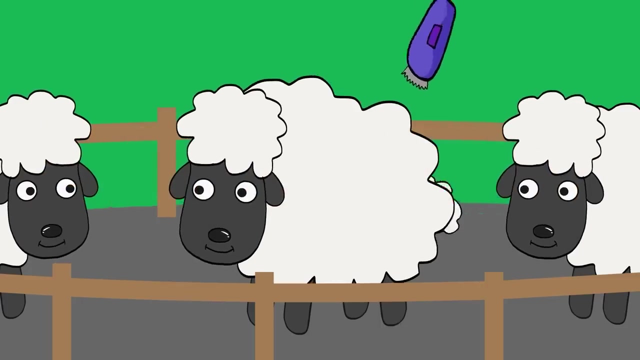 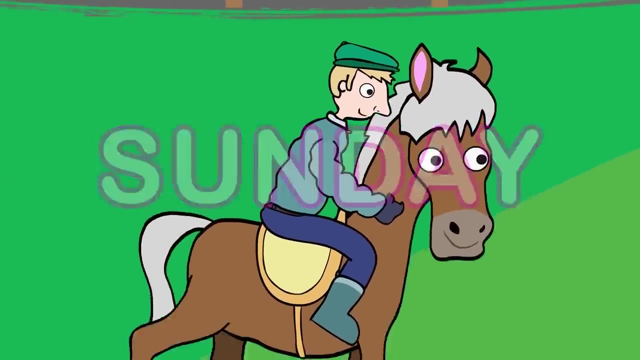 Can you remember the days of the week? No, Oh, On Monday, Monday, Friday, Friday- sheep Friday was a rainy day and we fed the ducks. Saturday was a very hot day, so it was sheep shearing day, And on Sunday, Farmer George went riding on Harry the horse. 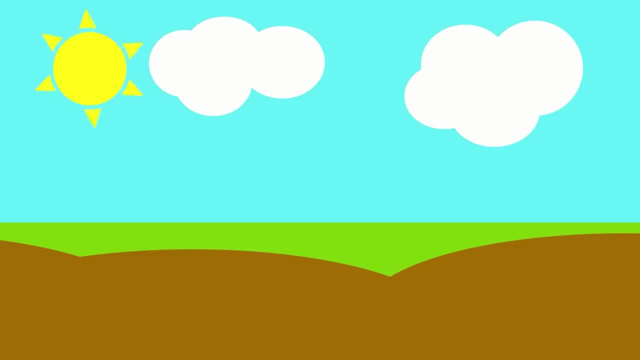 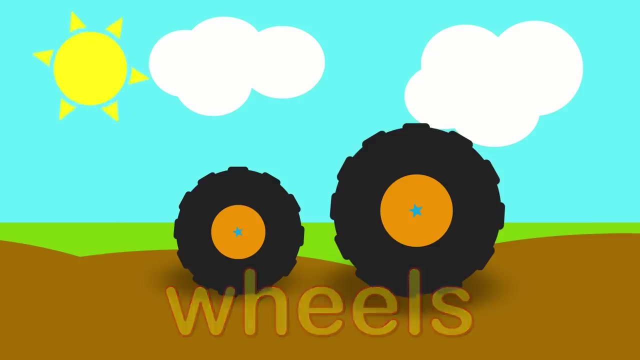 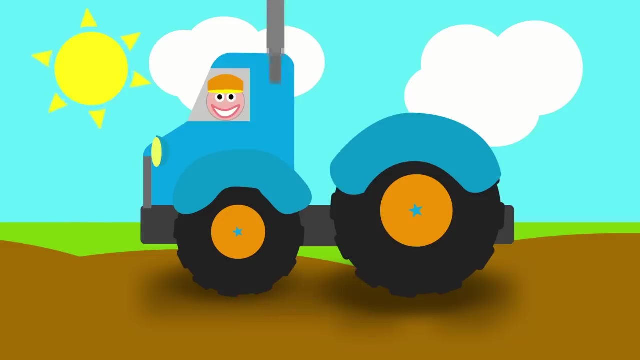 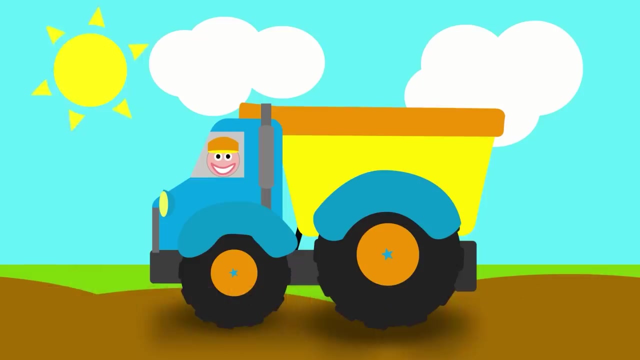 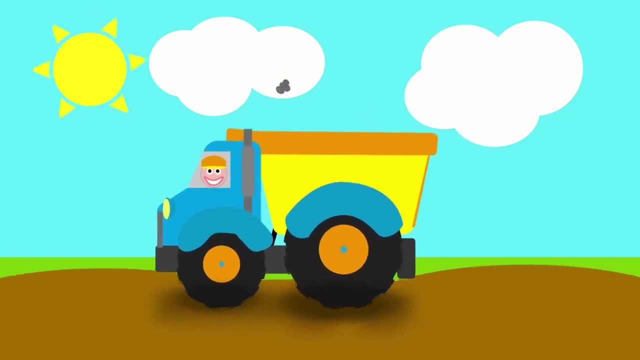 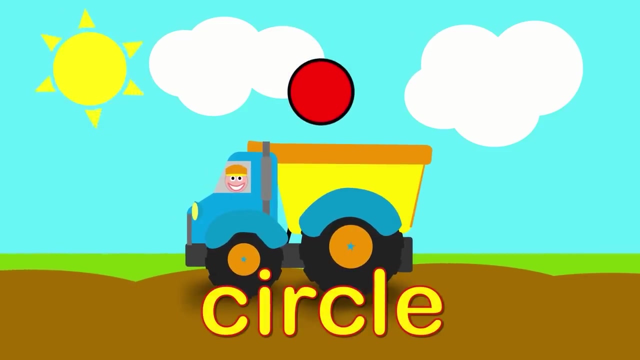 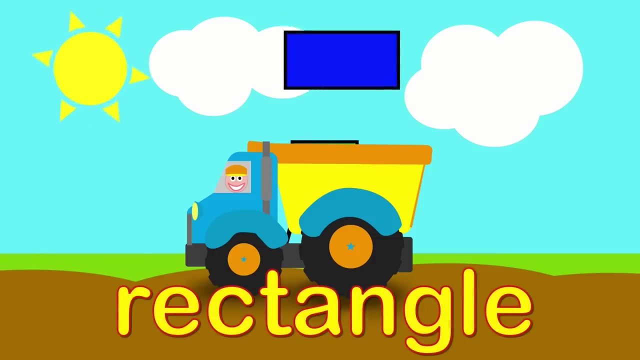 Let's build a dump truck: Wheels, Chassis, Cab, Exhaust, Rear bumper, Hydraulic ram, Dumping bed, Back gate. Let's load some shapes into our dump truck: Circle Square Dump truck, Rectangle Star, Hexagon. 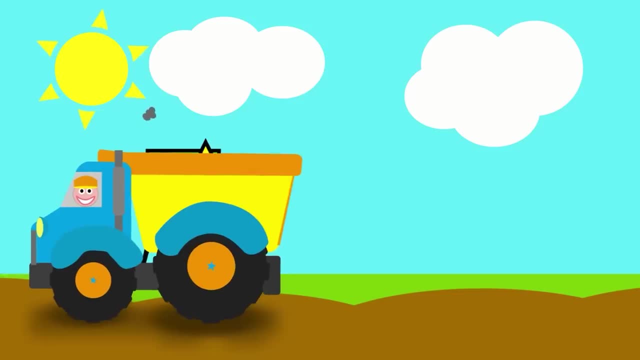 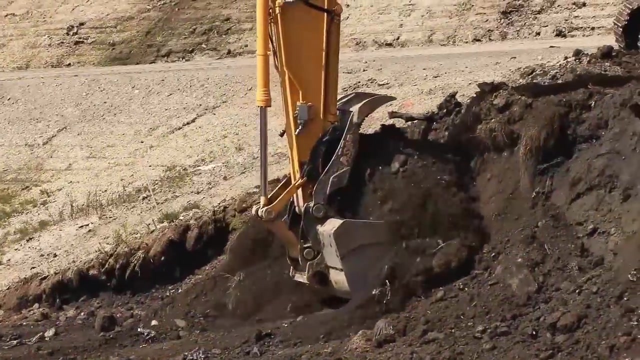 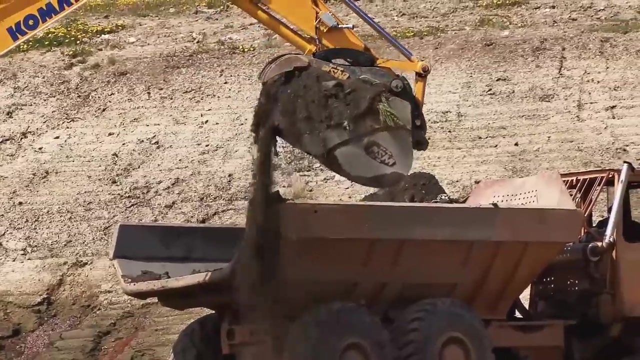 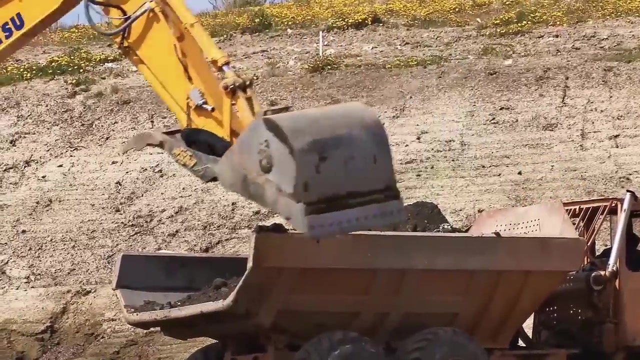 Now let's tip them out again. Circle Square: Rectangle Star Hexagon ощ. Circle Square. Circle Dumping. Rectangle bar Circle- Vigorous Dumping. Circle Circle- Vigorous Dumping. 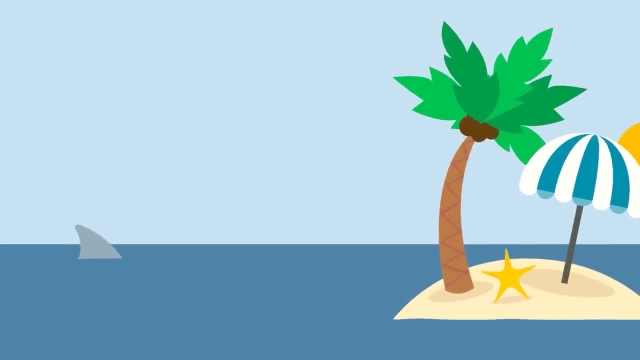 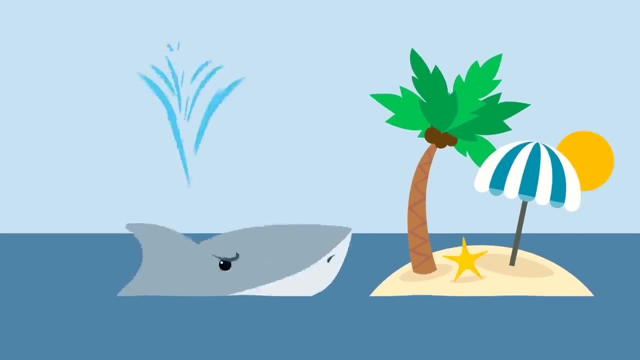 Square, Hexagon, Star Circle, Curve Circle- It almost looks just like a fin. Oh, Mr Shark, don't scare me, so It isn't funny. No, no, no, We need to count your teeth. 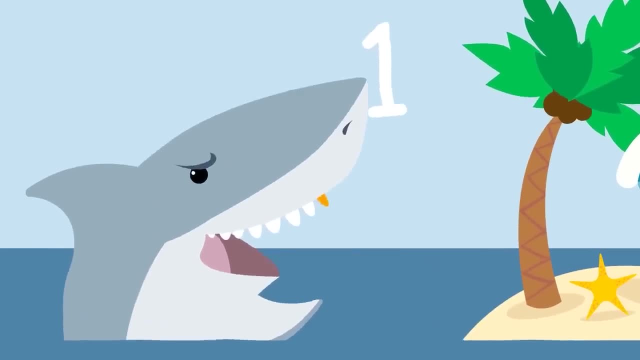 OK, One, Two, Three. Now please go away. What We need to count at least one more. Very well then, Three plus one makes four. Oh, what a cheeky cheeky shark. Always snap, snap, snapping. 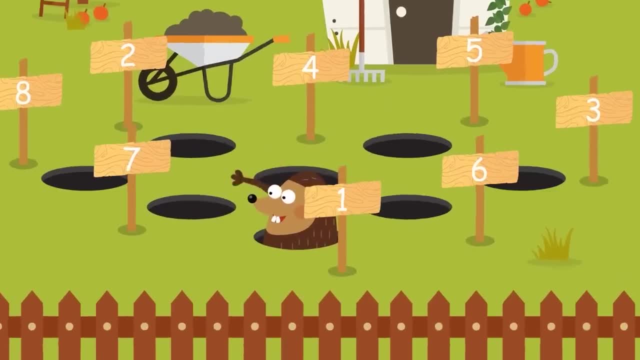 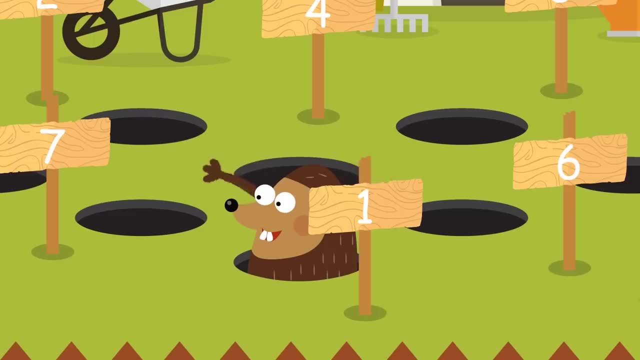 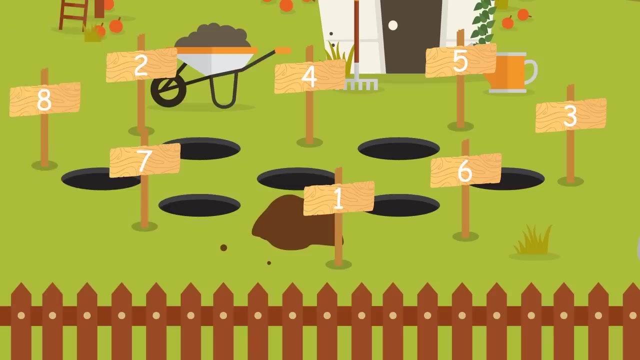 Hello there, Mr Messy Mole, Have you alone dug all these holes? It's quite a lot of mess you've made. Oh look, Here comes the gardener's spade. He's filling up holes one and two. Now three and four have been filled up too. 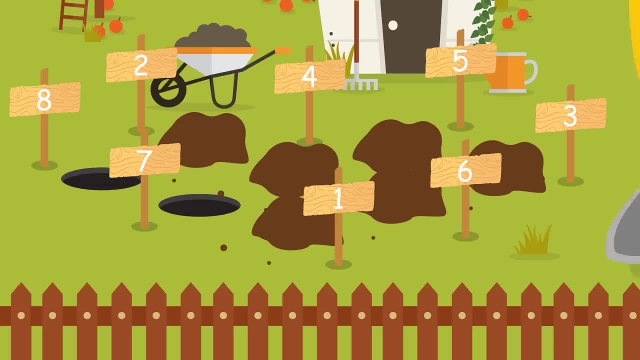 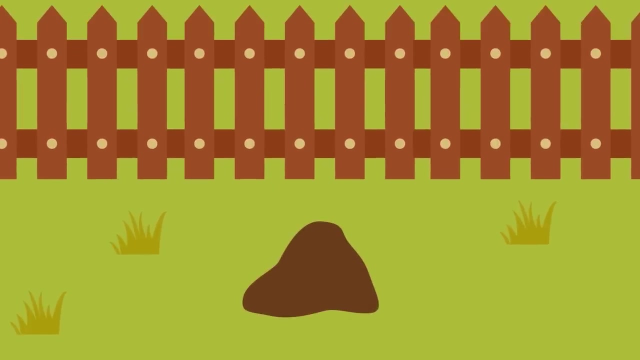 Five and six. He's nearly done. Now seven holes. That leaves just one. Oh no, He's filled up number eight. But look Who's that up by the gate. Hooray, It's Mr Mole. He's just not going to stop dig, dig, digging holes. 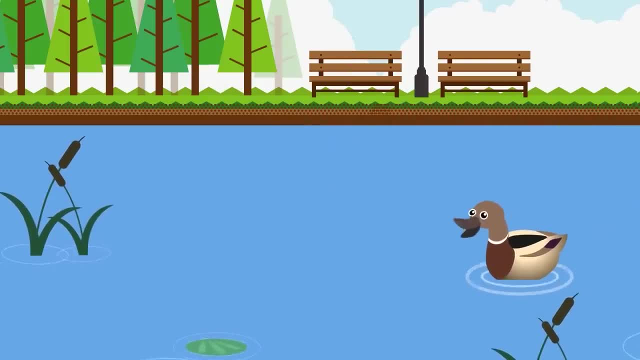 Sweet mummy, duck out on the lake. That's such a lot of noise to make. You're trying to call your babies back. Well, let us help you. Quack, quack, quack, Here they come. One, two, three, four. 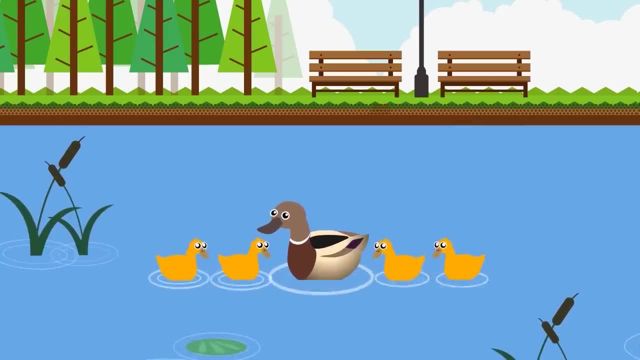 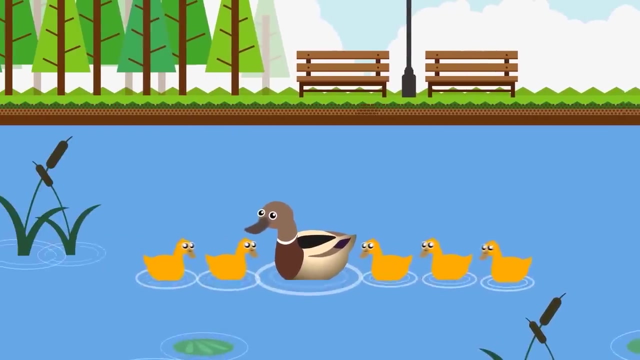 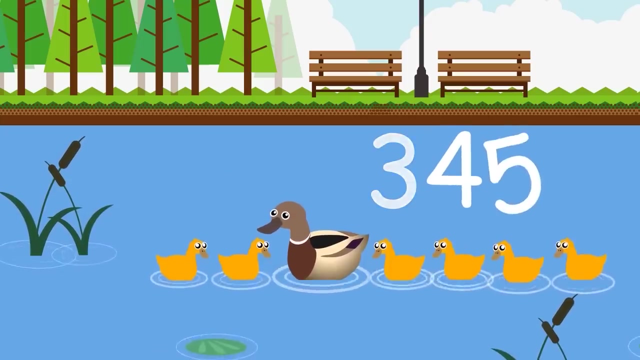 Was that it, Or are there more? You have six ducklings all in all. That means we've one, two, two more ducks to call. Here they are Just by those sticks. Now we've got all One, two, three, four, five, six. 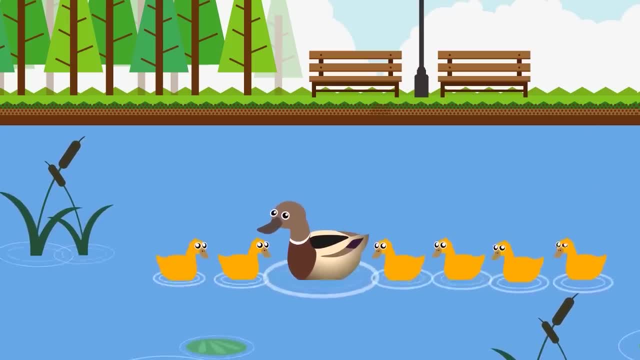 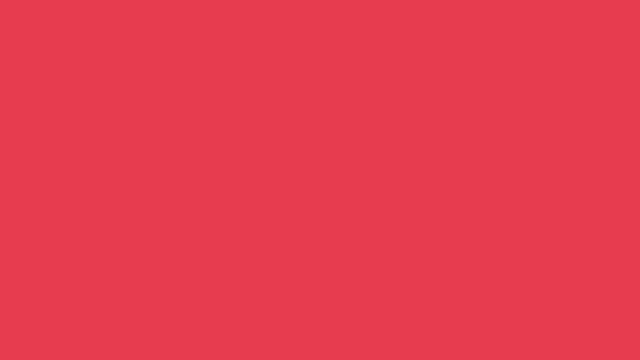 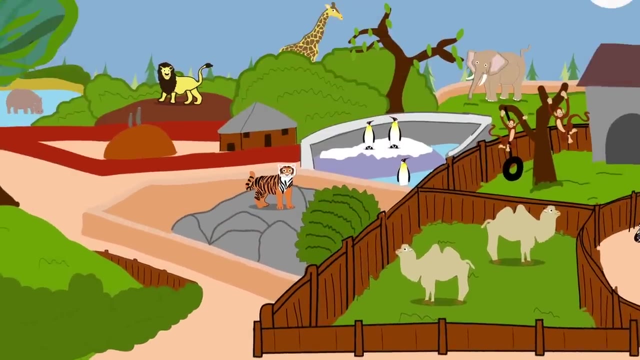 Yay, Hooray. Now you've helped the babies find their mum. Welcome back to Number Zoo. Our zookeepers have been busy creating some new homes for all of our new animals. Let's meet the animals and check that they've settled in. 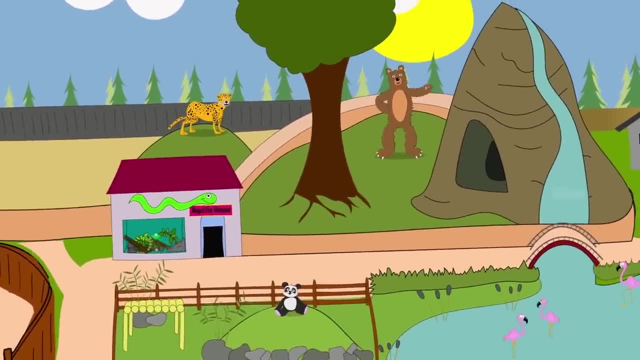 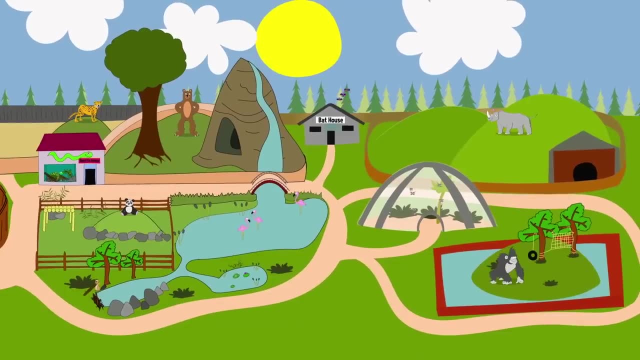 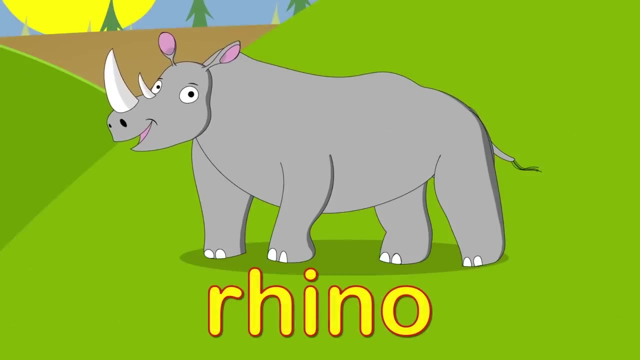 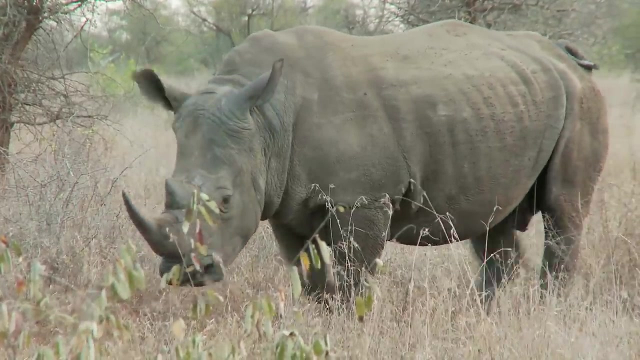 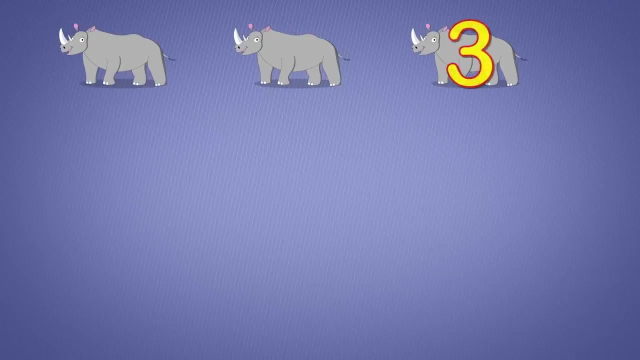 It's time to do some counting with our new friends. Is everybody ready to count to twenty this time? Yes, Hello, Wrinkly Rhino, How are you today? One, two, three, four, five, six, seven, eight, nine, ten. 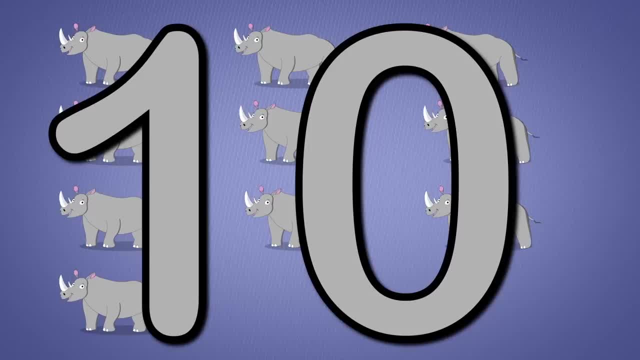 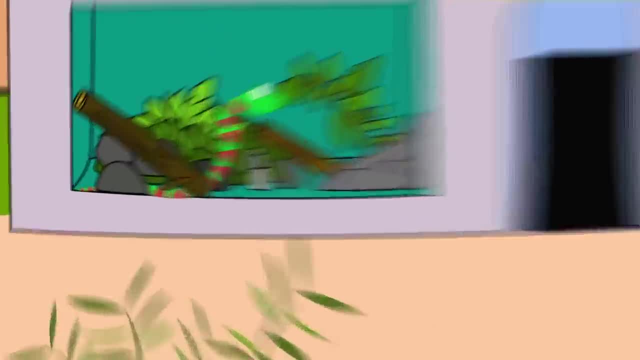 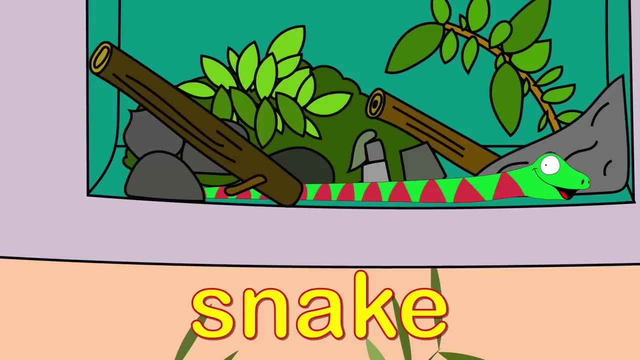 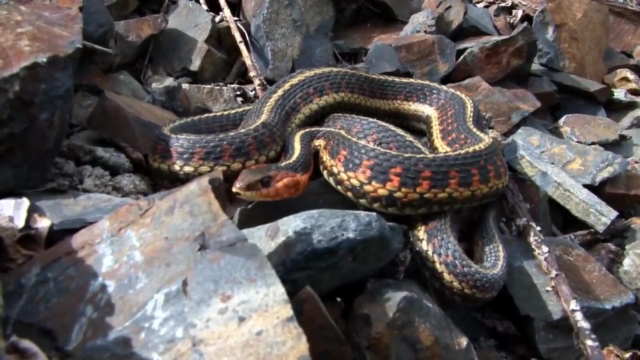 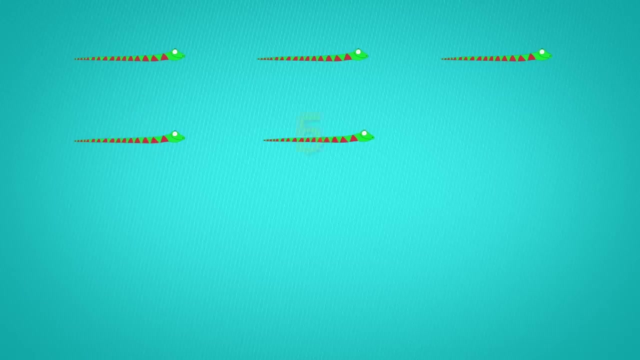 Ten Rhinos. Ooh, hello, Slithery Snake. I hope you like your new home. I hope you like your new home One, two, three, four, five, six, seven, eight, nine, ten, eleven. 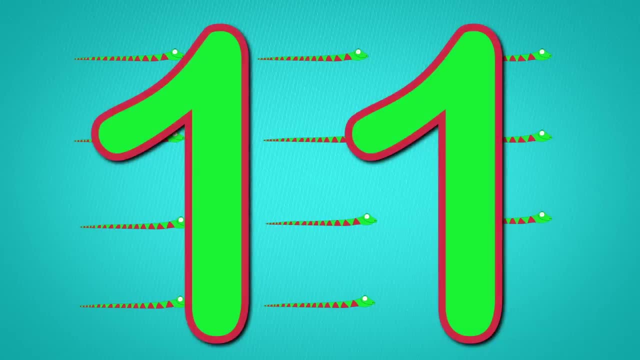 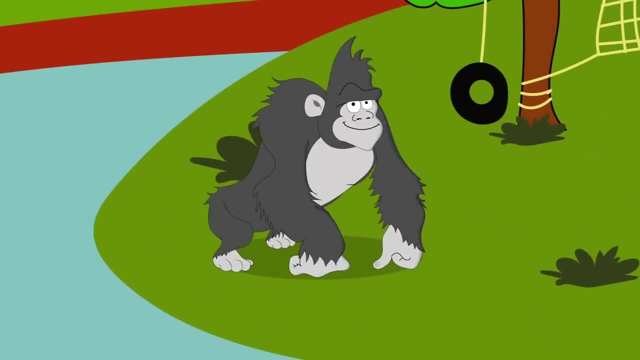 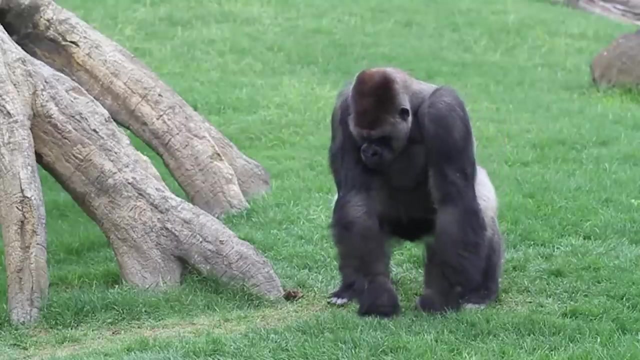 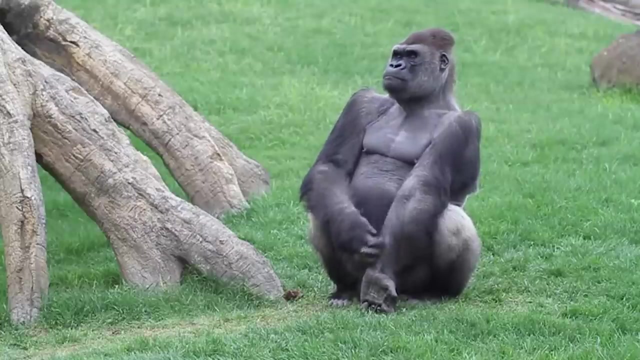 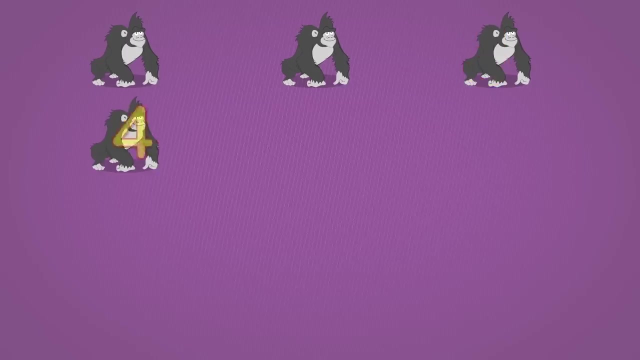 Eleven, snakes. Well, hello, Mr Gorilla. One, two, three, four, five, six, seven, eight, nine, ten, 1,, 2,, 3,, 4,, 5,, 6,, 7,, 8,, 9,, 10,, 11,, 12. 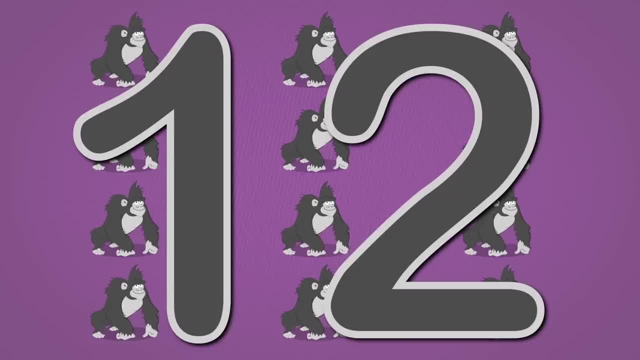 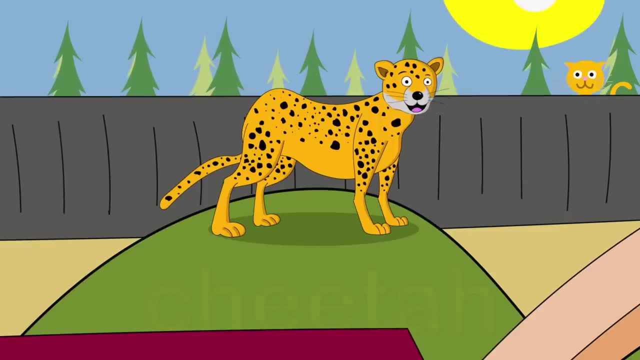 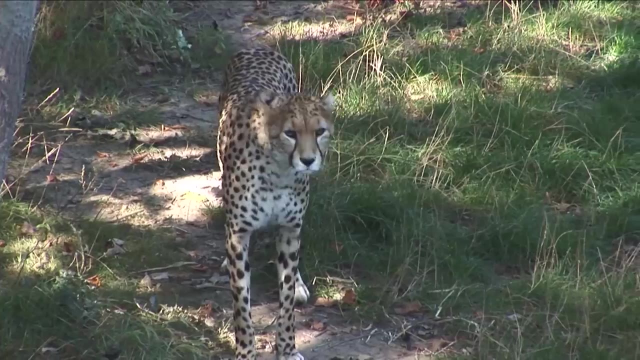 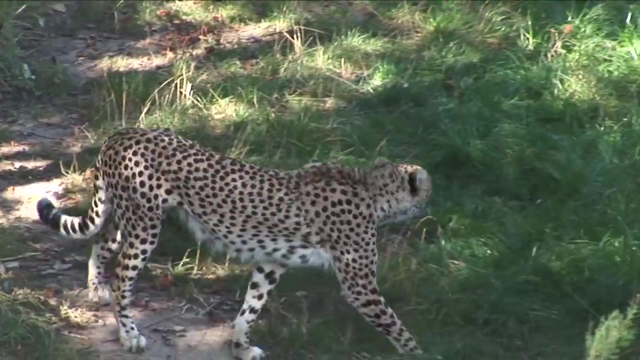 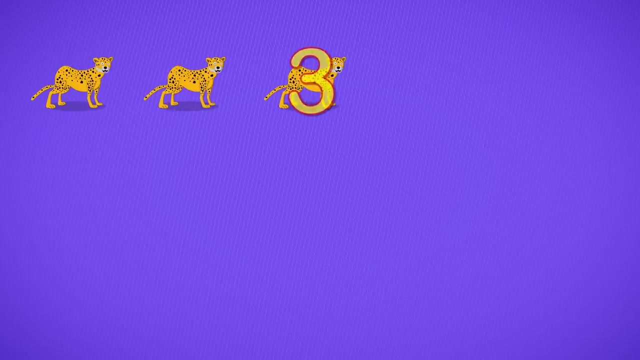 12 gorillas. Who's next? Oh, speedy cheetah, I love your spotty fur. 1,, 2,, 3, 4,, 5,, 6,, 7,, 8,, 9, 10. 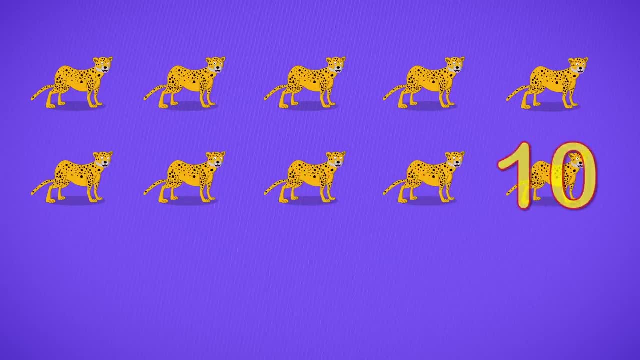 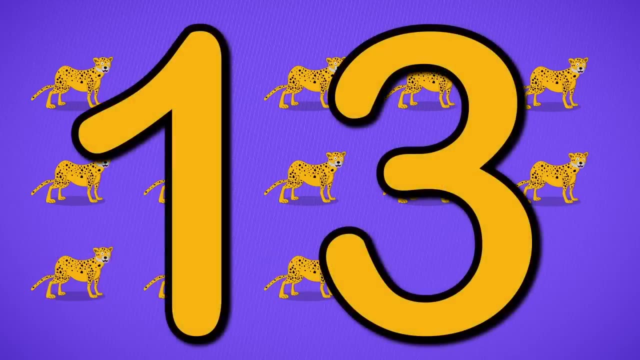 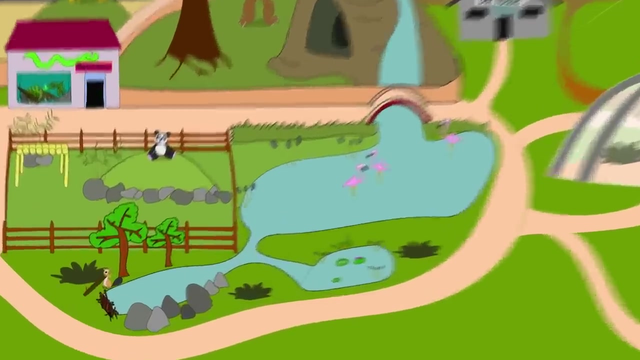 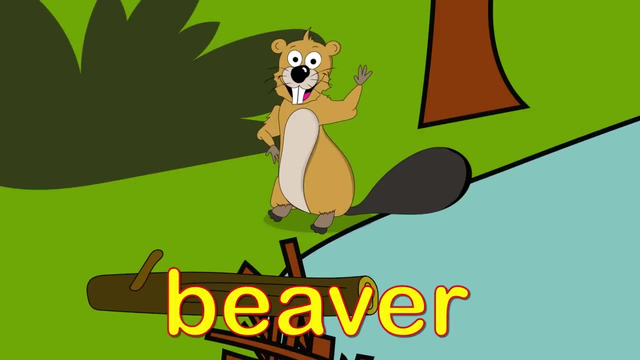 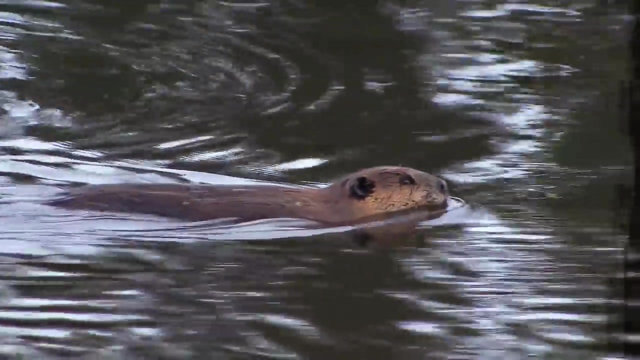 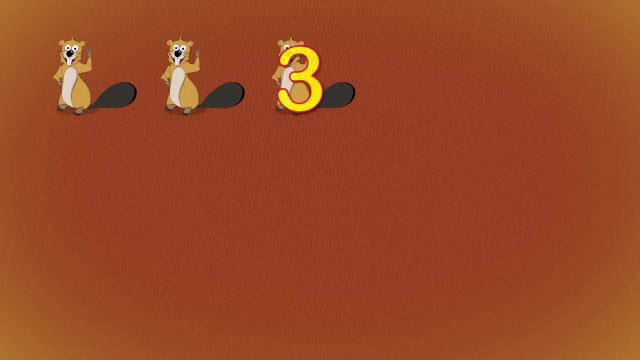 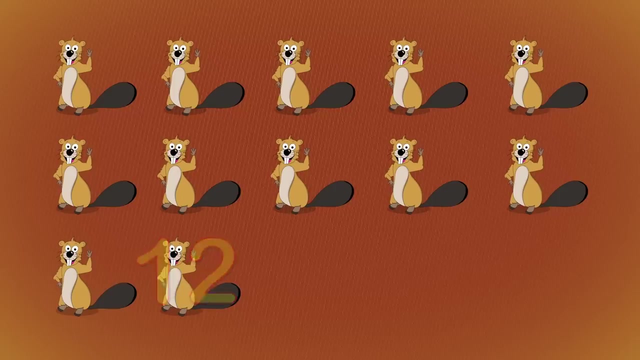 11,, 12,, 13,, 13 cheetahs. Hello, happy beaver. Look at your big teeth. Are you building a dam? 1,, 2,, 3,, 4,, 5,, 6,, 7,, 8,, 9,, 10,, 11,, 12,, 13,, 14. 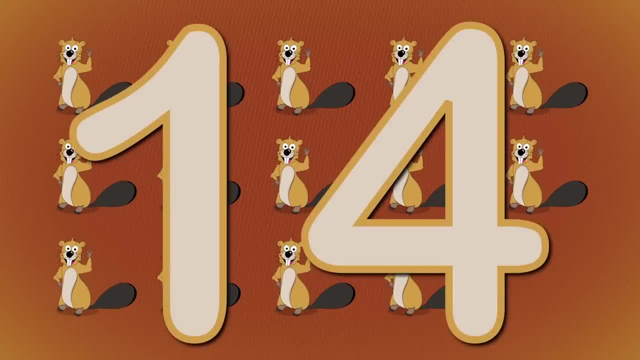 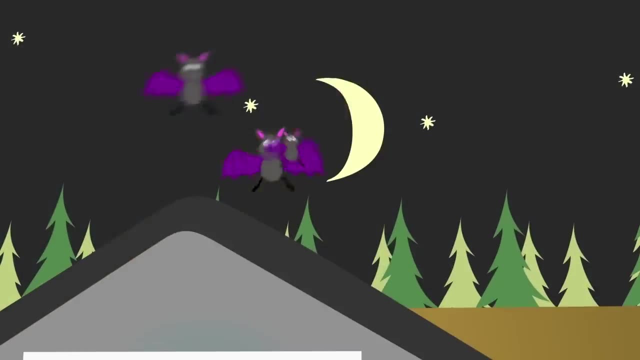 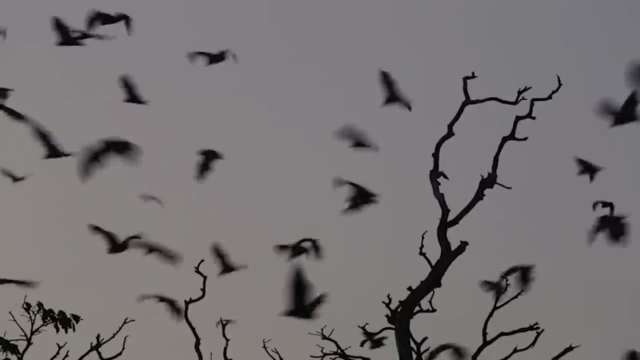 14 beavers. Hello, flappy bats. When it gets dark, the bats come out to play. 1, 2, 3, 4,, 5, 6,, 7,, 8, 9,, 10,, 11,, 12,, 13, 14. 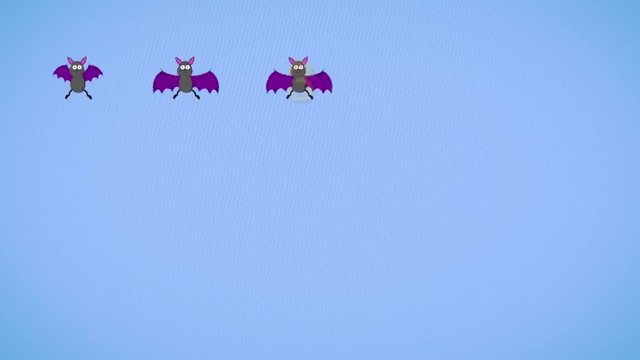 1,, 2,, 3,, 4,, 5,, 6,, 7,, 8,, 9,, 10,, 11,, 12,, 13,, 14, 15 beavers. Good afternoon, cuddly panda. are you enjoying the sunshine? 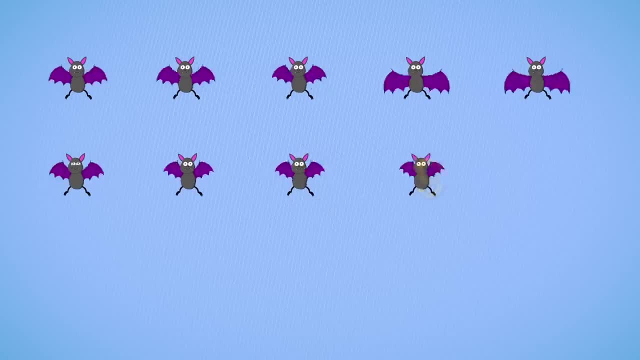 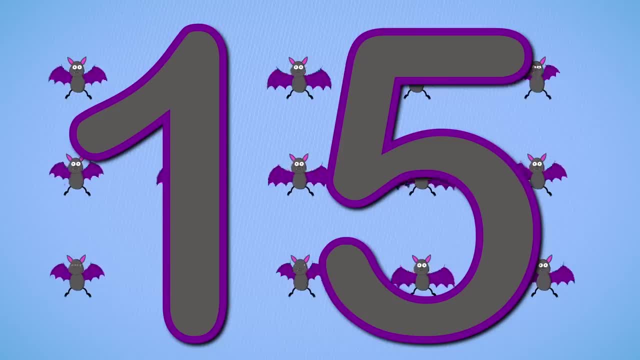 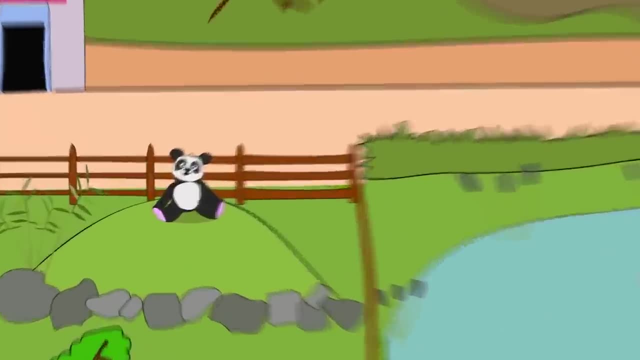 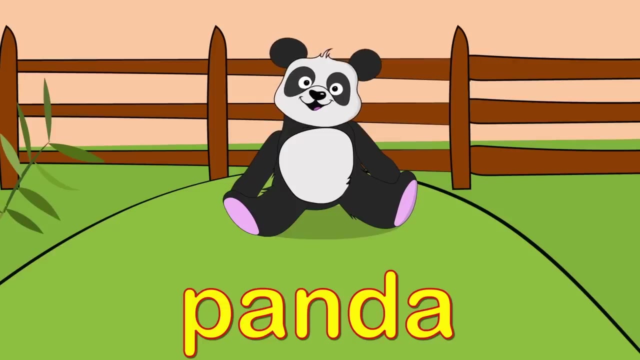 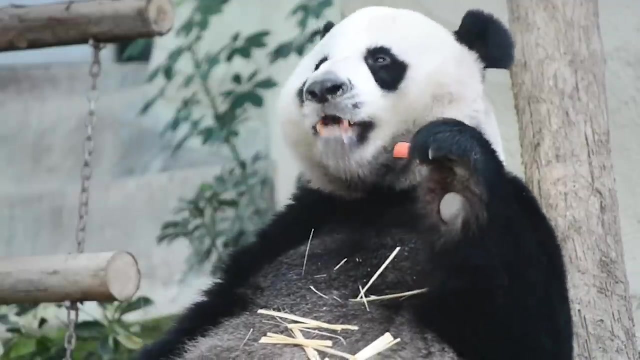 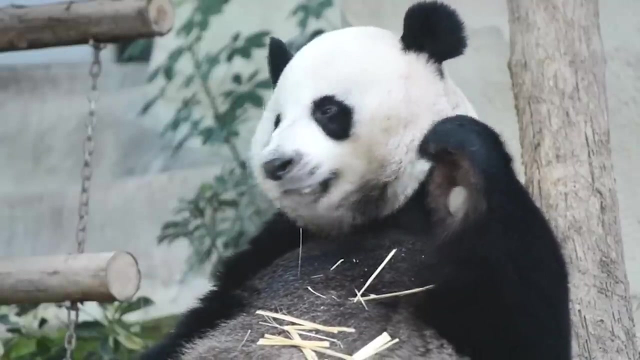 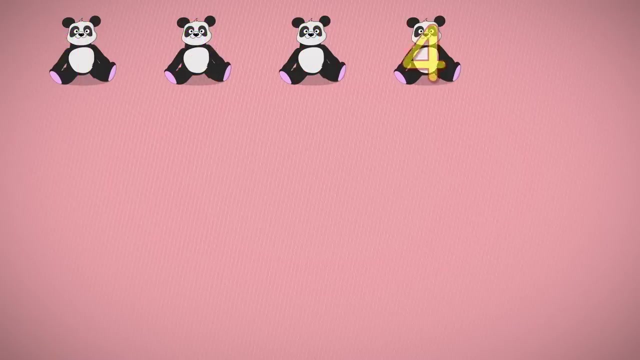 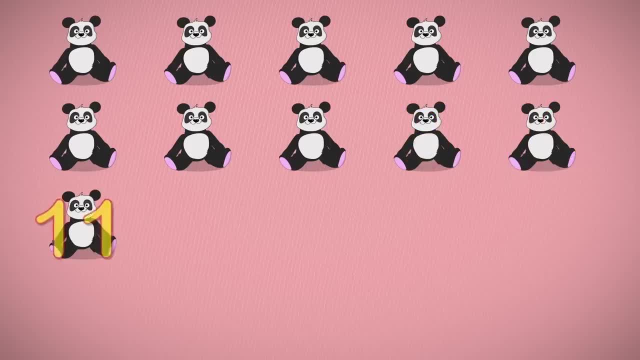 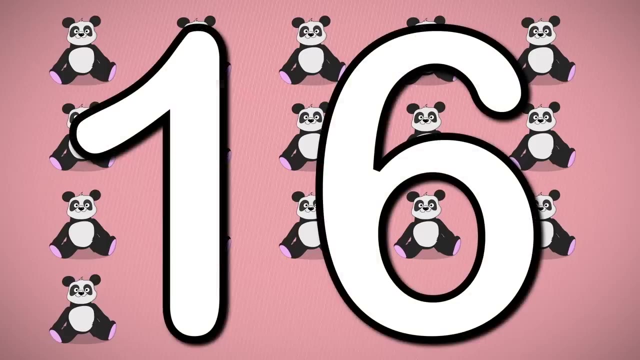 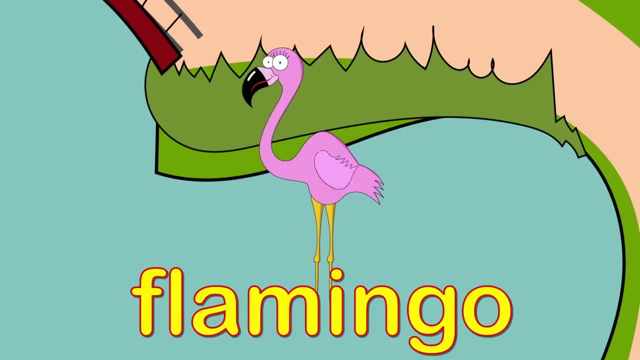 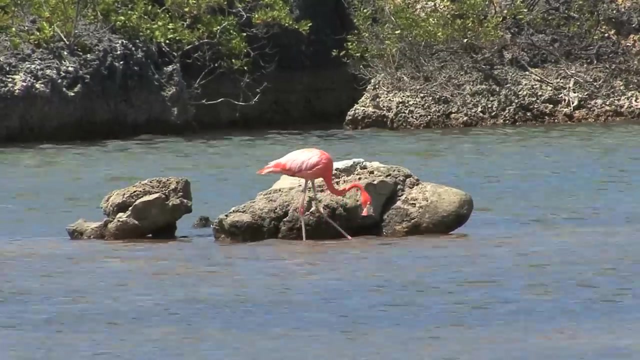 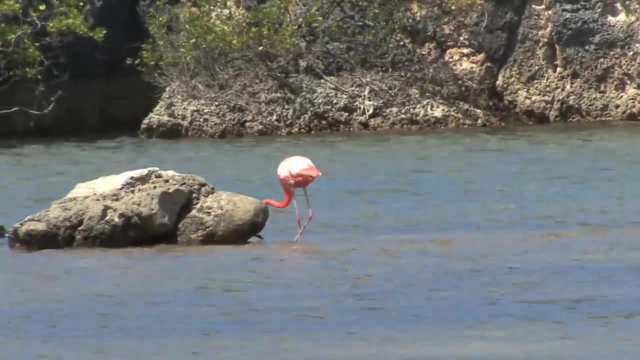 9,, 10,, 11,, 12,, 13,, 14,, 15, 16.. 16 pandas: Hello, pretty flamingo, I love your pink feathers. 1,, 2,, 3,, 4,, 5,, 6,, 7,, 8,, 9,, 10,, 11,, 12,, 13,, 14,, 15,, 16.. 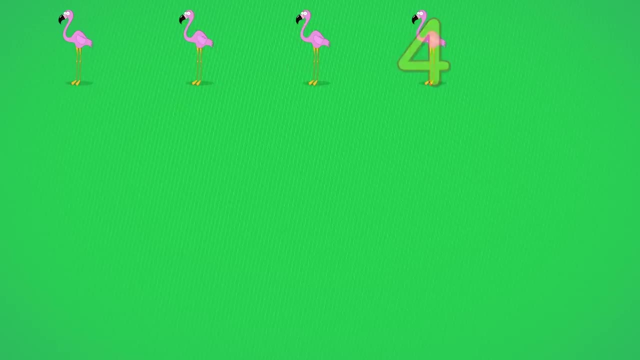 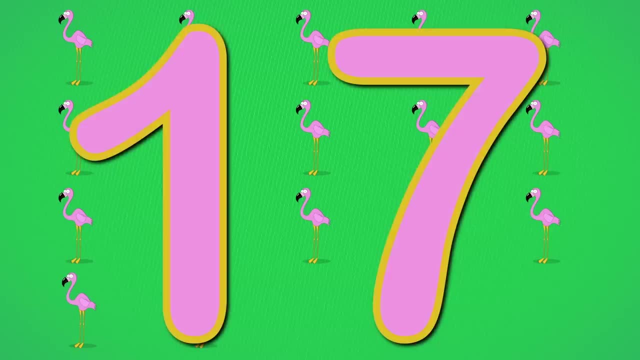 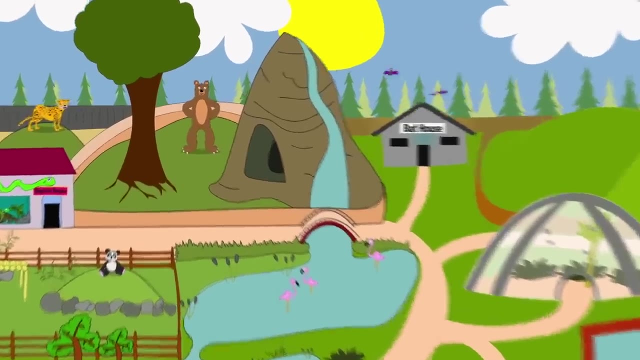 14,, 15,, 16,, 17,, 17,, 14,, 16,, 17,, 18,, 19,, 10,, 21,, 21,, 22,, 23,, 24,, 25,, 26,, 27,. 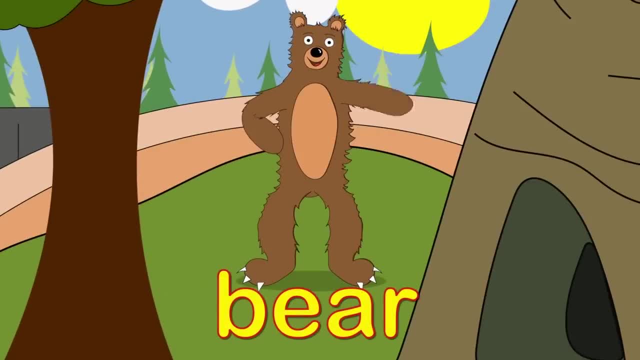 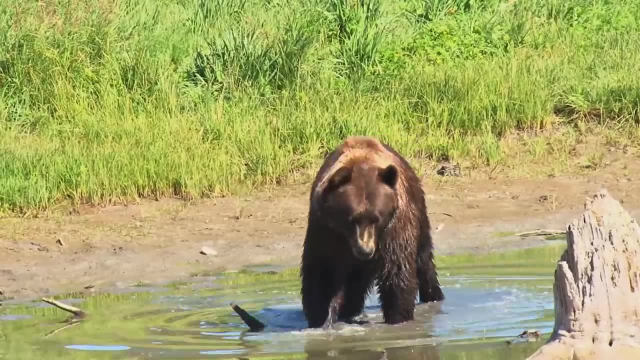 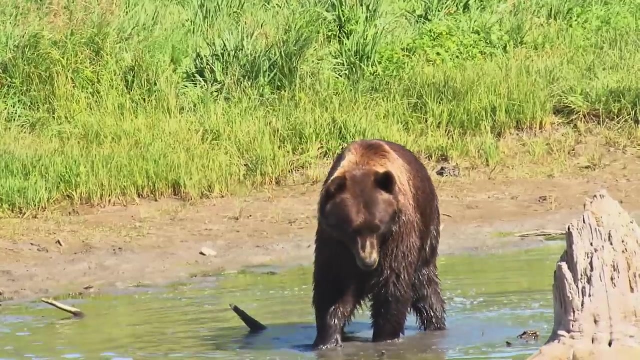 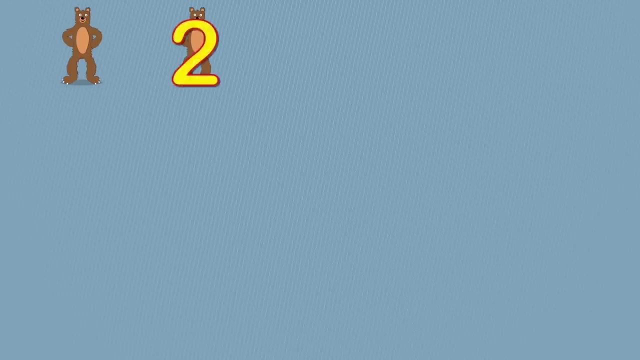 28,, 30,, 31,, 32,, 33,, OK, a hundred of them- This is the last star- One, two, three, four, five, six, seven, eight, nine, ten, eleven, twelve, thirteen, fourteen. 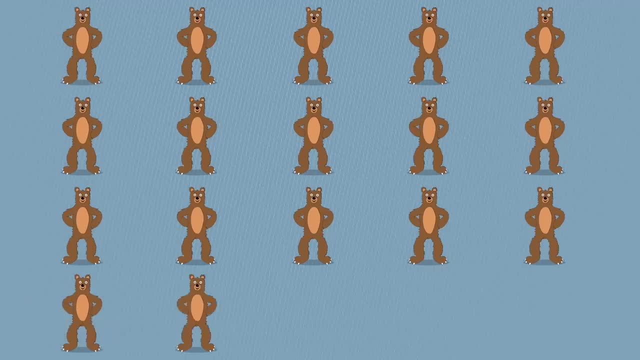 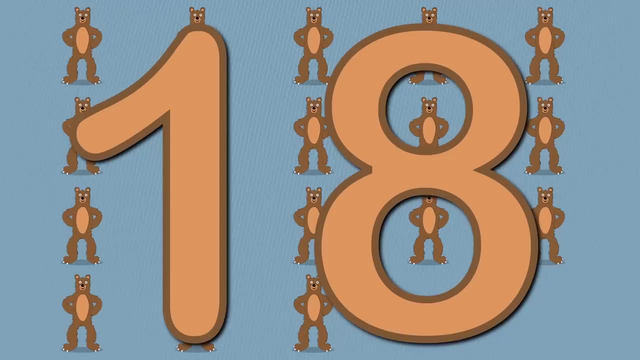 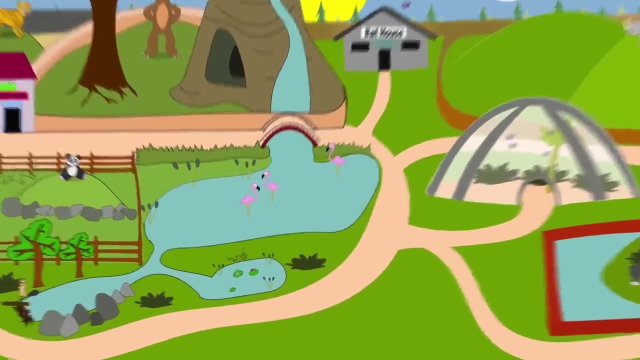 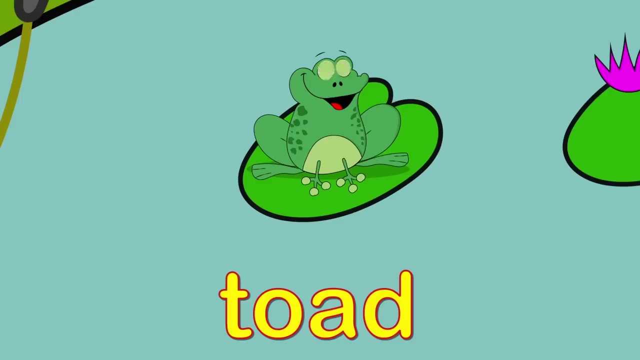 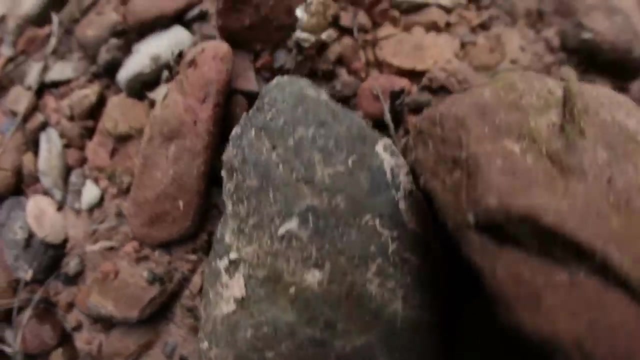 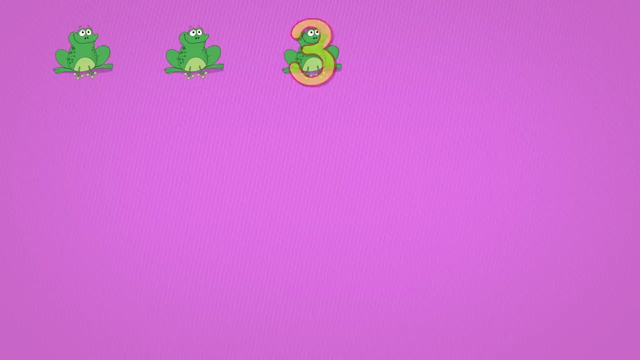 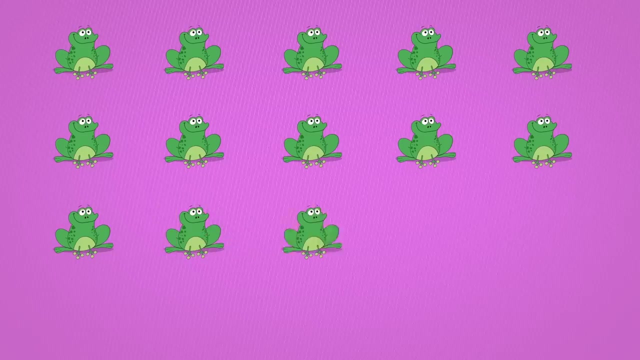 fifteen, sixteen, seventeen, eighteen, Eighteen brown bears. Hello Toad, Is that a yummy fly. One, two, three, four, five, six, seven, eight, nine, ten, eleven, twelve, thirteen, fourteen, fifteen, sixteen, seventeen, eighteen, nineteen, twenty. 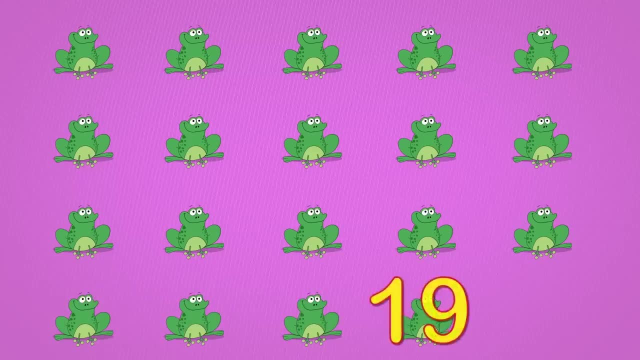 One, two, three, four, five, six, seven, eight, nine, ten, eleven, twelve, thirteen, eighteen, nineteen, Nineteen toads. There is only one more new animal to visit. What could it be? 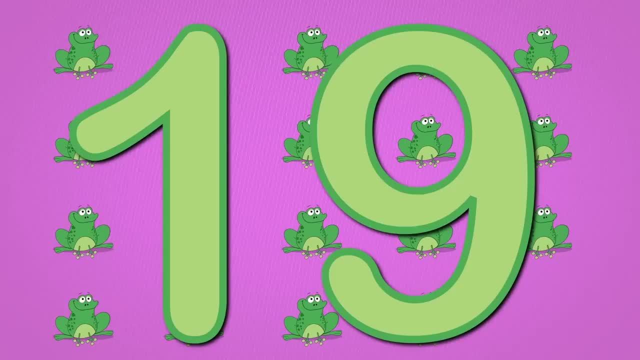 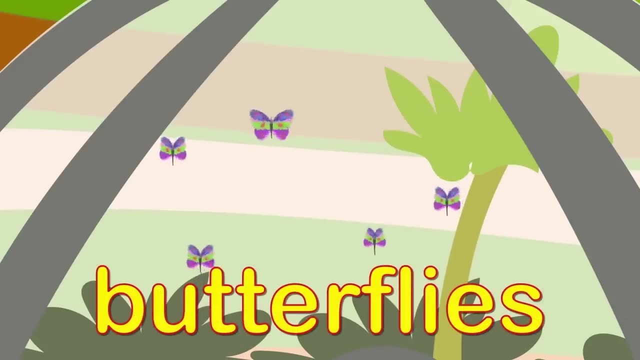 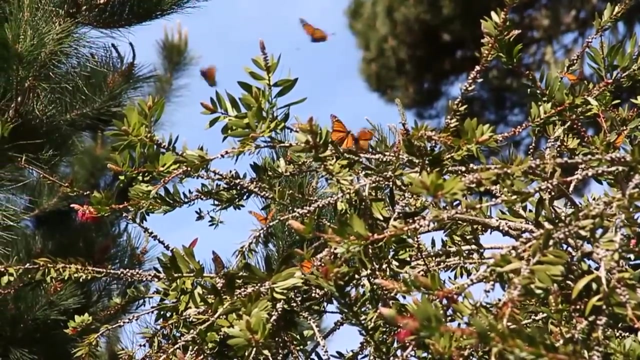 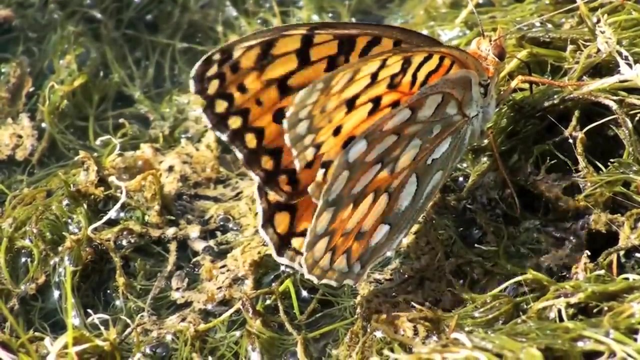 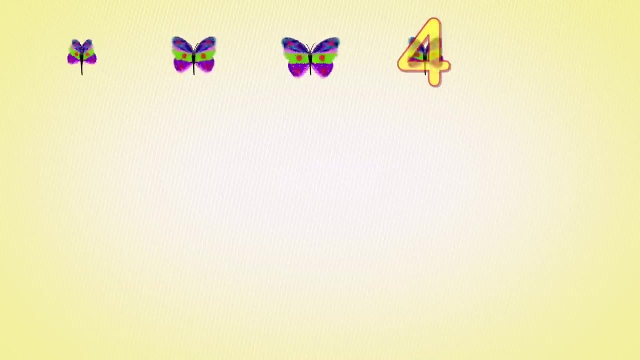 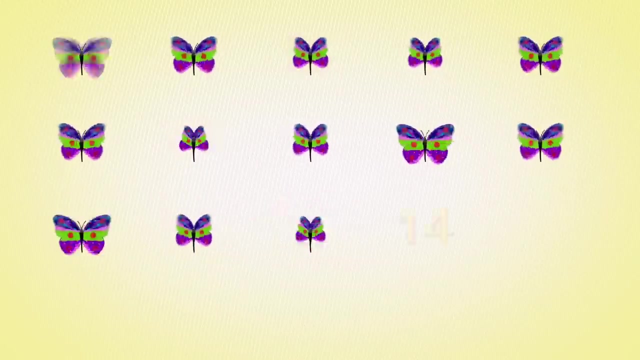 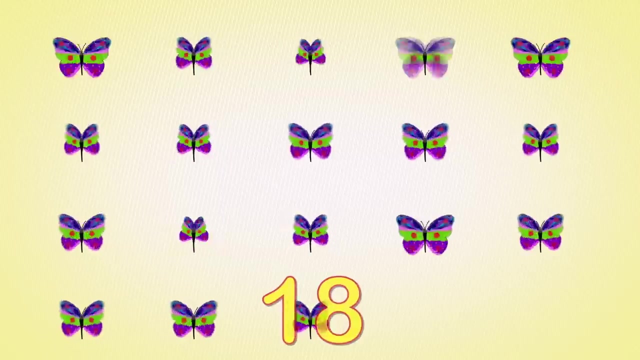 Beautiful butterflies, Hello. 1,, 2,, 3,, 4,, 5,, 6,, 7,, 8,, 9,, 10,, 11,, 12,, 13,, 14,, 15,, 16,, 17,, 18,, 19,, 20. 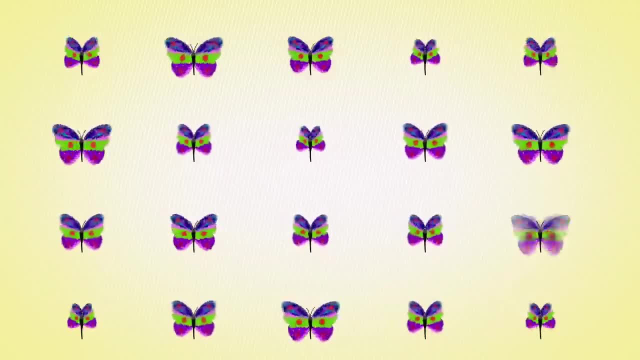 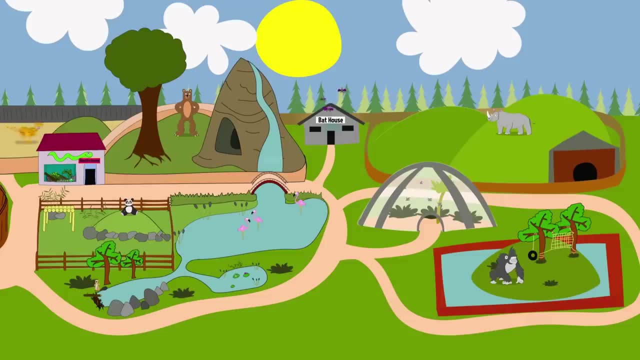 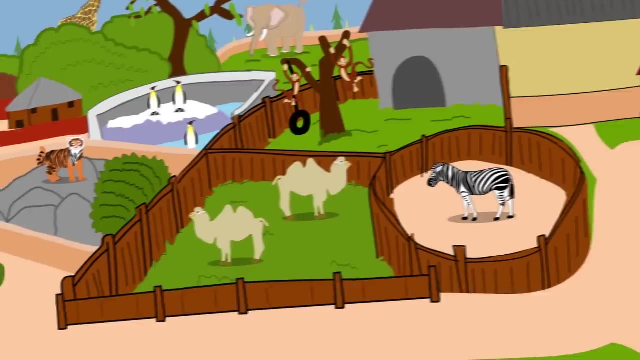 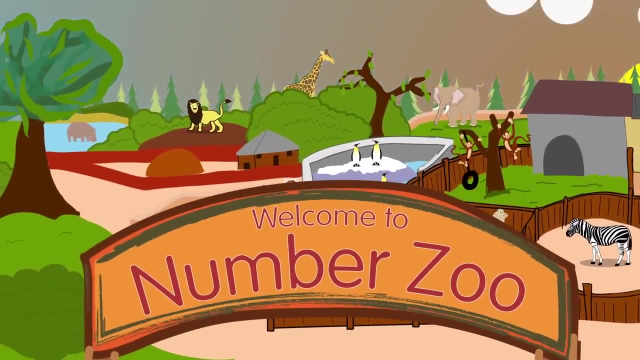 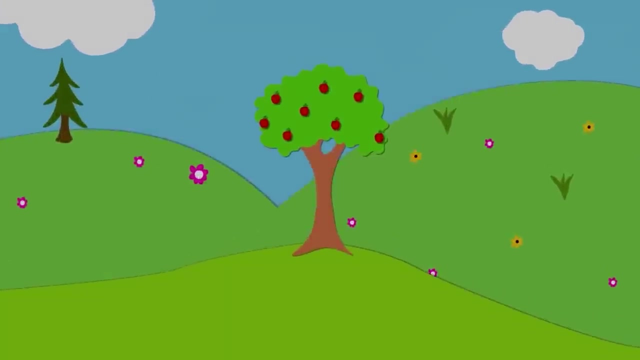 19,, 20, 20 butterflies. We've had such fun visiting the new animals. Thank you for joining us. We hope you enjoyed counting to 20.. You've done really well. Goodbye animals. We'll see you again soon. A for apple. 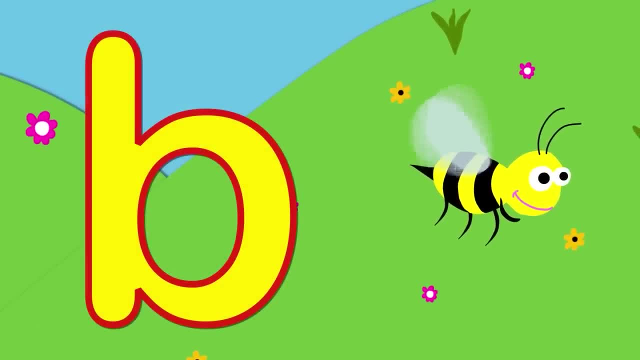 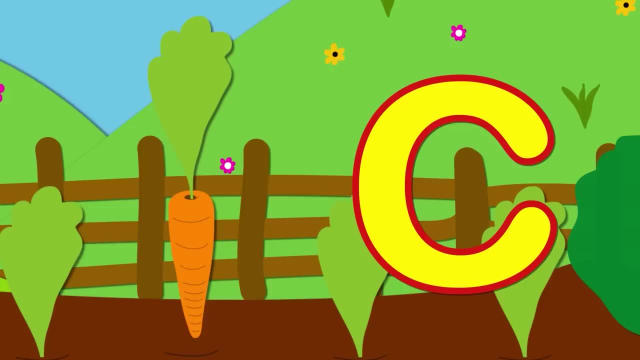 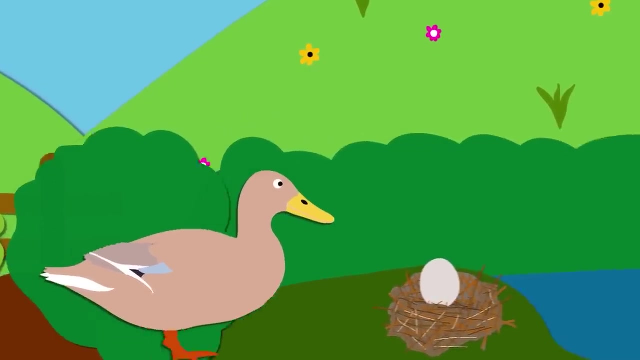 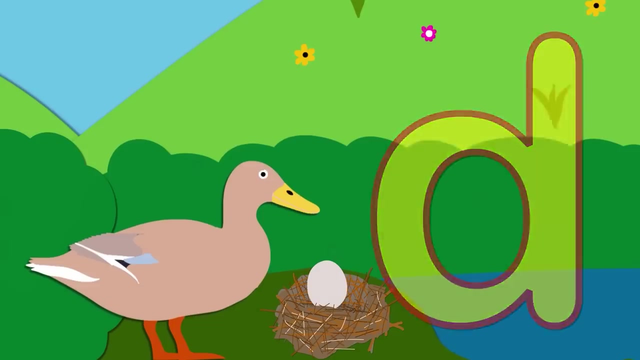 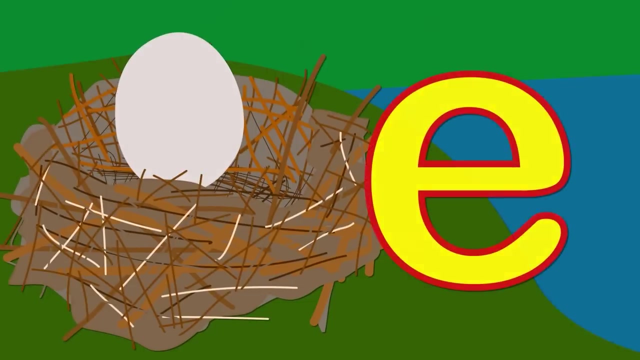 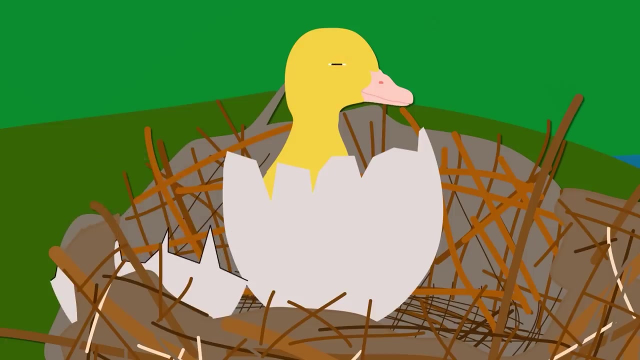 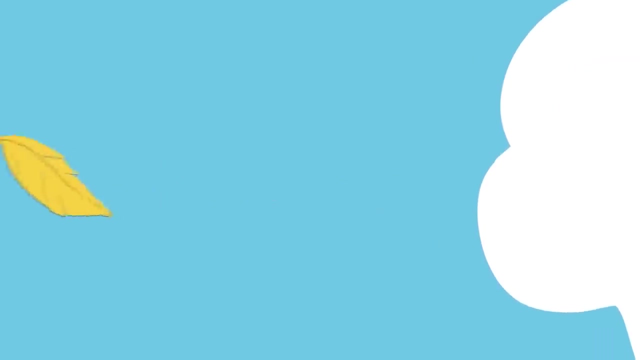 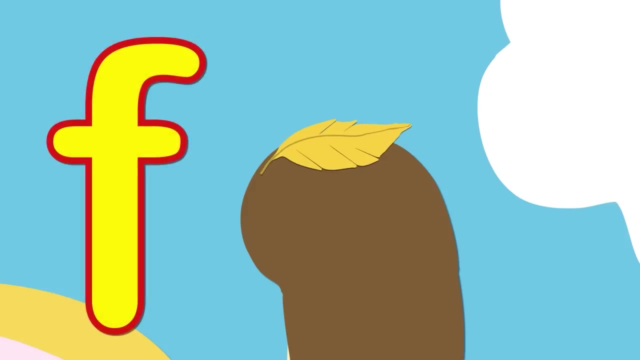 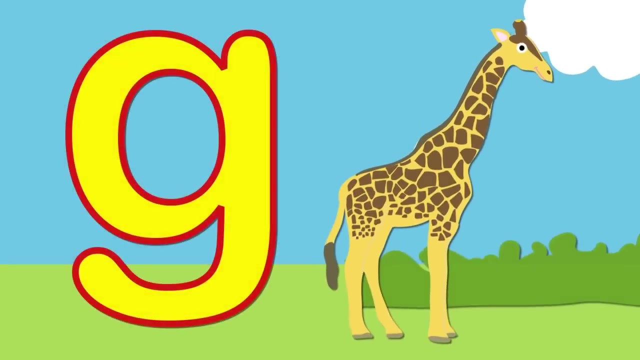 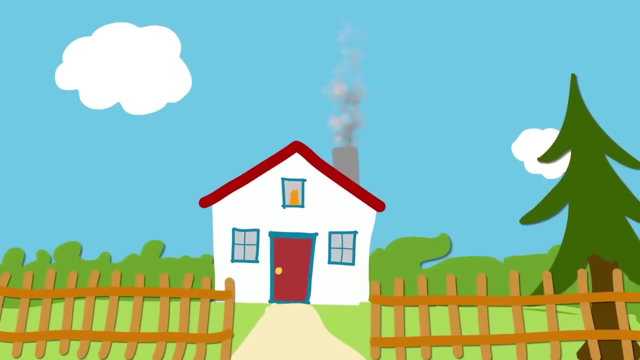 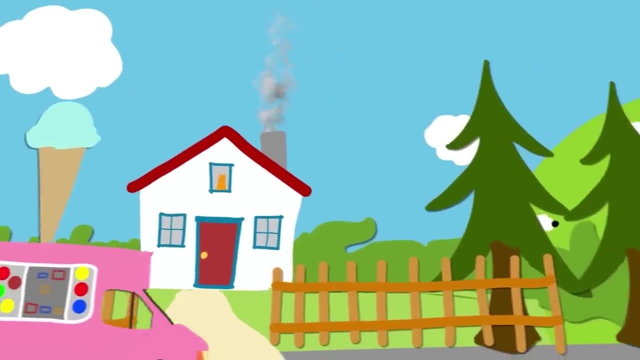 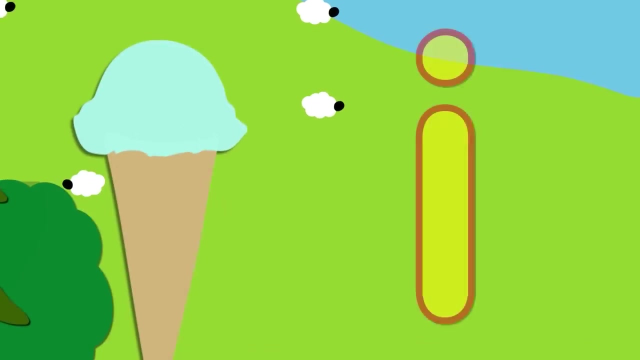 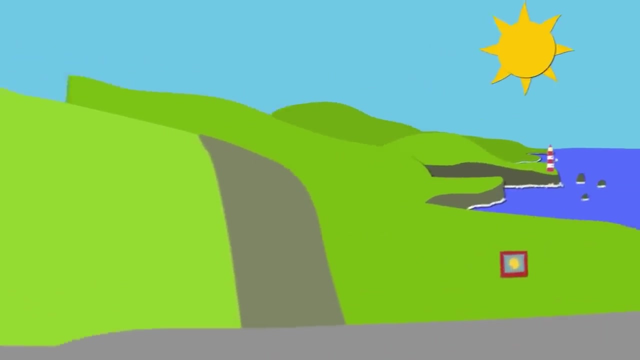 B for bumblebee, C for carrot, D for duck, E for egg, F for feather, G for giraffe, H for house, I for ice cream, J for L, J for jack-in-the-box- Jack-in-the-box. 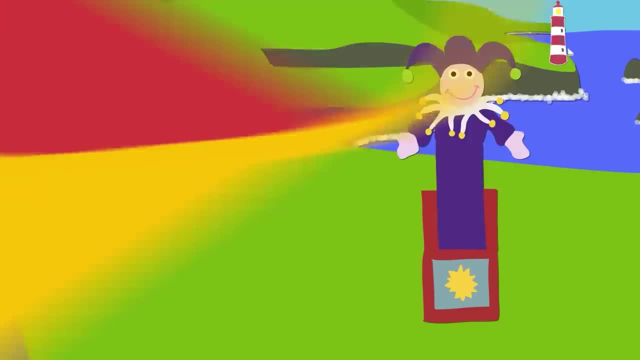 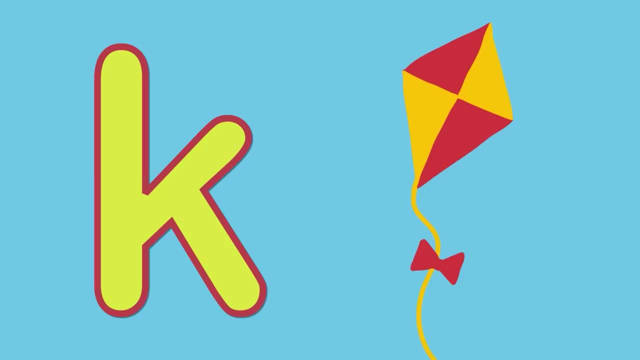 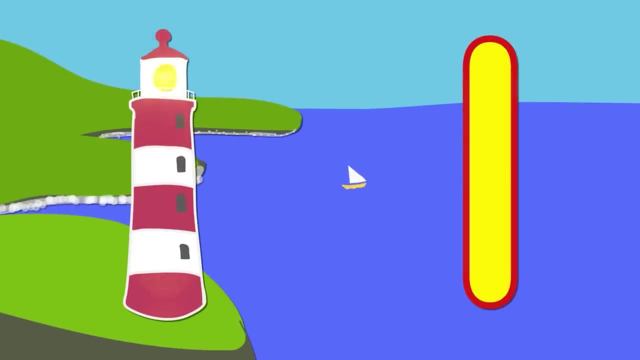 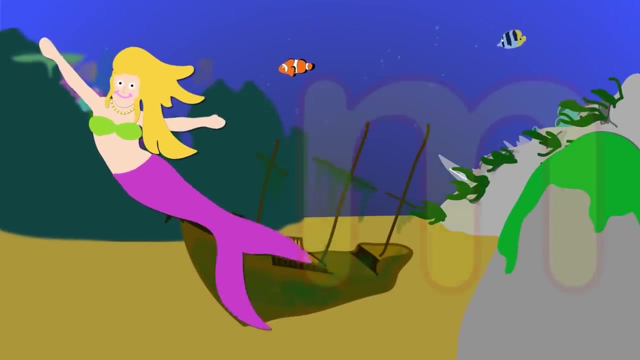 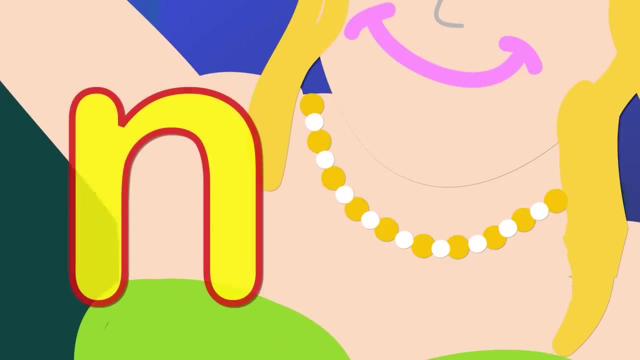 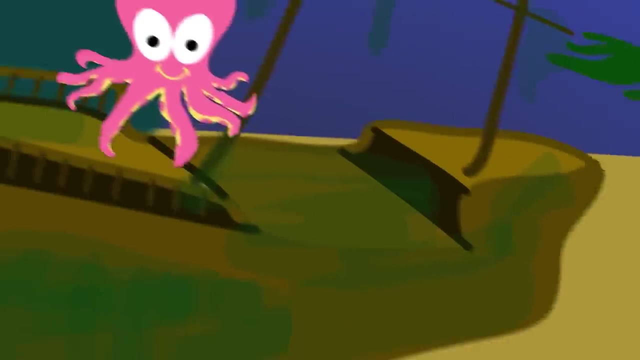 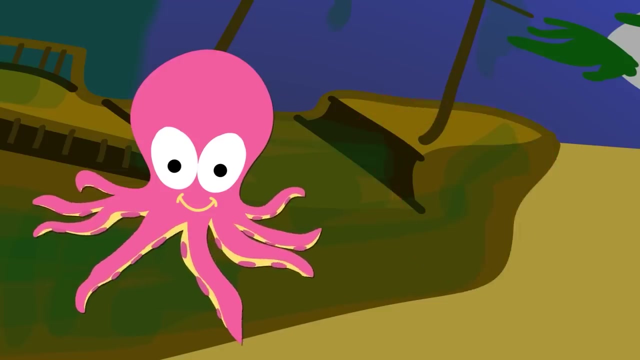 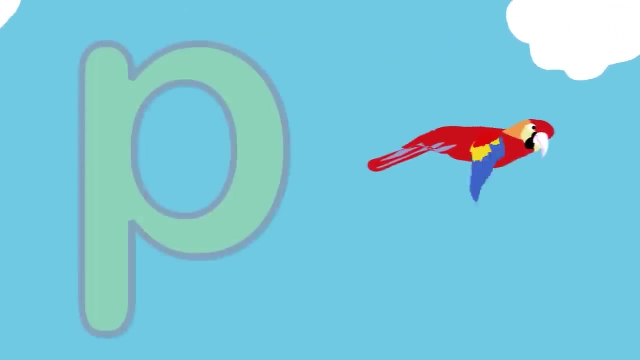 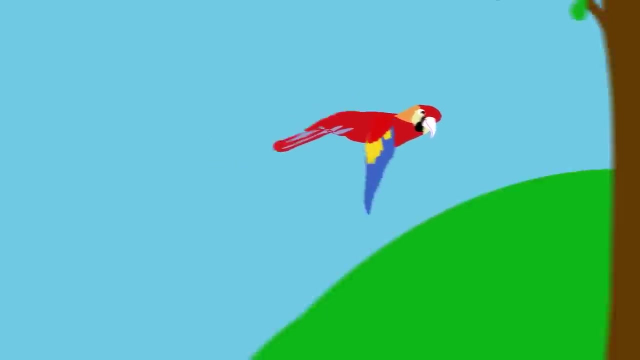 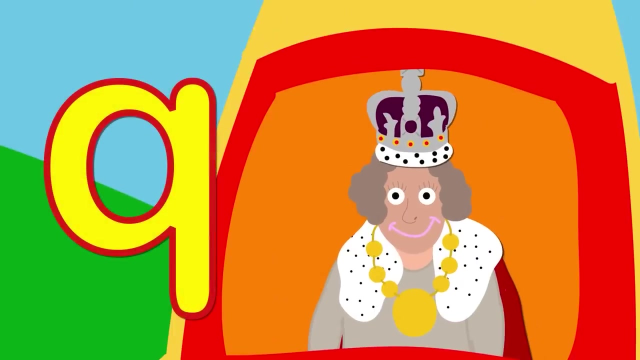 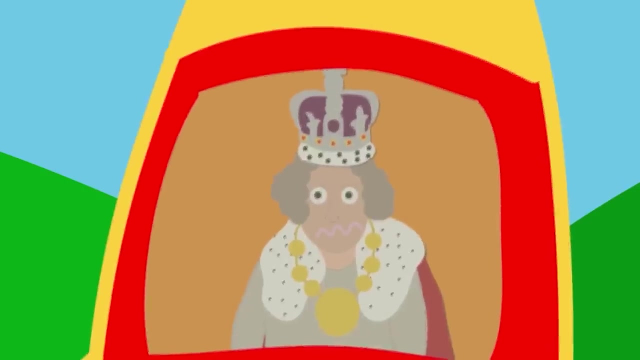 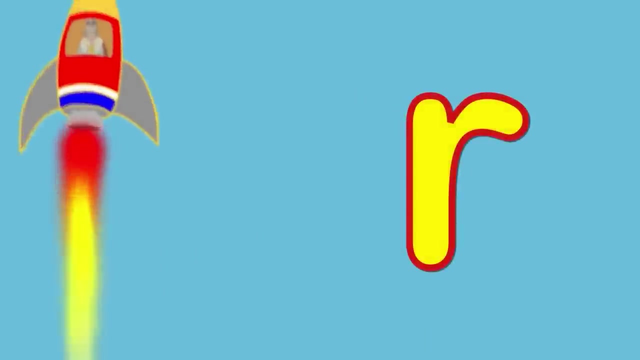 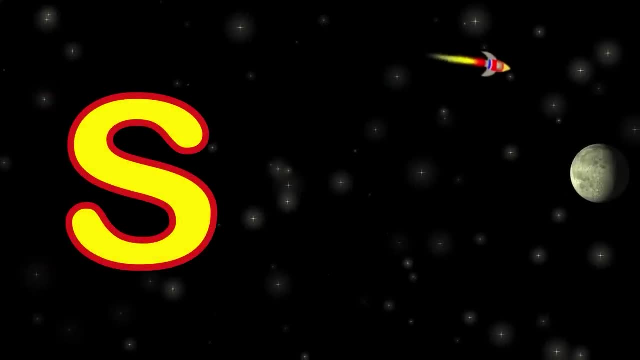 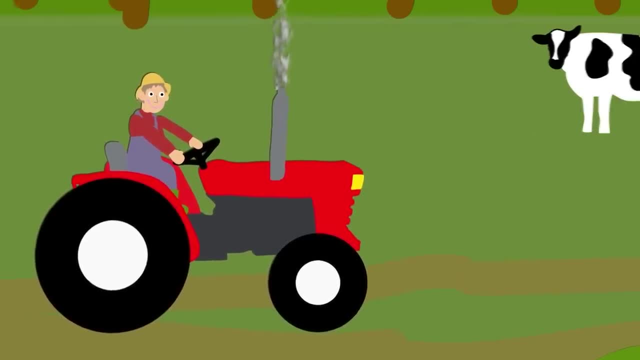 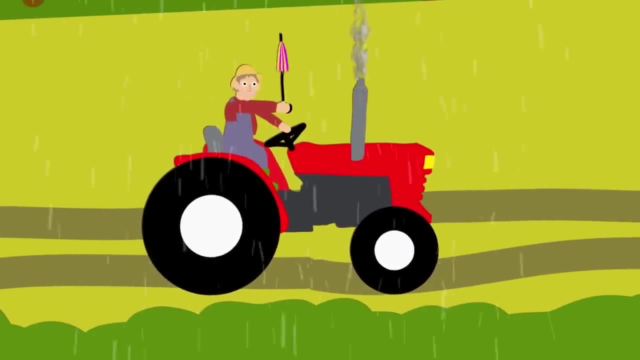 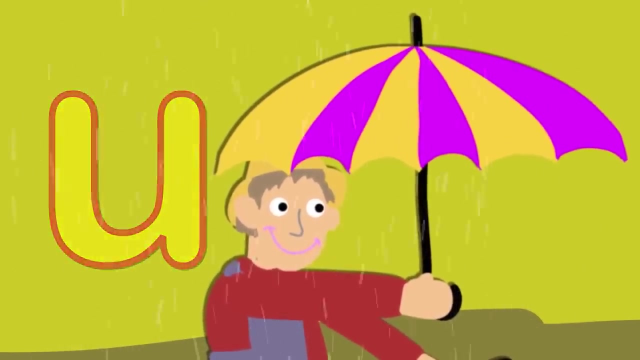 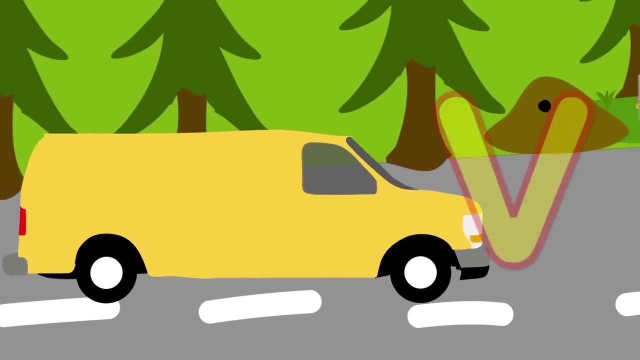 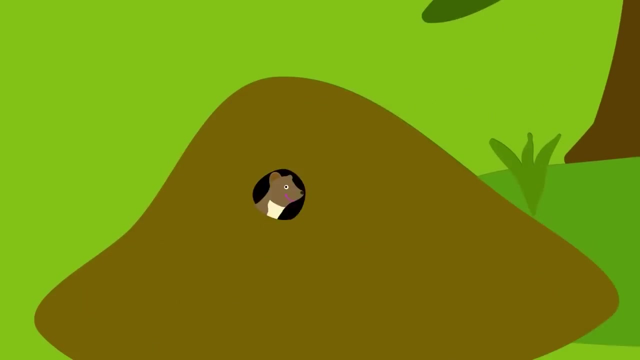 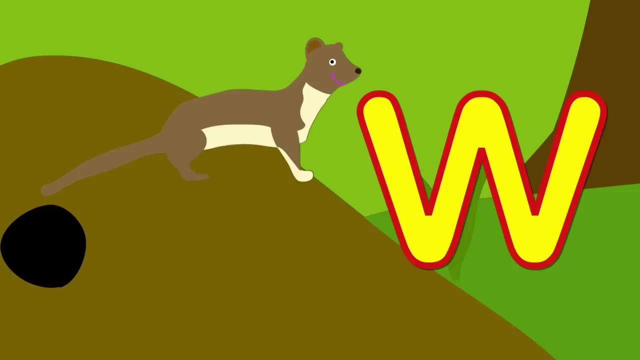 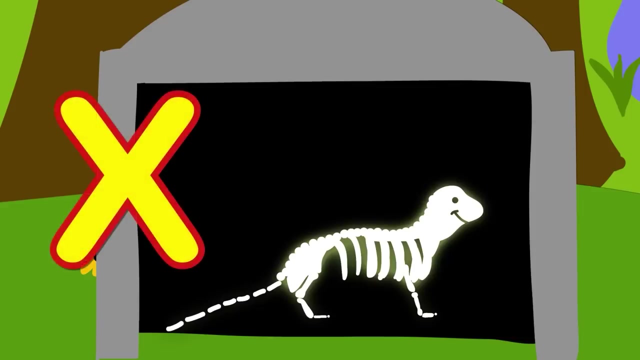 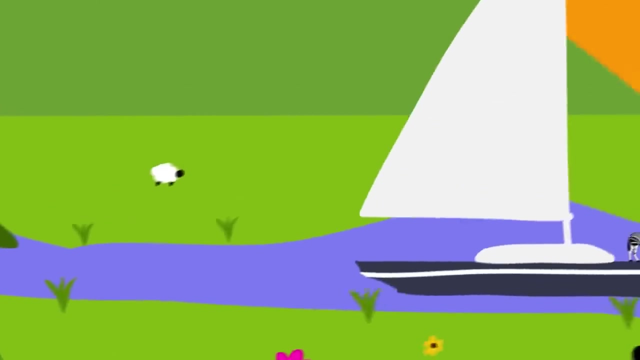 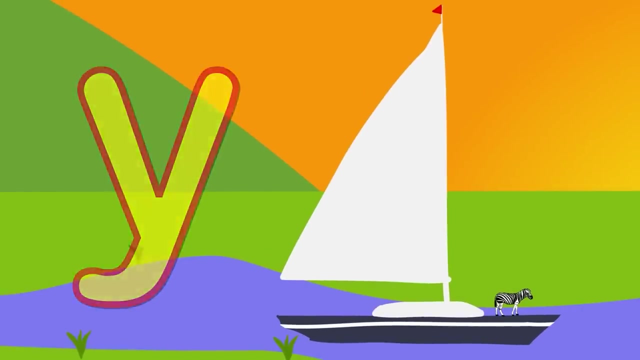 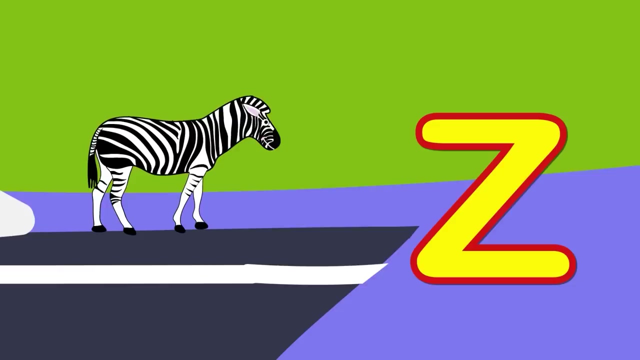 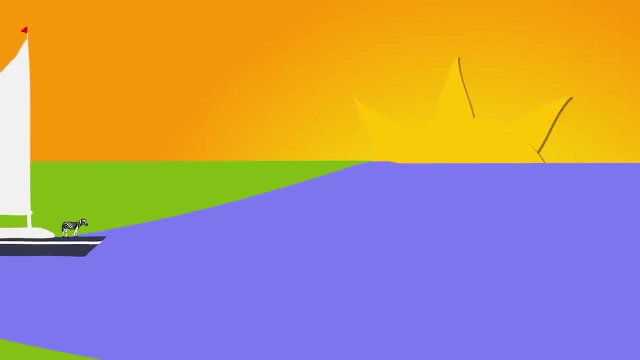 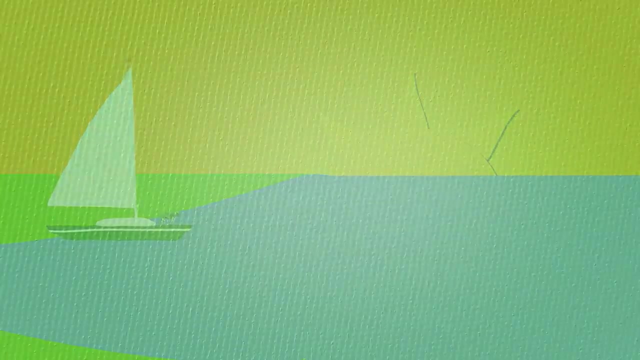 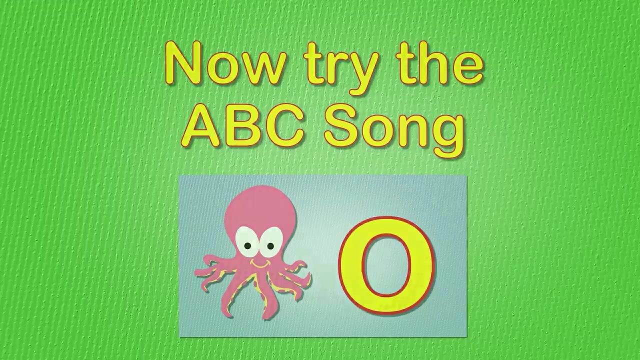 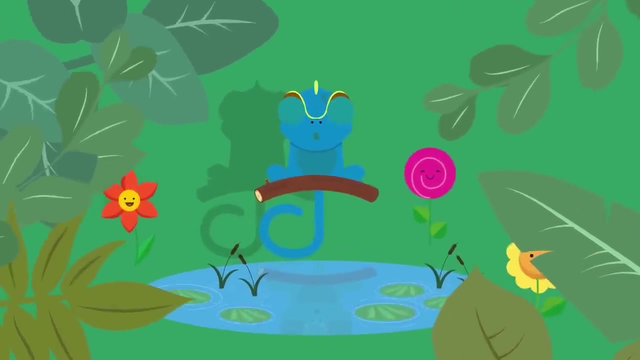 T for Tractor. U for Umbrella, V for Van, W for Weasel, X for X-Ray. Y for Yacht. Z for Zebra. X for X-Ray, X for X-Ray, X for X-Ray. Where's my chameleon? Where's my chameleon? 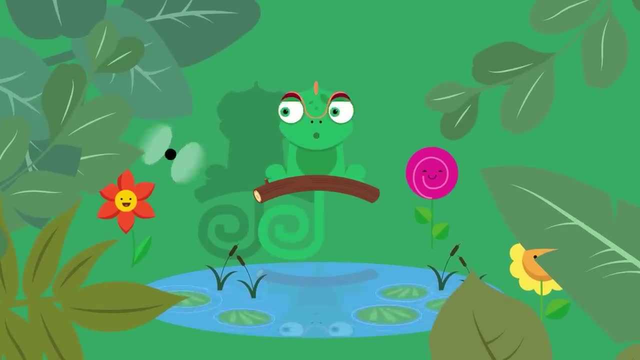 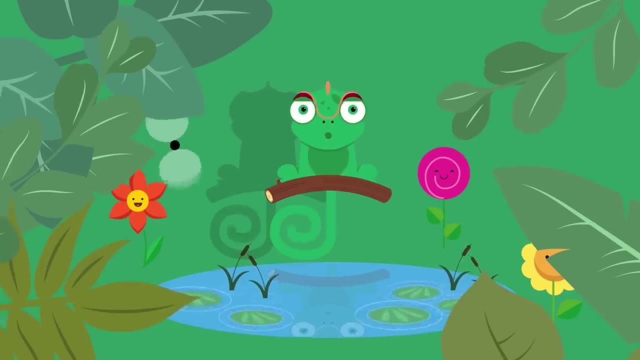 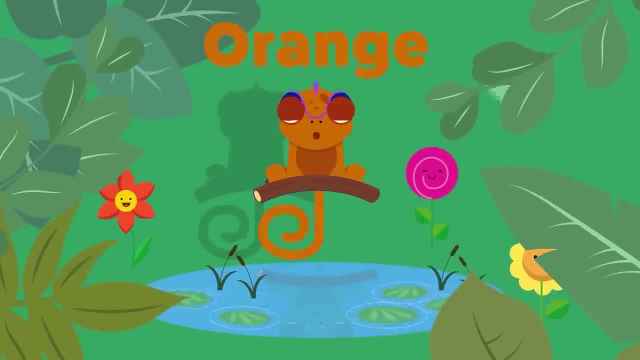 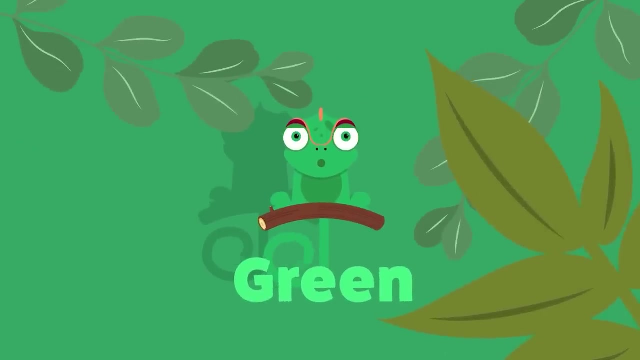 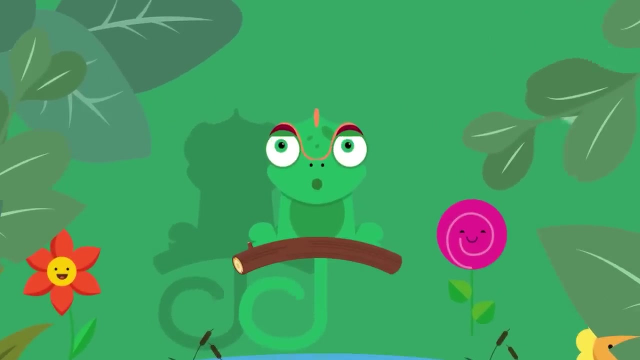 Anyone know? She was sitting right here just a second ago. No, no, she's not orange, nor yellow, nor green. She's not green. I said Unless- Hey, it is you. Your skin just changed colour from green back to blue. 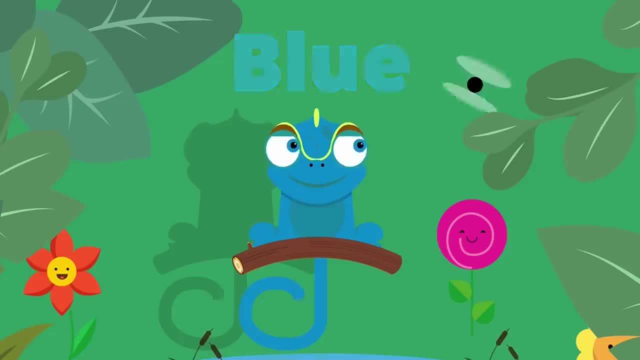 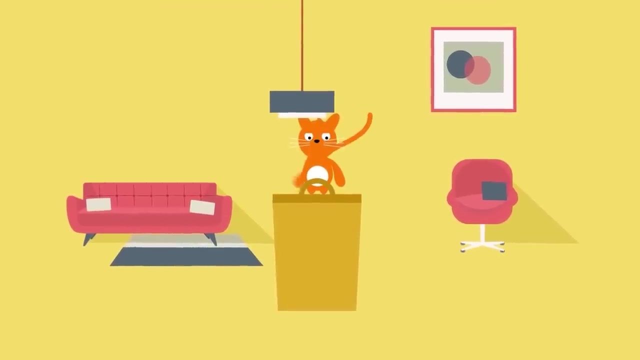 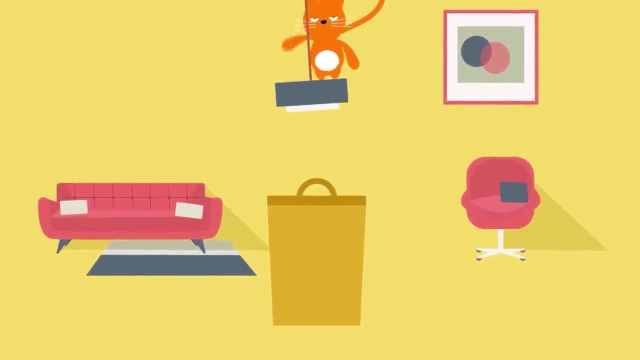 What a clever colour changing chameleon you are. Were you hiding all along? That's one great way to catch something crunchy for lunch. Where is my playful orange cat Jumping on this, swinging on that? Ah, the dirty clothes basket. 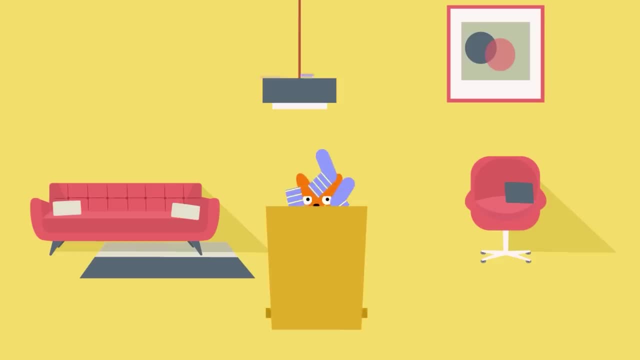 Yes, this'll be you. Wait, you're not my cat, She's orange. you're blue, Now you look green. How's that? Now you're red. Unless, Wait, is that just a sock on your head? Funny, crazy orange cat. 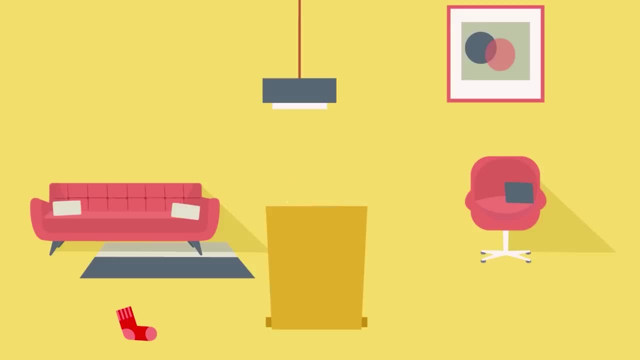 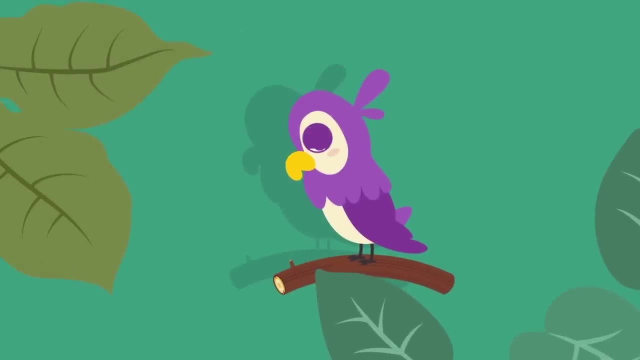 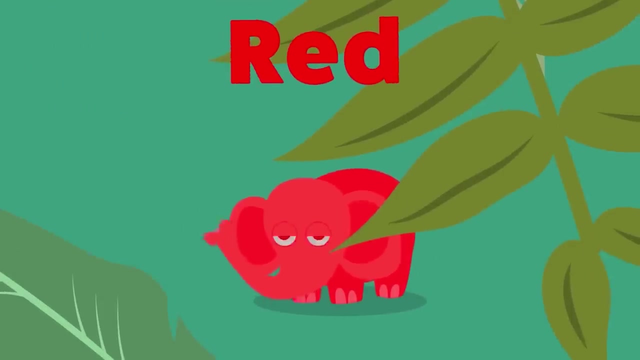 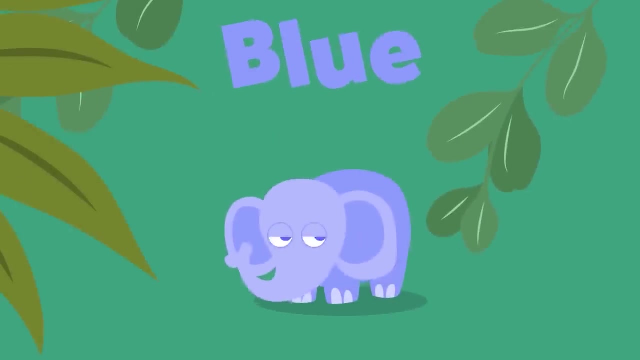 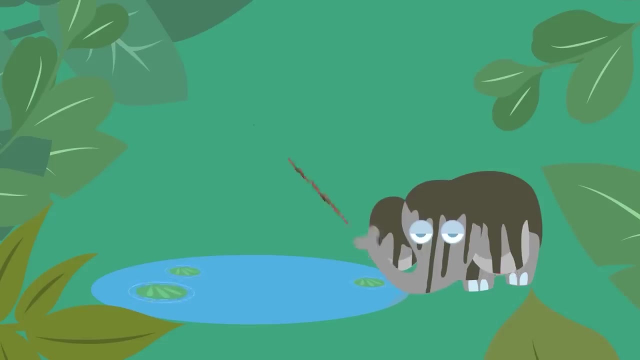 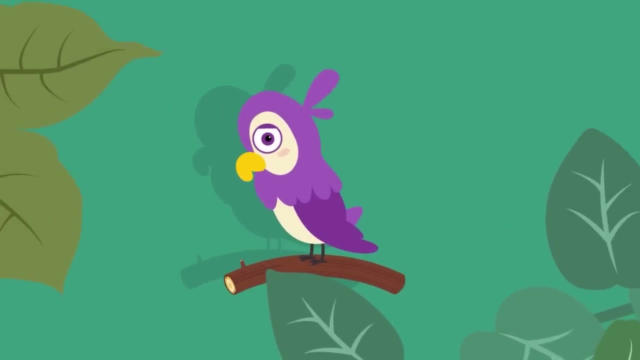 It was you all along, under all those smelly socks, I can't find my elephant. What shall I do? Ahhhh, What is this? my Ellie's? not red, not pink, not blue, nor is he mud brown. he's decidedly gray. Oh, Ellie, where are 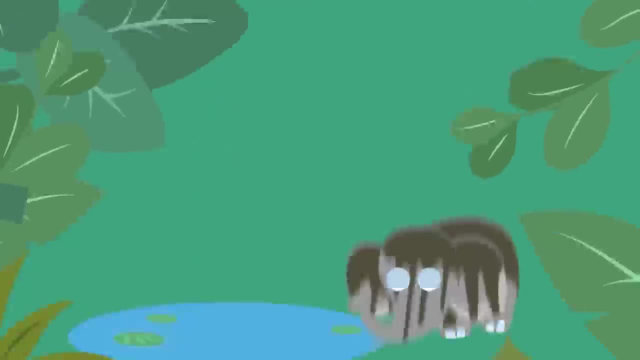 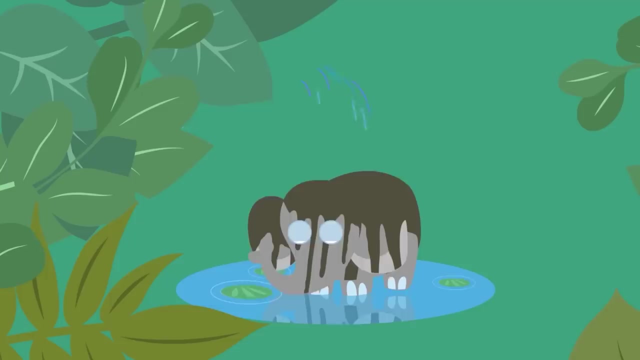 you. you've been gone all day unless- no, it can't be I have to be wrong. but look, there's the gray. it was you all along. I can't believe what's going on here. Ellie's not red, not blue, nor is he mud brown. he's decidedly gray. 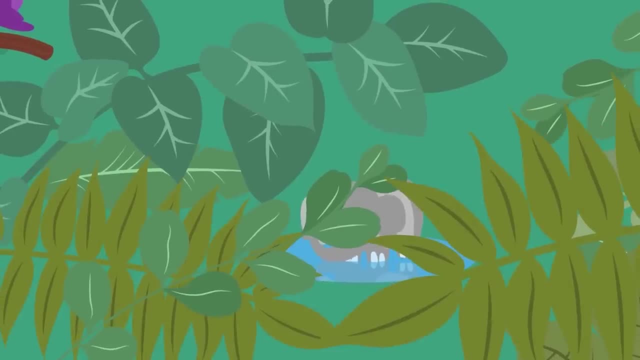 what's going on here? Ellie's not red, not pink, nor is he mud brown- he's decidedly gray. what's going on here? Ellie's not red, not blue, nor is he mud brown- he's decidedly gray. that's a muddy mess. you are, Ellie. good job, you're having a bath. the pups are going to. 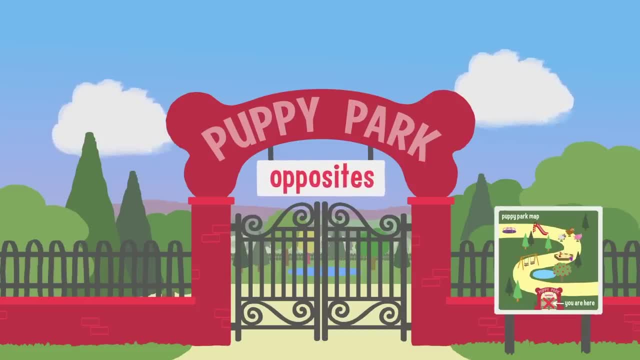 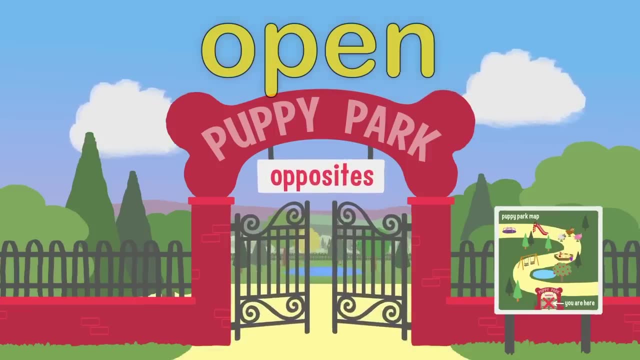 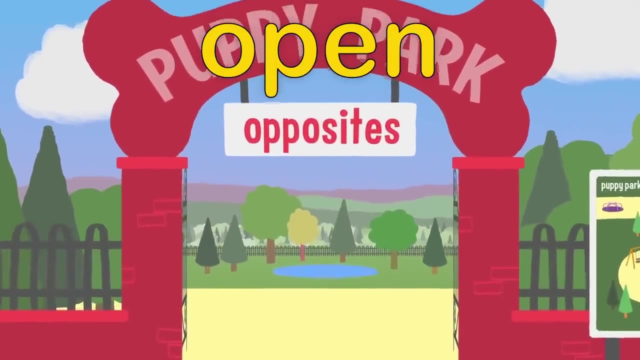 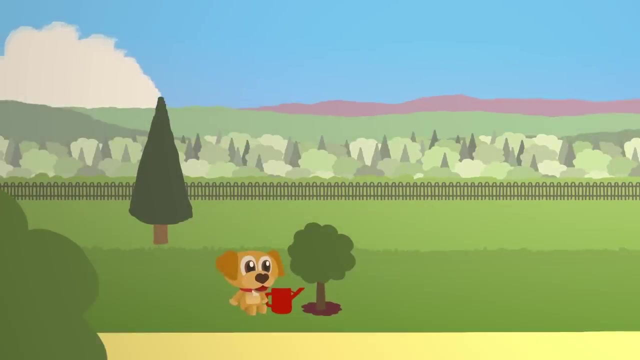 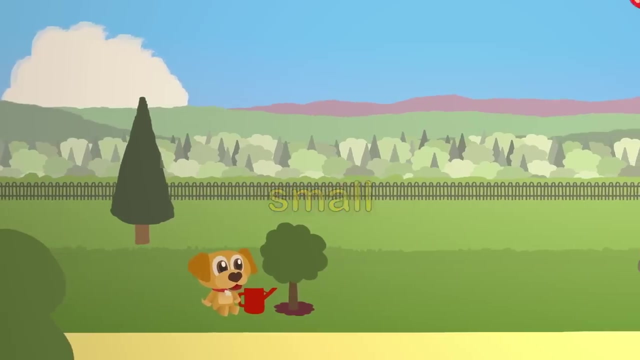 show us some opposites. today. it's very early in the morning and the gates to the park are closed. here we go now the gates are open. come on, pups, let's head into the park and have some fun. you, Henry, has just planted a new tree and he is watering his small tree to help it grow. 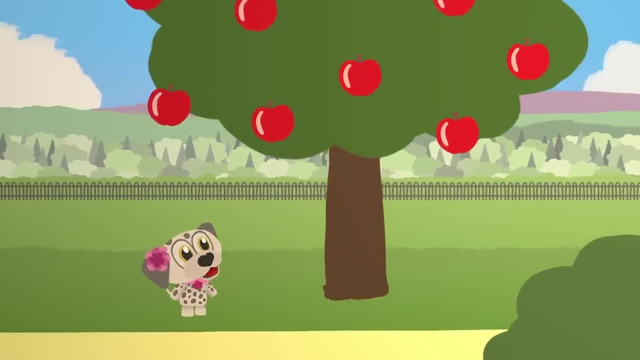 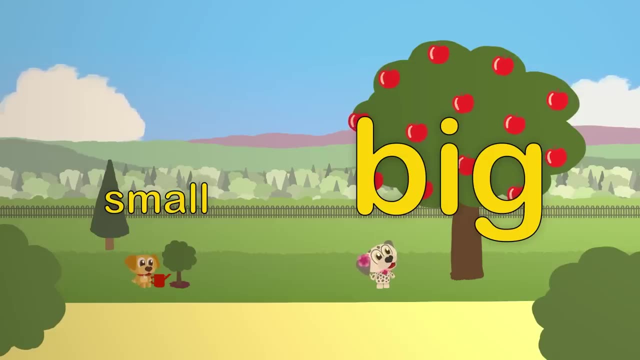 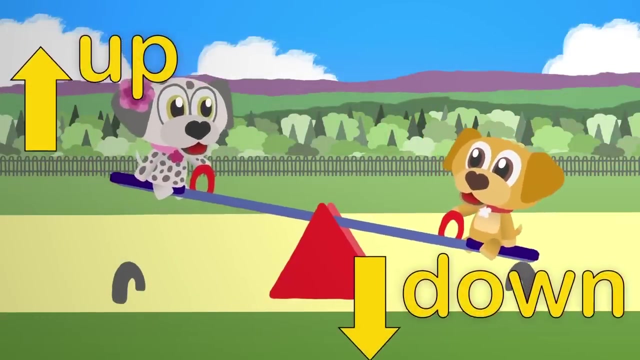 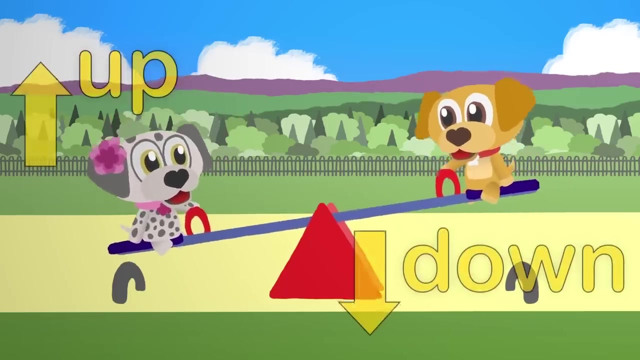 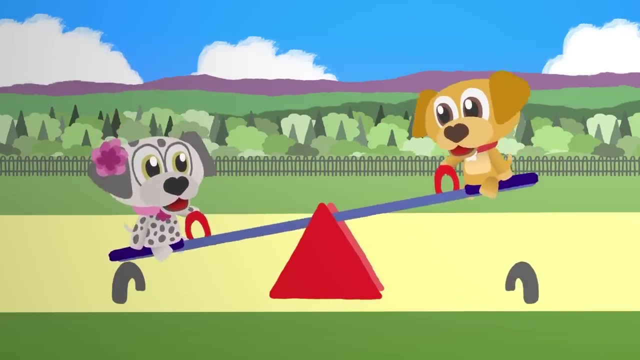 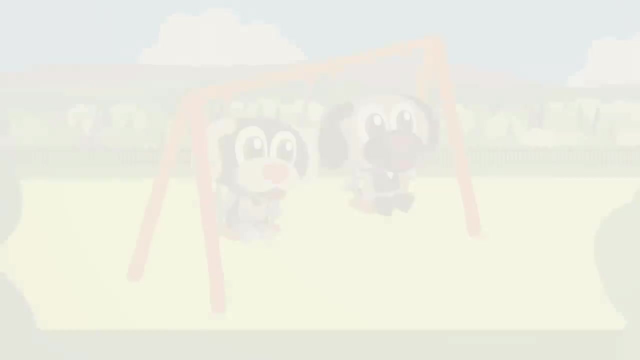 Dottie is looking at her big tree which has lots of juicy apples on it. Small and big, they are opposites. The pups are playing on the seesaw. The seesaw goes up and down, up and down, up down. opposite. 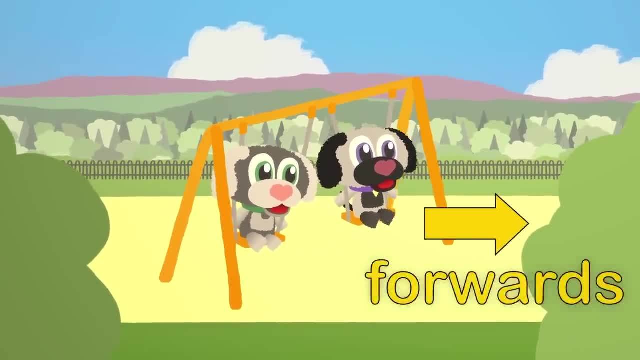 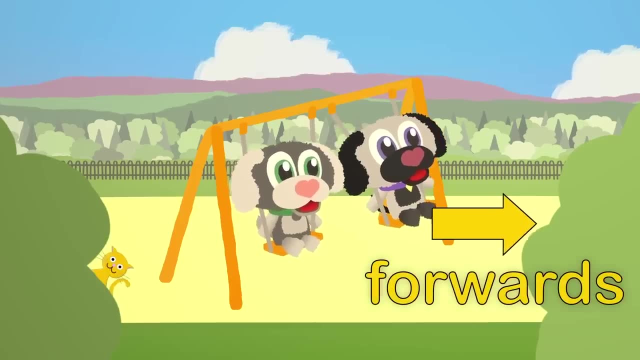 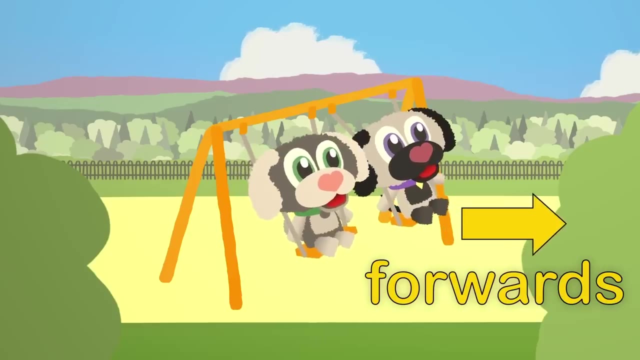 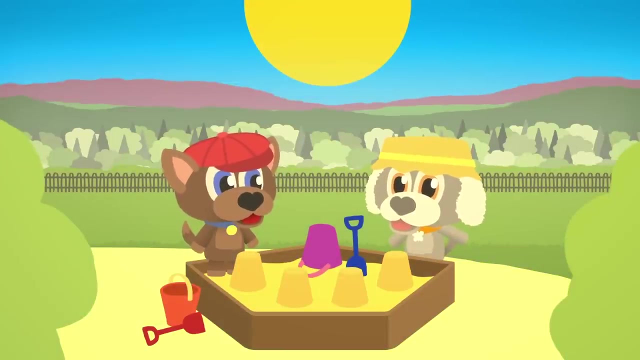 Ollie and Thomas are swinging high on the swings. They are swinging forwards, They are swinging forwards, They are swinging forwards and backwards, forwards, backwards. They are opposites. Freddy and Bertie are building sandcastles and the weather is hot. 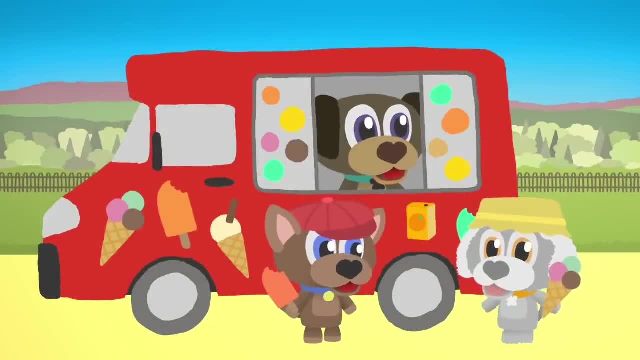 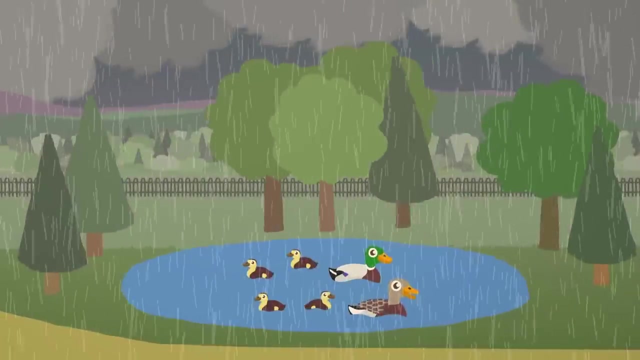 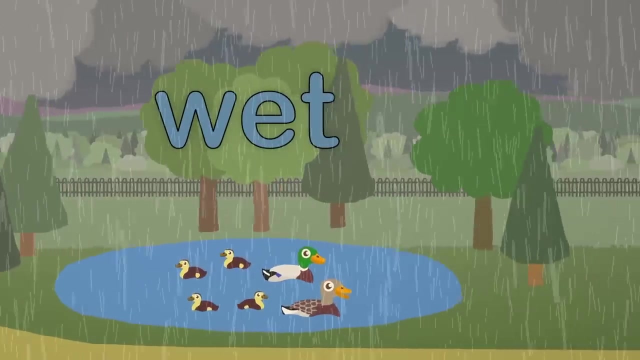 They need to cool down by eating a cold ice cream. That's another opposite: hot and cold. Can you think of something that's hot And then something that's cold? The ducks are swimming in the pond and are getting very wet. Luckily, Dottie has her umbrella, which is keeping her dry. 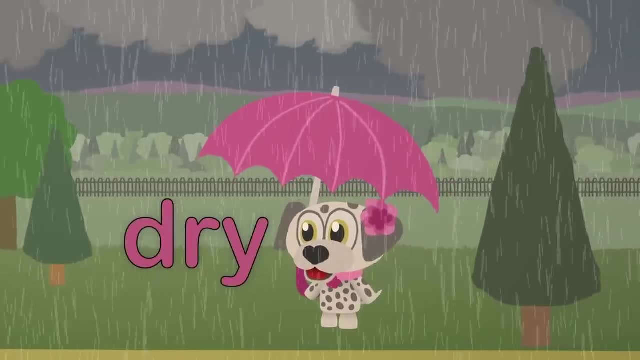 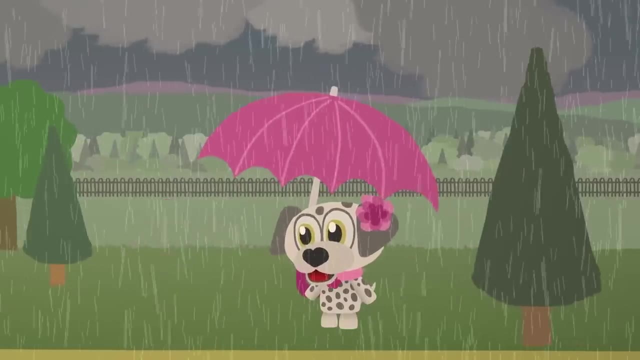 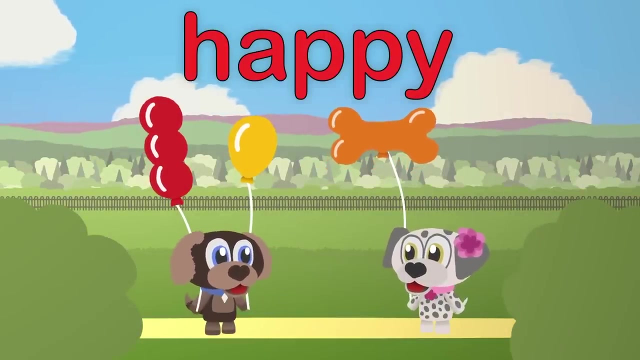 I can have some ice cream. I can have some ice cream. I like ice cream, I love ice cream. That's another opposite: Hot and cold, wet and dry. the pups are both happy. but oh no, Dottie has let go of her balloon, so 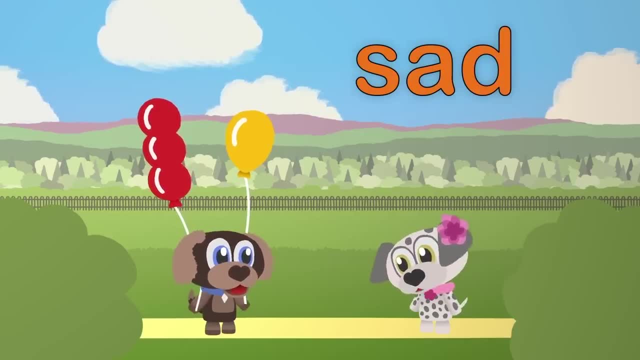 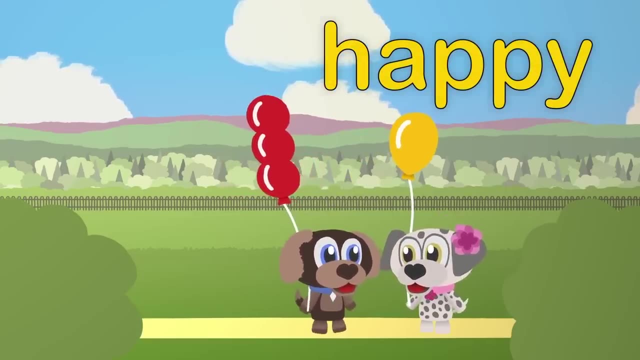 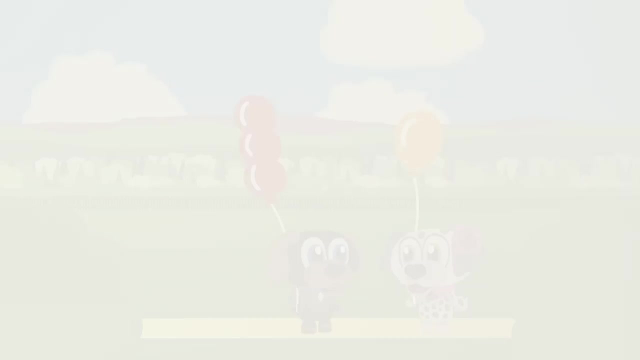 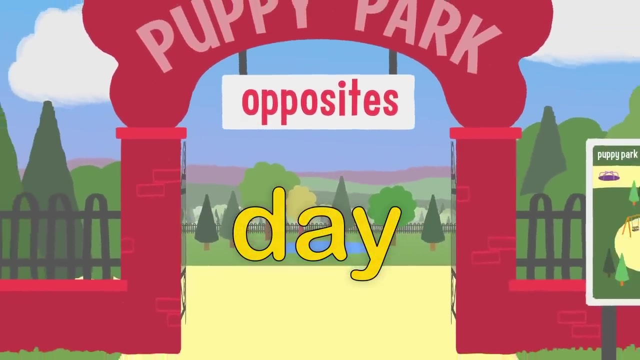 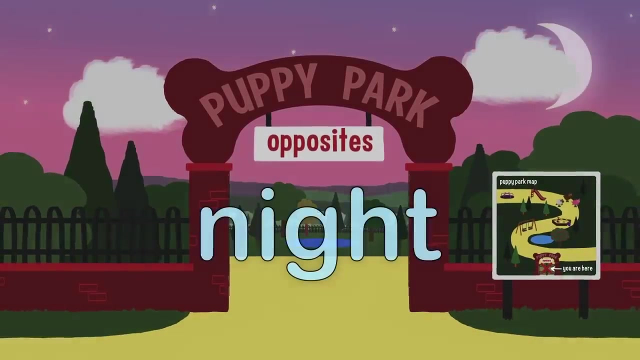 now she is sad. Milo is very kind. he gives one of his balloons to Dottie, which makes her happy again. well done, Milo. happy is the opposite to sad. it's daytime in the park now, but now it's getting dark and it will soon be nighttime. day and night, they are opposites. 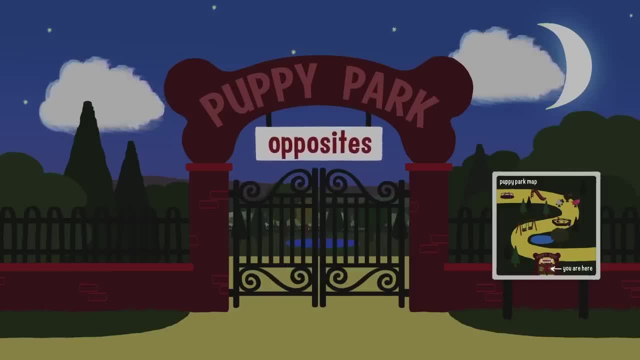 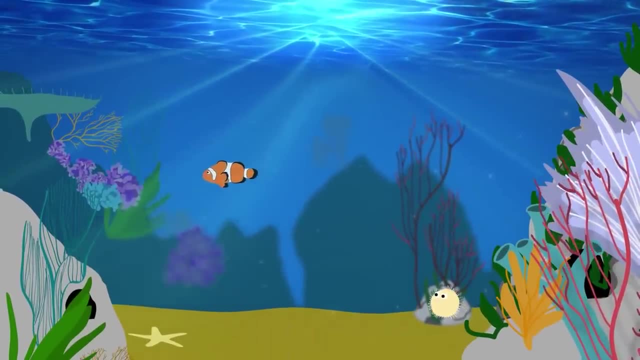 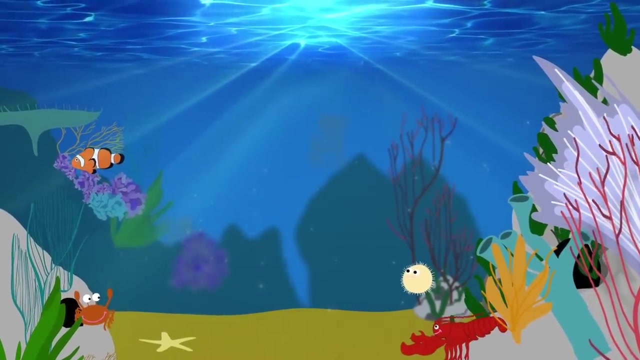 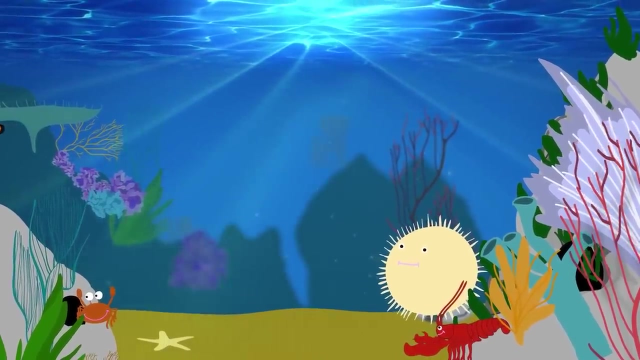 bye, bye, here we are under the sea. it is my favorite place to be: a watery world beneath the waves, where crabs and lobsters crawl from their caves. let's learn some shapes with our funny sea friends and we can discover how this fishy tale ends. 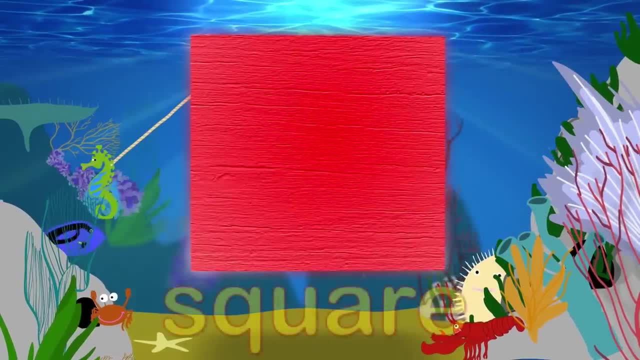 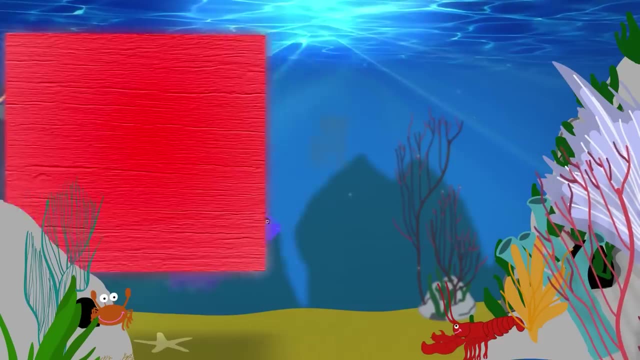 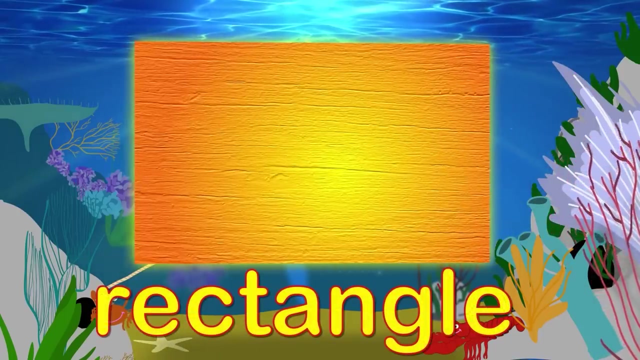 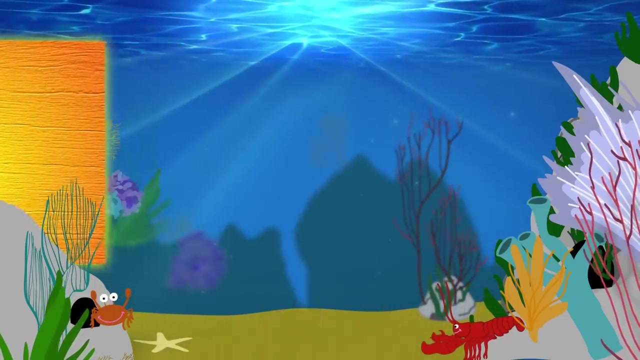 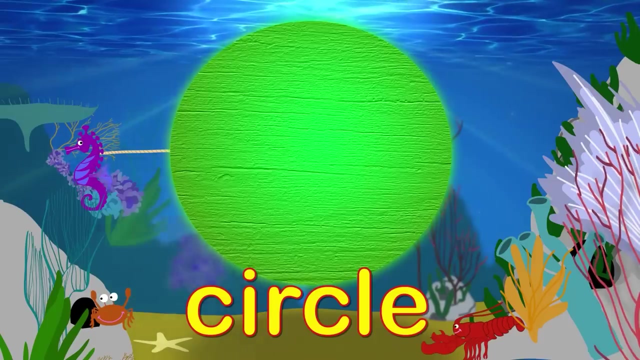 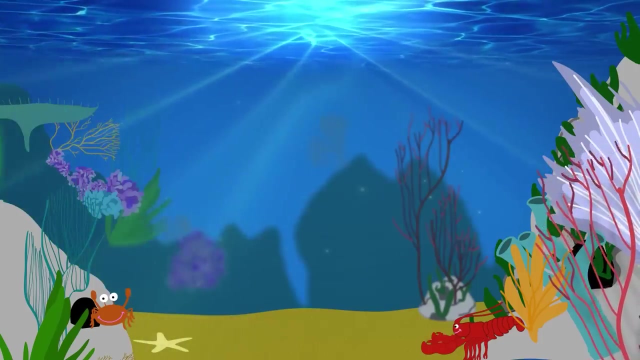 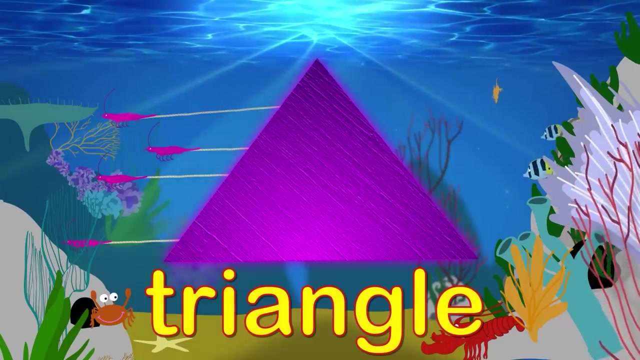 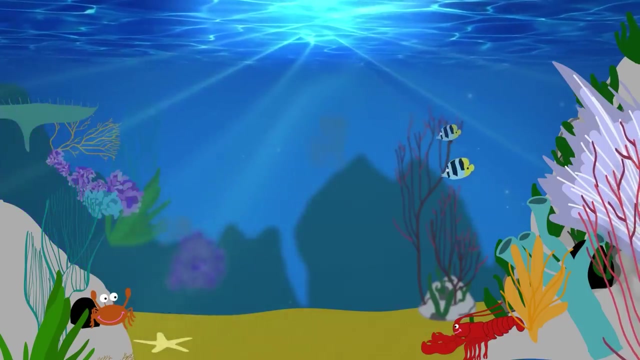 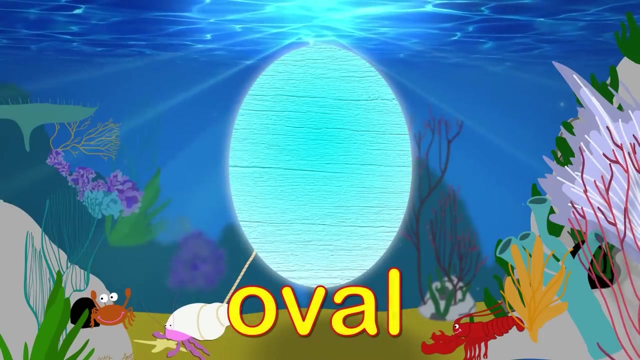 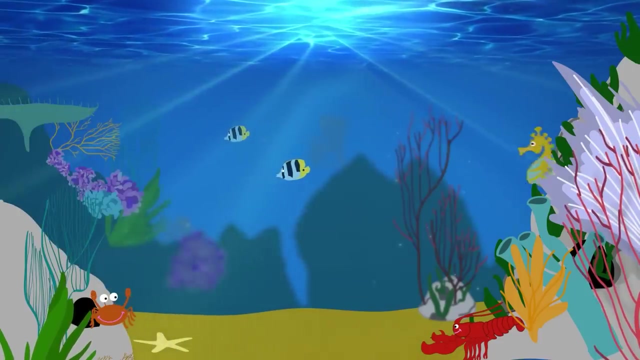 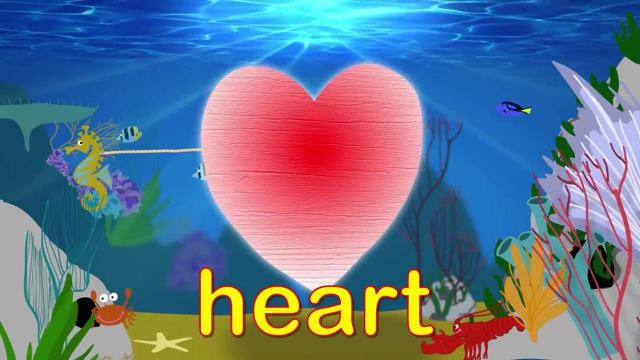 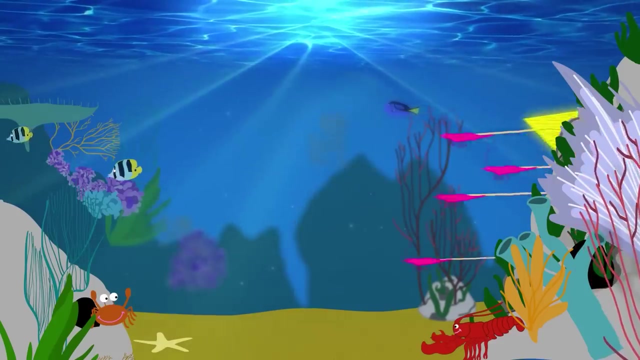 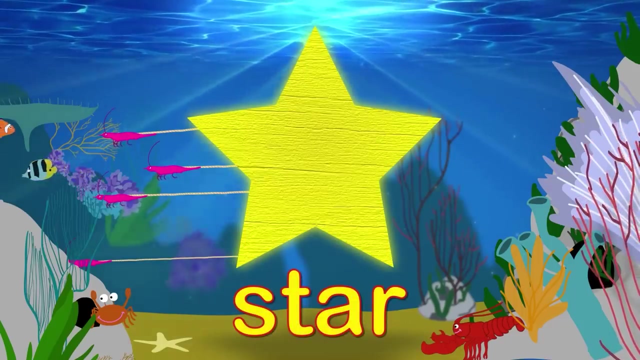 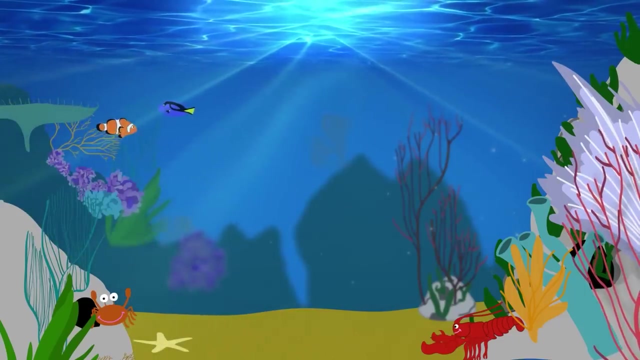 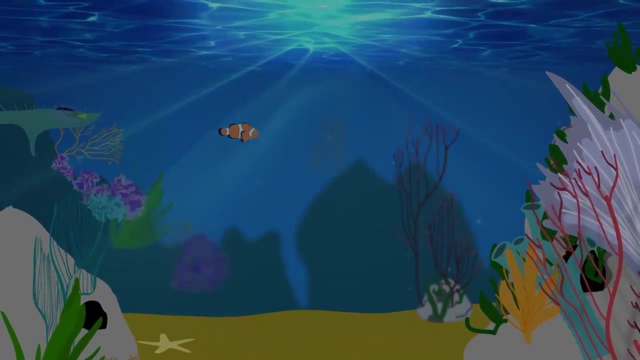 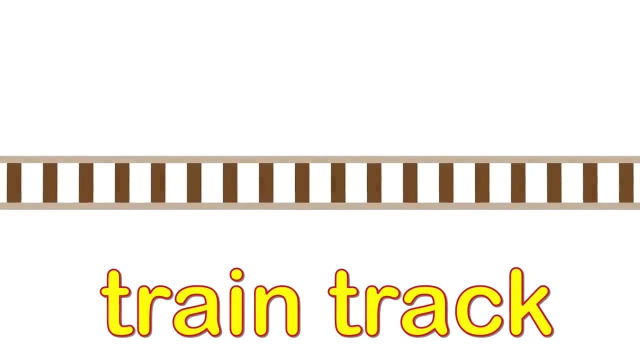 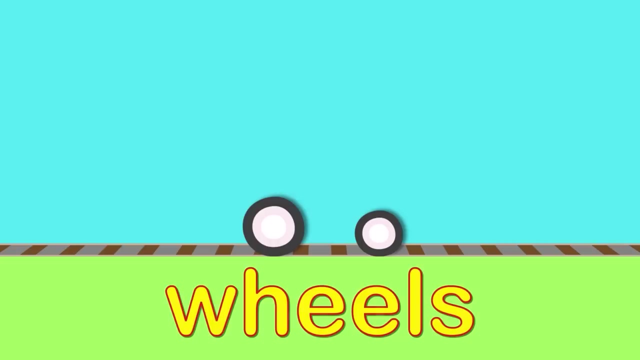 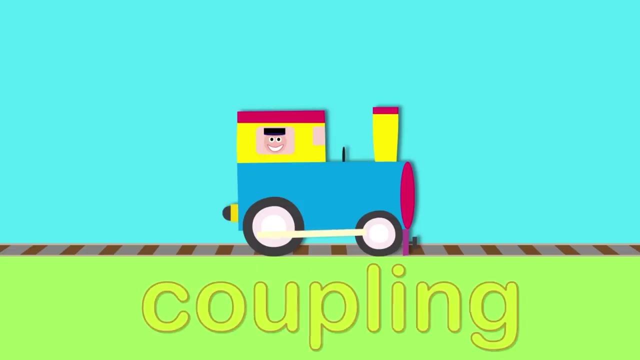 square rectangle. oh, oh, oh, circle, circle, triangle, oval, oval, circle, circle, carrion, circle, circle, circle, circle, heart, our water star star. Thank you, friendly sea creatures, see you again soon. Boiler Jiminy, Cabin Buffer Whistle Coupling Coal Truck.